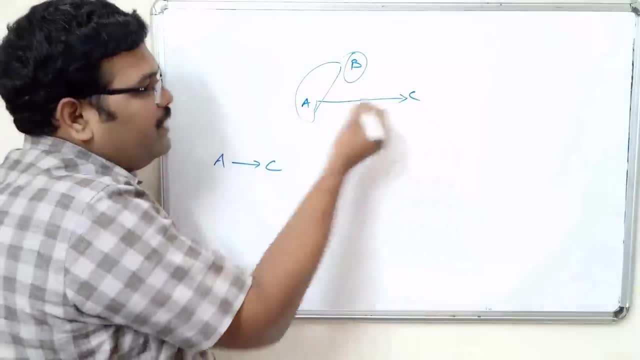 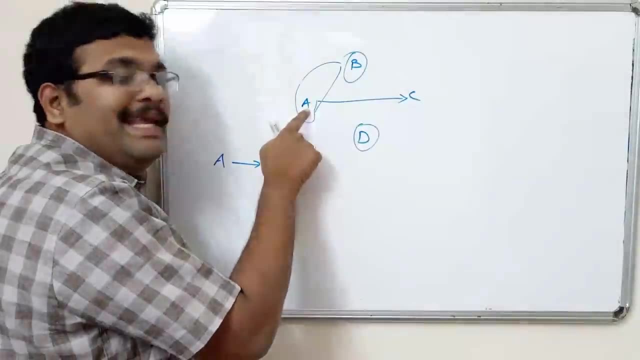 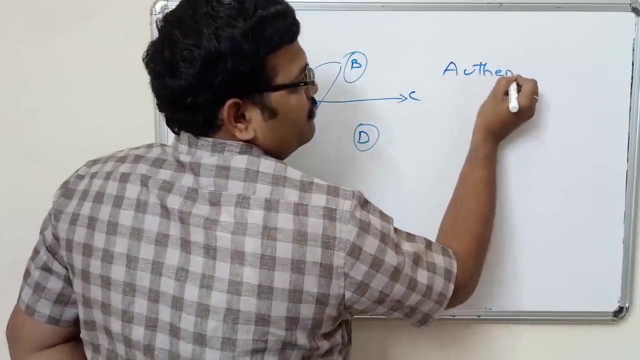 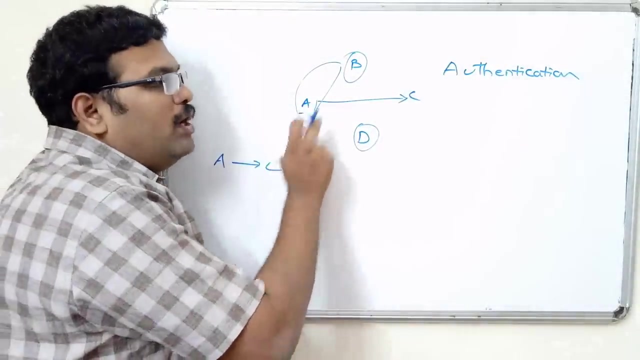 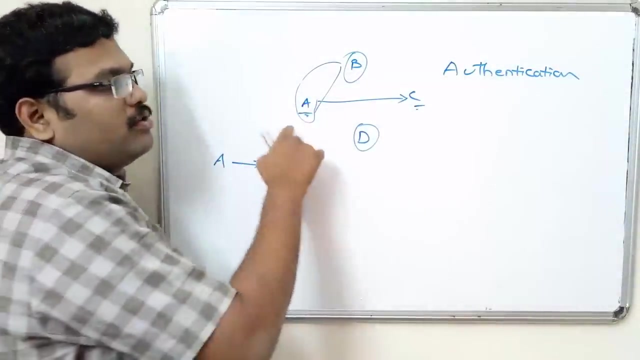 authorization, and here the authentication means verifying the user identity. so among these three users, C should receive the message only from A, so that identity is called authentication. so similarly, A should send the message only to C, so A should authenticated by C and C should be authenticated by A, so this is called authentication. so this is. 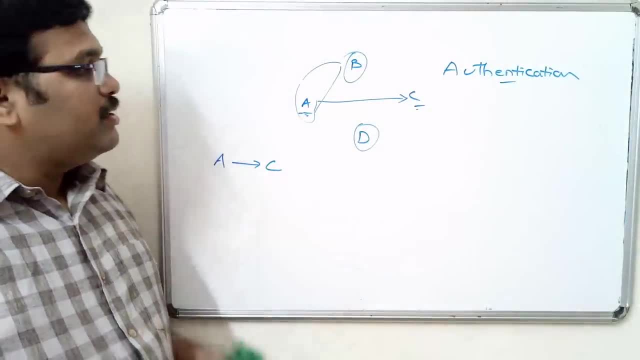 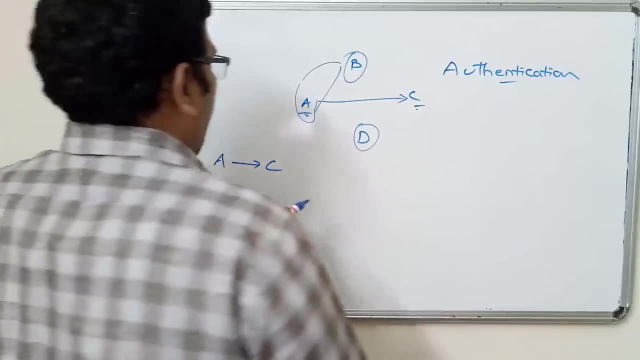 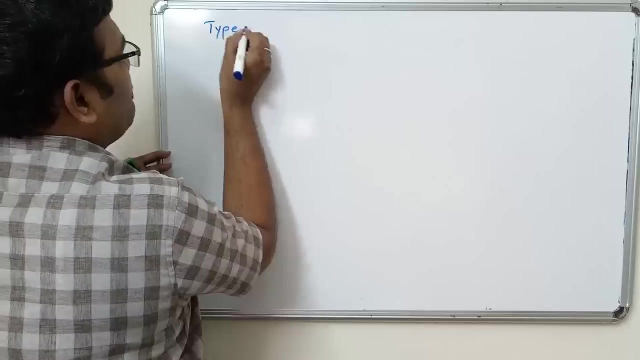 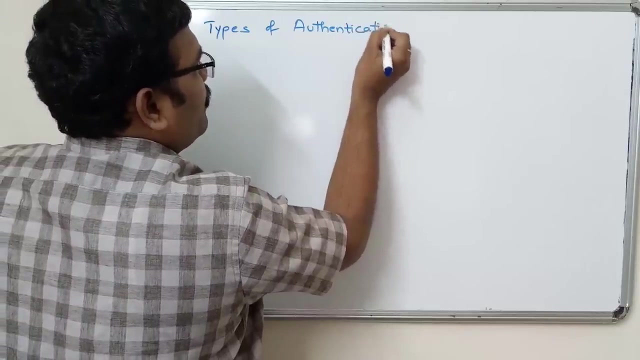 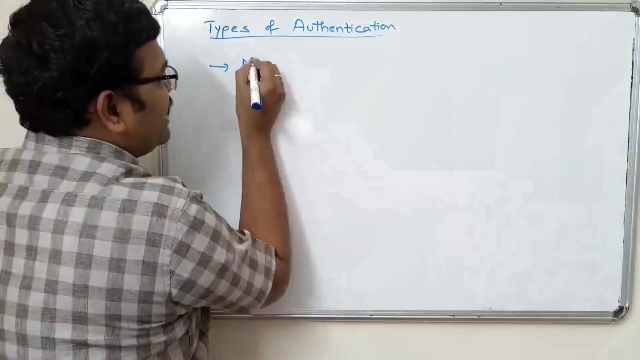 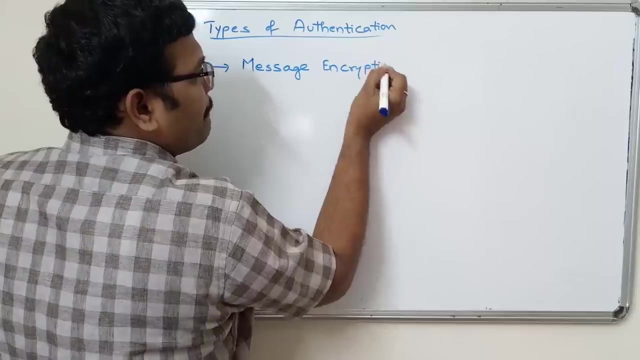 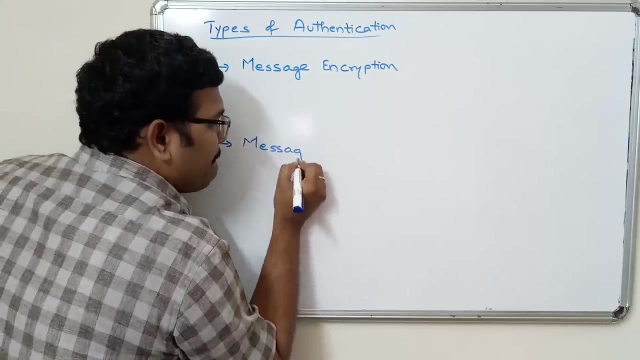 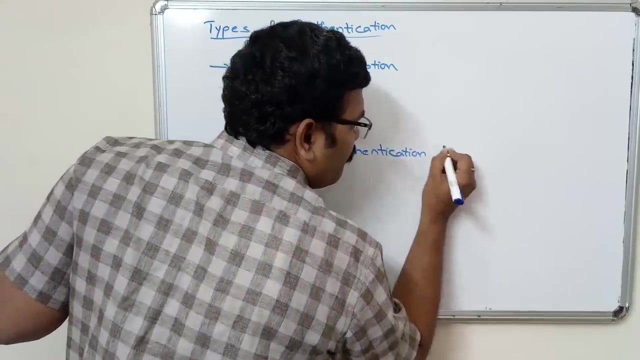 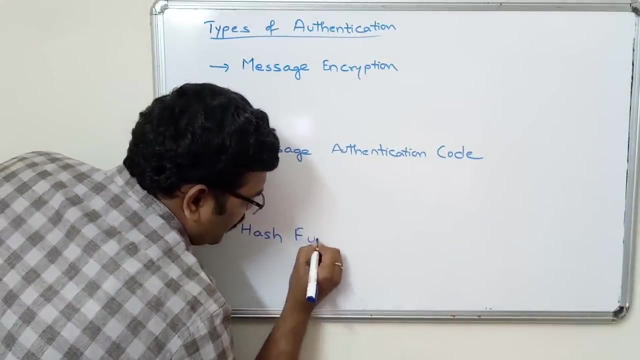 one more service of our security. so here, first let us see the different types of authentications. first, types of authentications. so there are mainly three types of authentications. first one is message encryption, next message authentication code, and the third one is hash functions. so, coming to this, 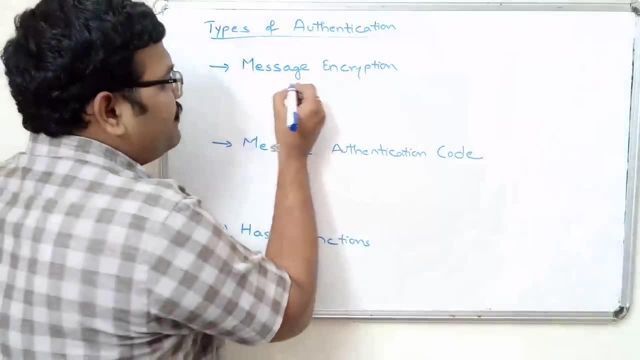 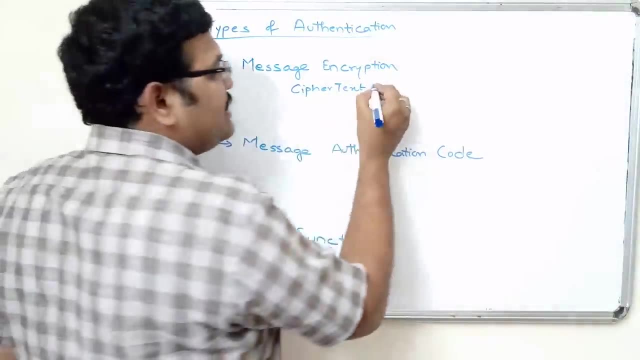 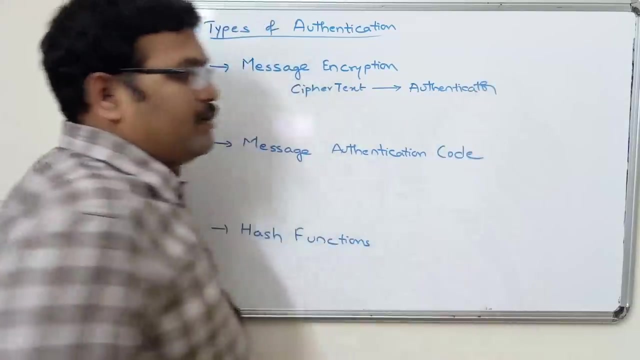 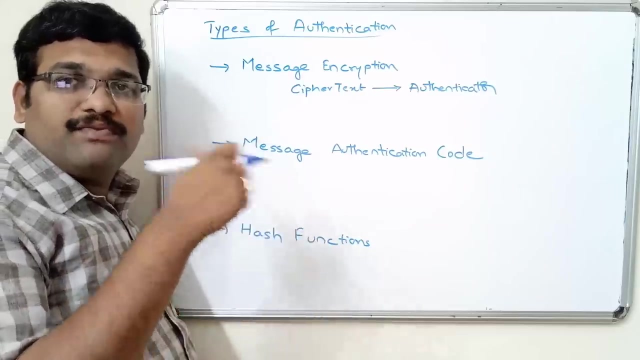 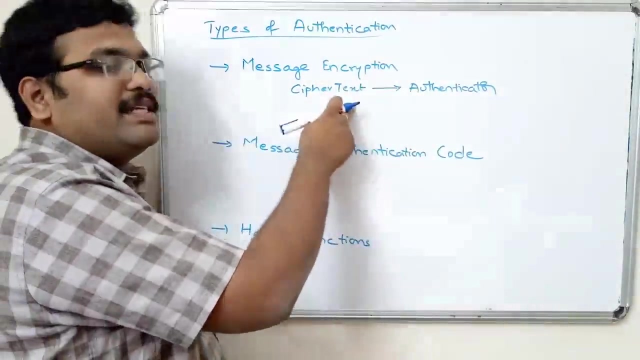 message encryption: the ciphertext. the ciphertext will itself acts as an authenticator. so the sender should be authenticated by the receiver and similarly the receiver should be authenticated by the sender. and this process will be done only through the ciphertext. so that's why we call it as authenticator. so here the ciphertext itself acts as an 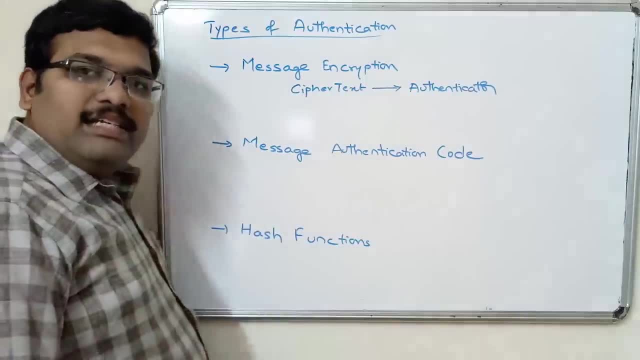 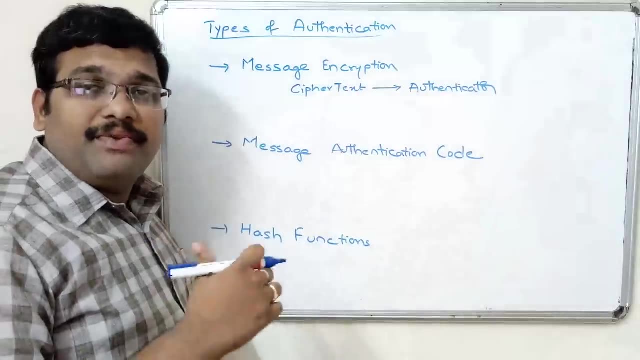 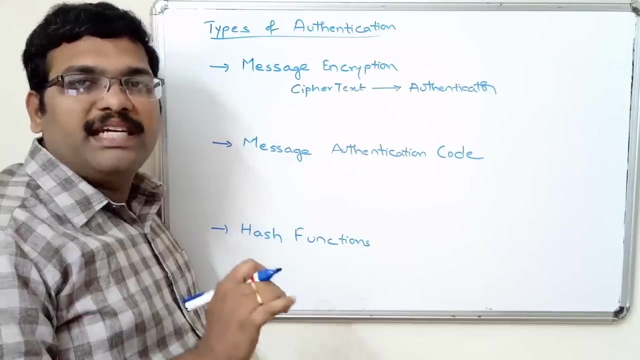 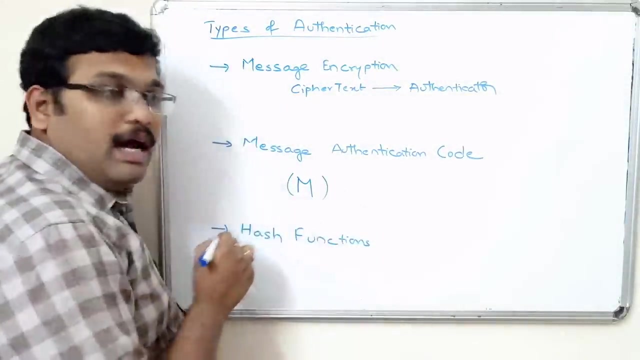 authenticator. in this message authentication code we will have some authentication functions, so we have to apply these authentication functions on the plaintext along with the key, which produces a fixed length code that is called message authentication code. so consider the plaintext, apply the authentication function along with the 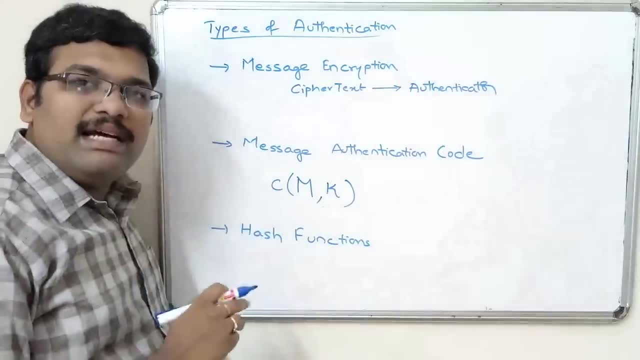 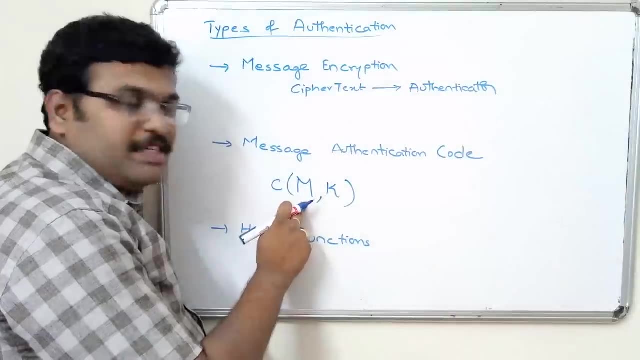 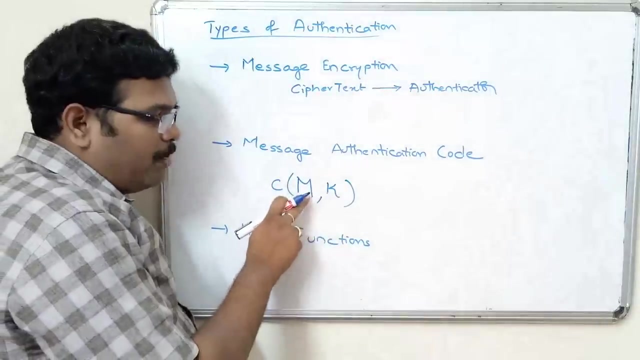 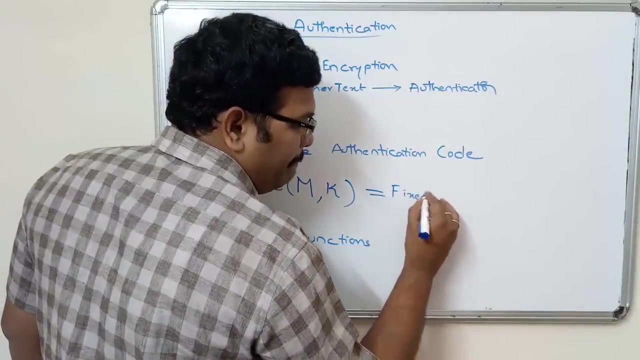 key. so here C represents the authentication functions, so C of M, comma, K. M stands for plaintext message and K stands for the simple key. so applying the authentication functions on plaintext message along with the key will produces a fixed length code, fixed length code which we will. 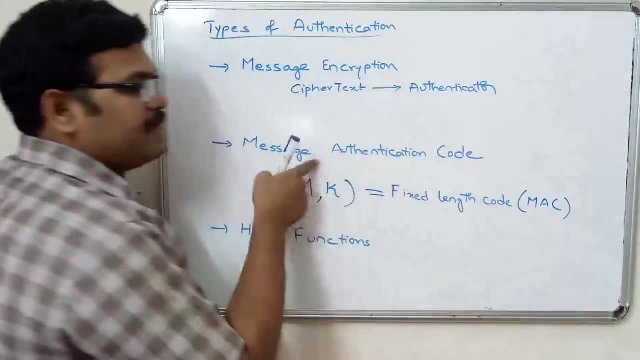 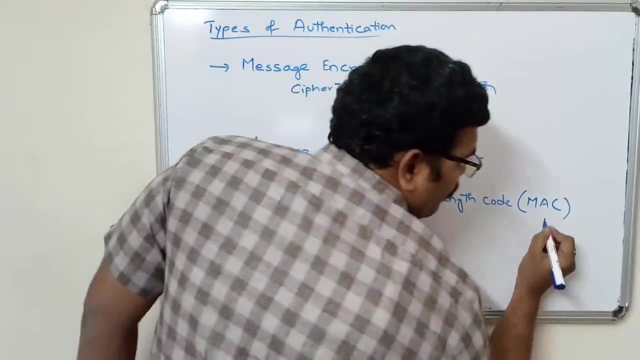 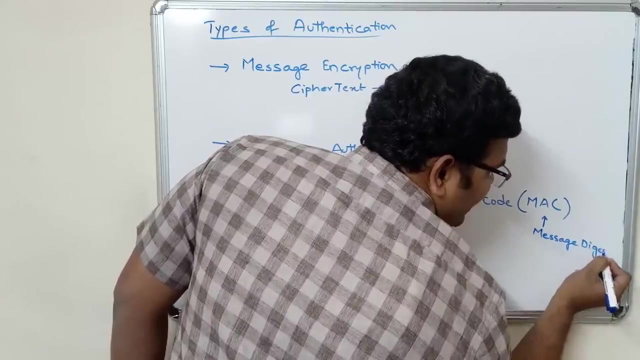 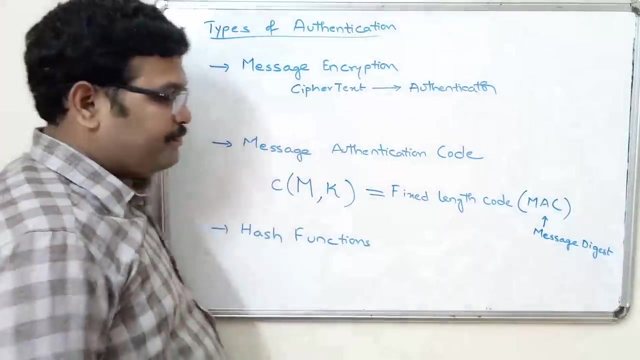 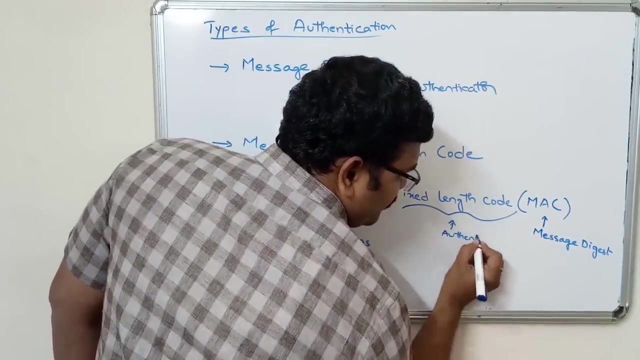 call it as MAC. that is message authentication code. so the output of this message authentication code is MAC. this can also be called as message digest- message digest, right? so this is a fixed length code and this will be acting as an authenticator here. so in the second function, I mean in the second category, there is message. 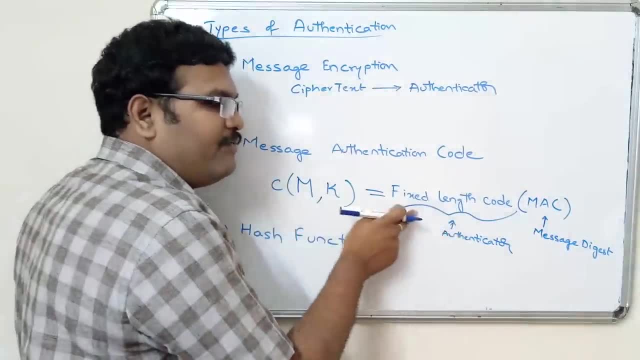 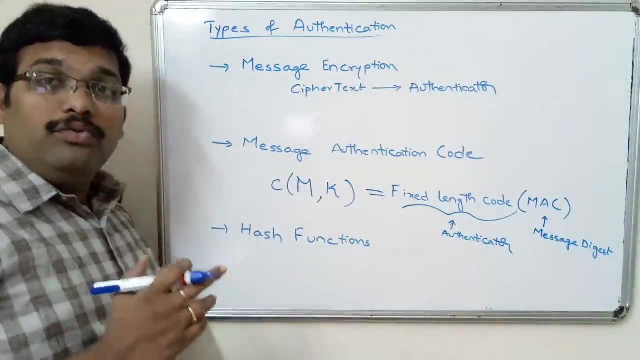 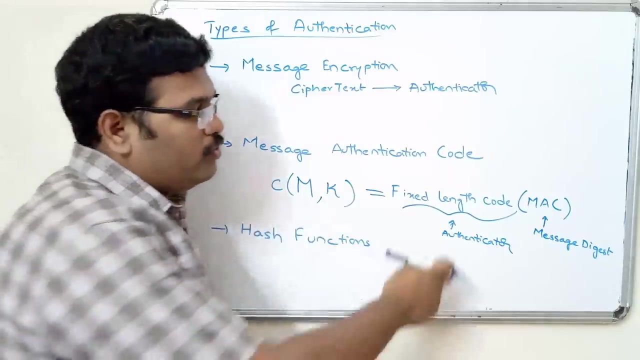 authentication code. we will get a fixed length code which is a MAC or message digest which acts as an authenticator. so in order to sender- I authenticate, I mean in order to authenticate by the sender or a receiver- we have to use this fixed length code. and coming to the third one, 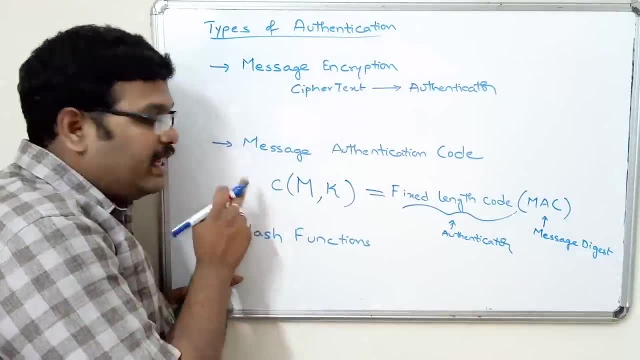 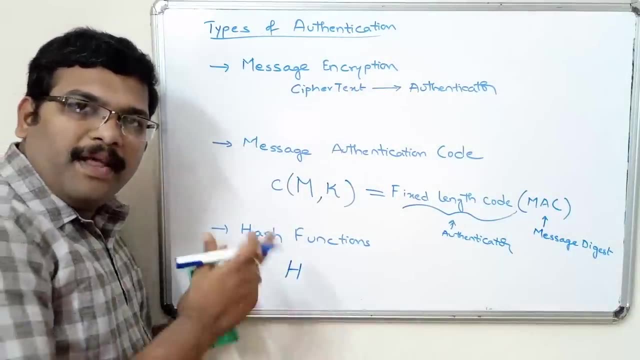 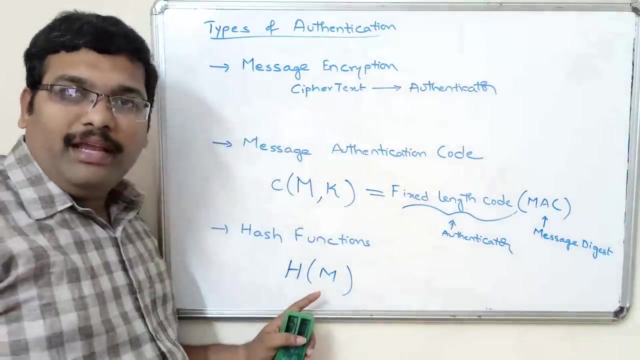 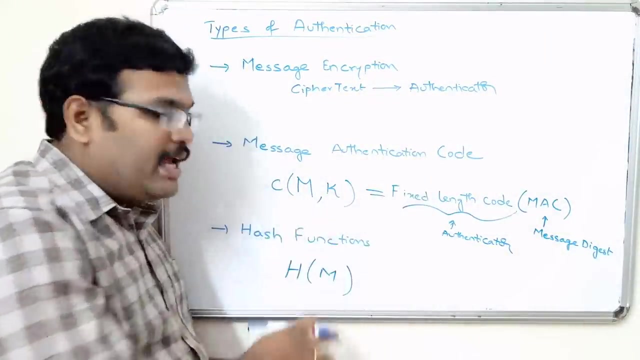 third one is also similar to the message authentication code. here we will apply hash functions, so H represents the hash functions. so applying these hash functions on a plain text message, that is, M, which is independent of key. in the second case we are using the key, so this message authentication code depends upon the key. 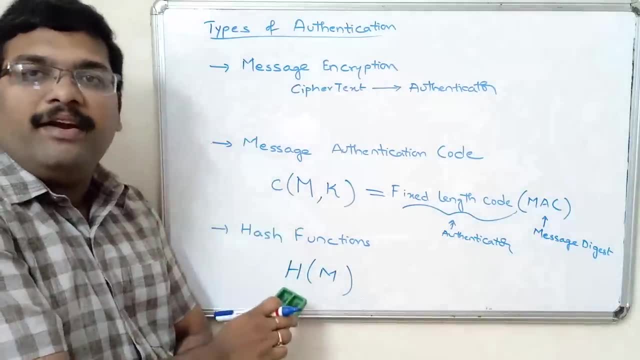 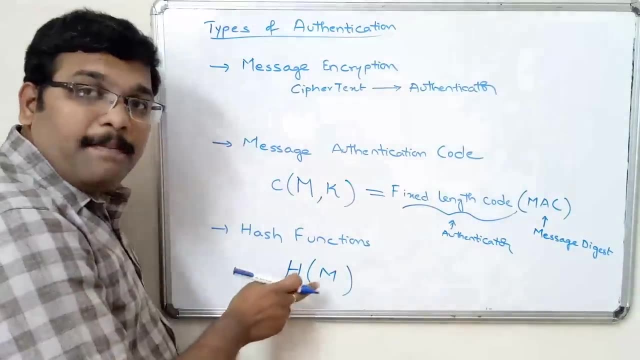 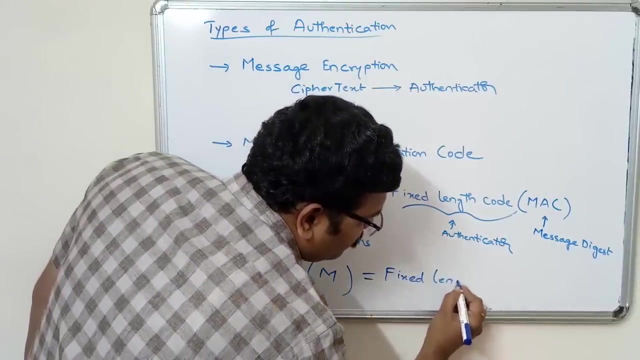 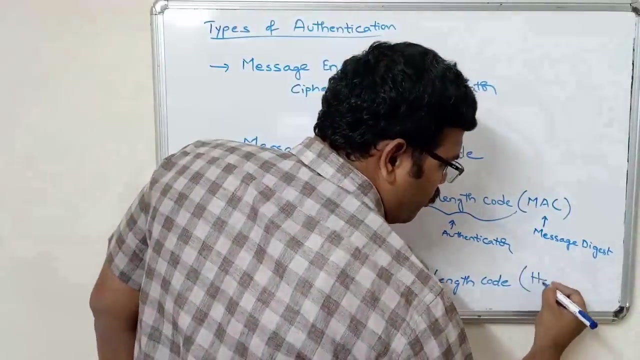 and this hash functions is independent of key, so we should not use the key for generating the authenticator. so hash functions. applying the hash functions on the plain text message will also produce the fixed length code, which is also called as hash code. it is represented as H. 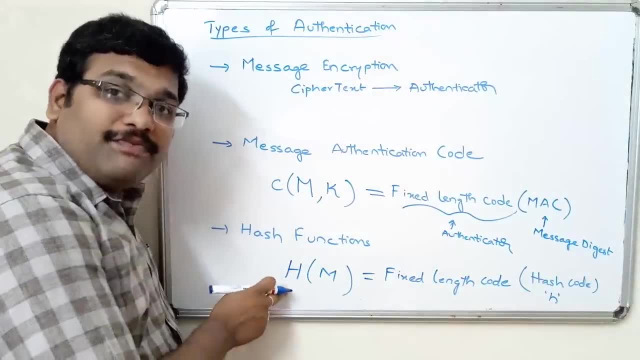 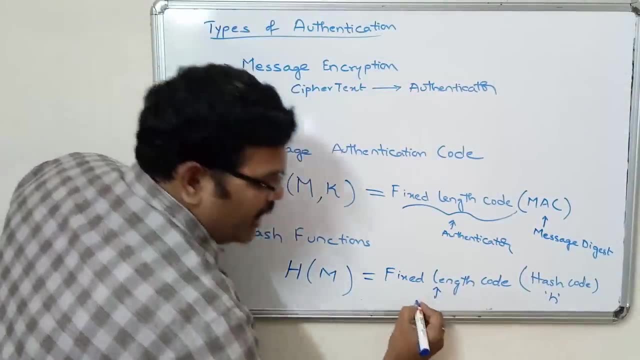 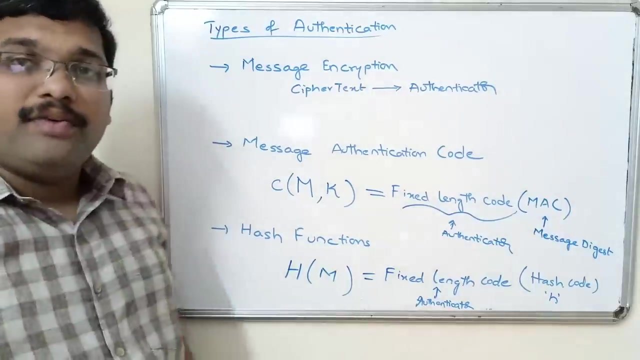 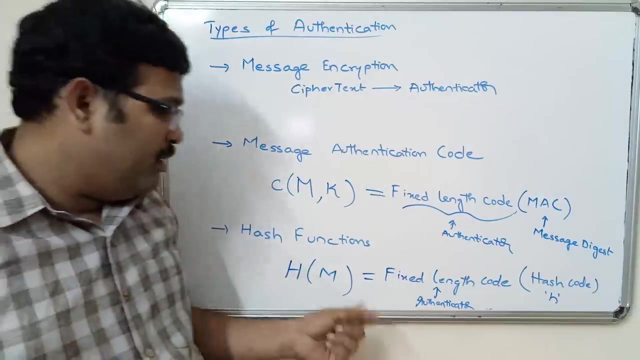 small h. so here the capital H represents the hash function, small h represents the hash code, and this fixed length code will act as an authenticator. so if the sender wants to authenticate by the receiver and the receiver wants to authenticate by the sender, we have to use this hash code. 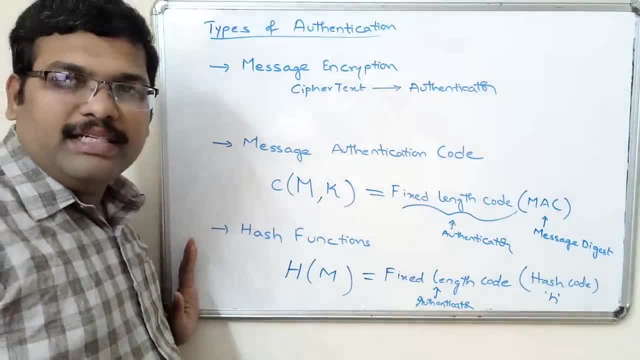 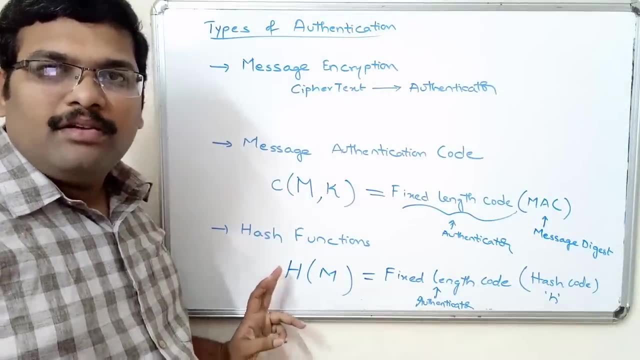 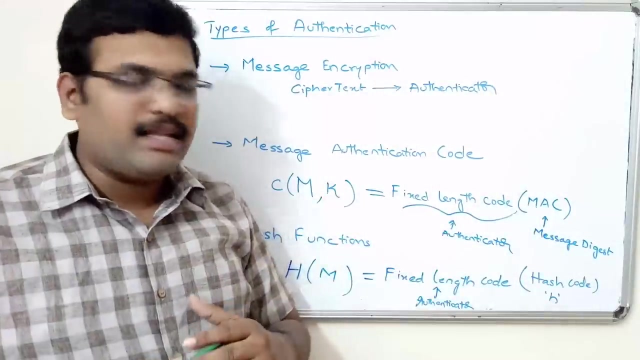 so these are the three categories of authentications, three ways we can achieve the authentication message: encryption, authentication code and hash functions. so let us see how this ciphertext acts as an authenticator and here how this MAC acts as an authenticator and here how the hash code acts as an authenticator. 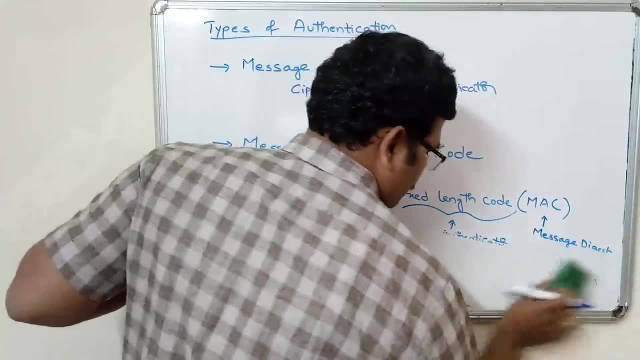 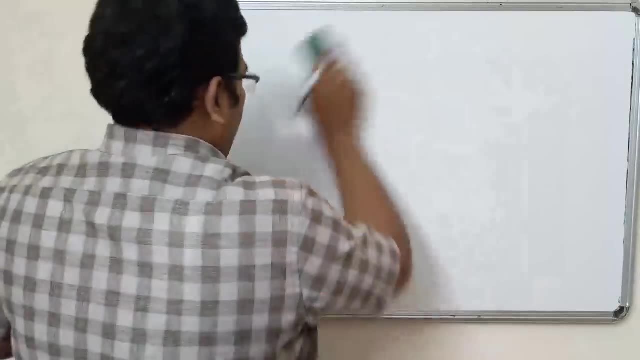 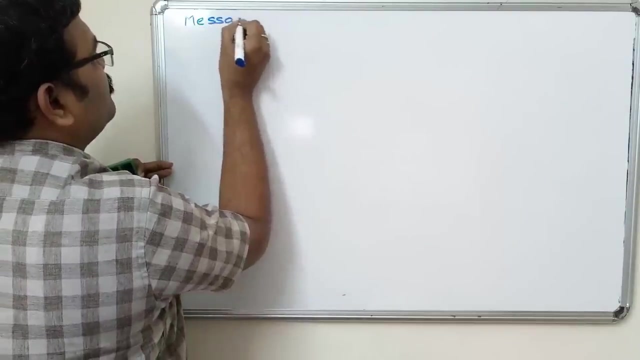 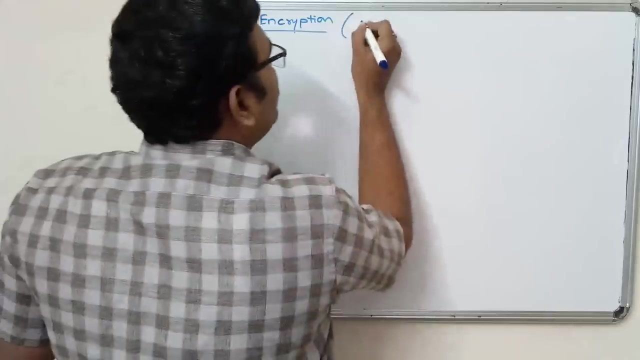 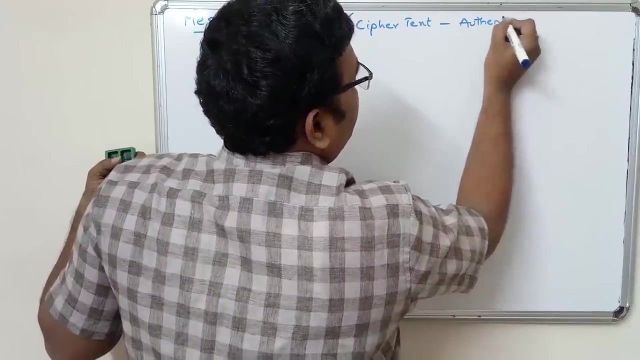 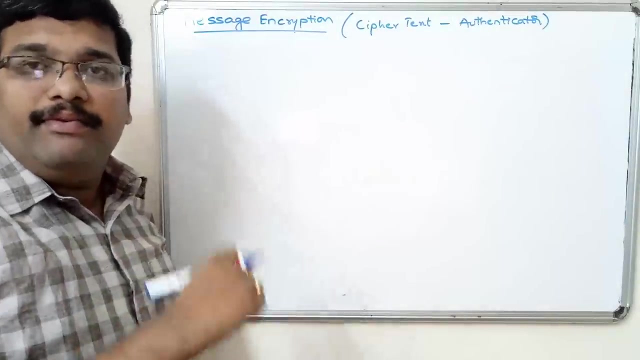 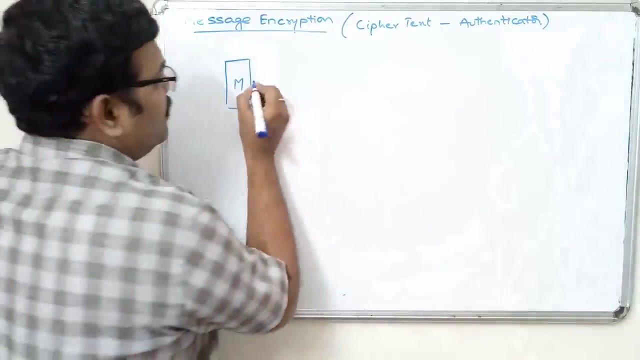 let us look one by one. first message: encryption. so here the ciphertext is an authenticator. so in the first case let us see in the symmetric and then we will go to the asymmetric. consider the plain text message. so this is the plain text message. apply the encryption algorithm. 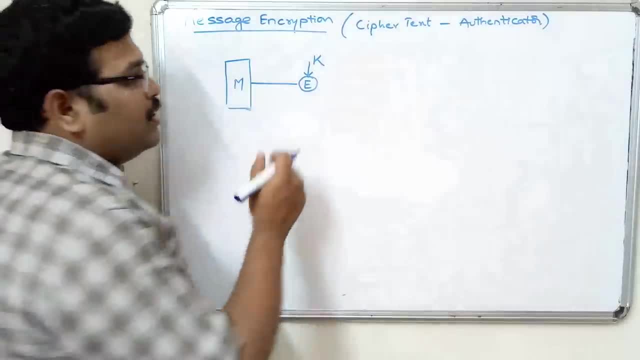 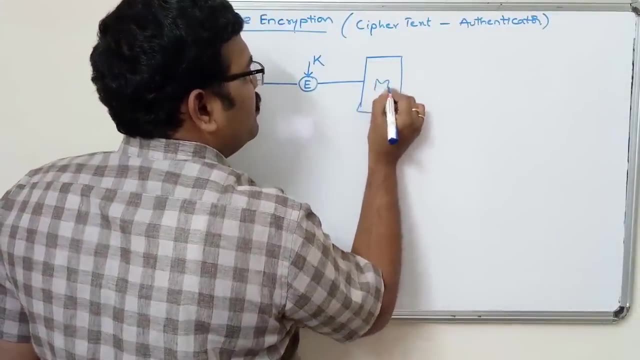 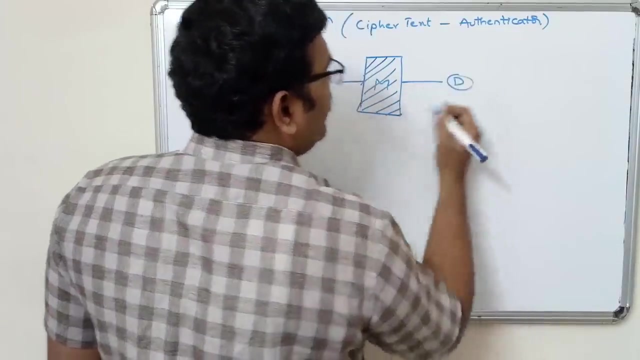 so use the key. this is symmetric, so we have to use the same key at the decryption. so after applying the encryption, we will get the encrypted message and then, at the receiver side, decrypt this encrypted message using the same key so that we will get the plain text message. 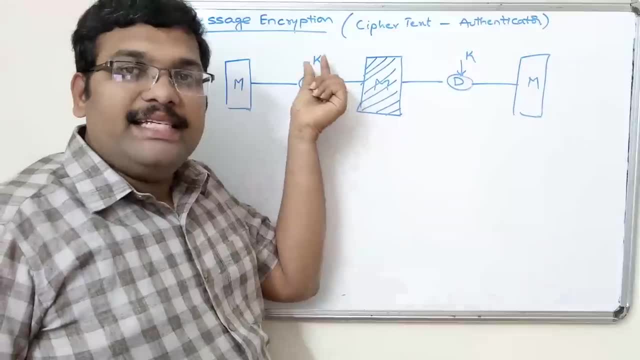 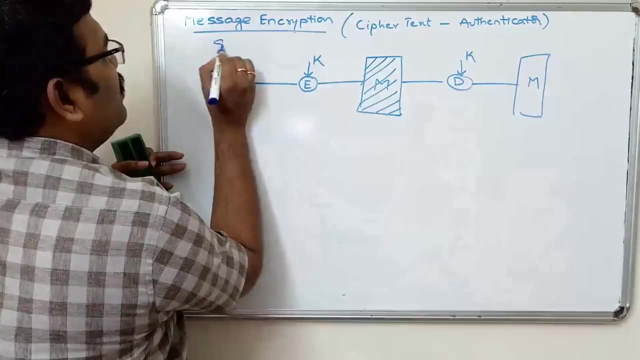 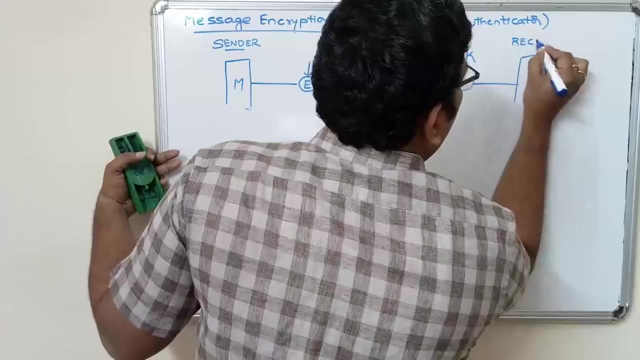 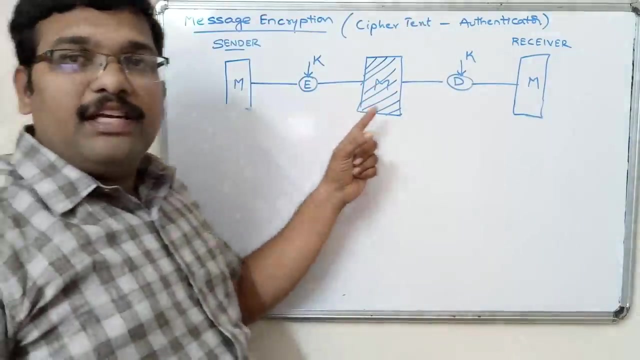 so here we have to share this secret key securely between the sender and receiver. so this is the sender, this is the receiver, right? so the key will not be shared among the different persons. so here the ciphertext only acts as an authenticator. so this is the symmetric encryption. 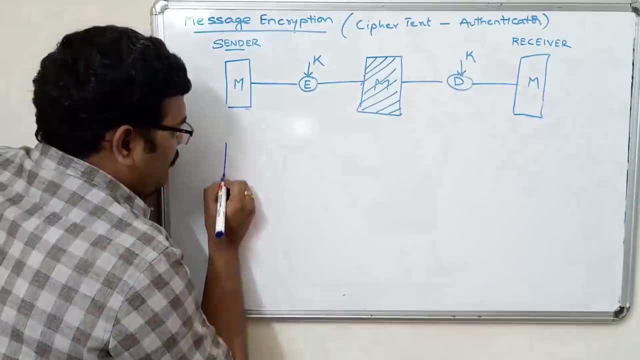 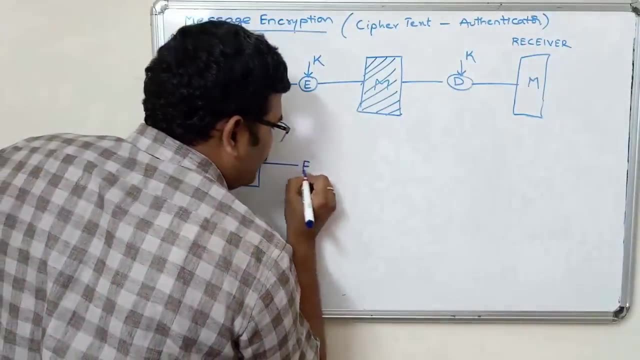 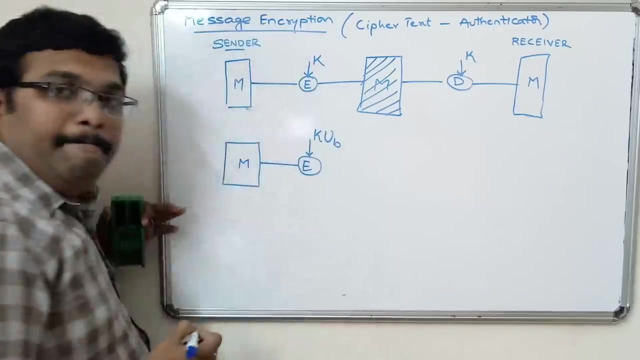 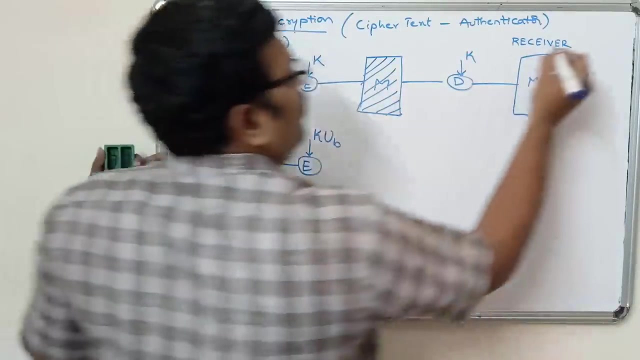 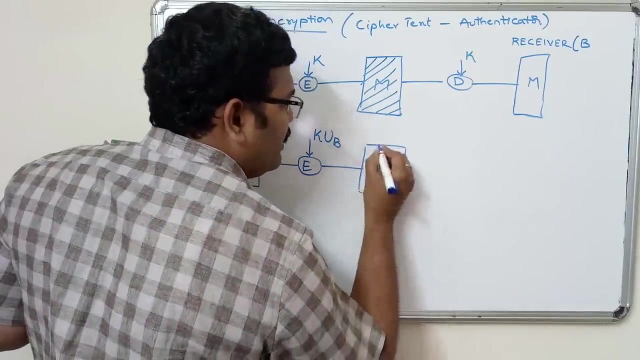 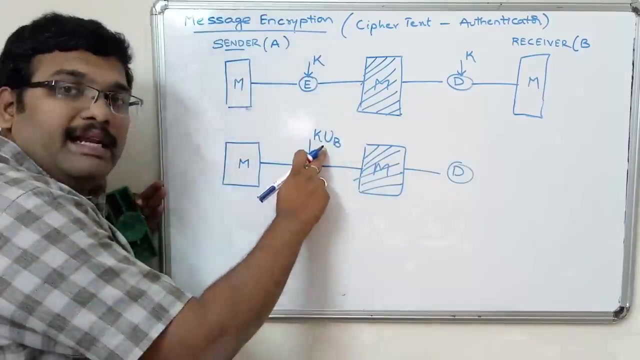 coming to the asymmetric encryption, if you consider the plain text message, encrypt this with public key of B. so, receiver, let it be A B, public key of B, so that we will get the encrypted message and decrypt it. so if we encrypt with public key of B, we have to use the 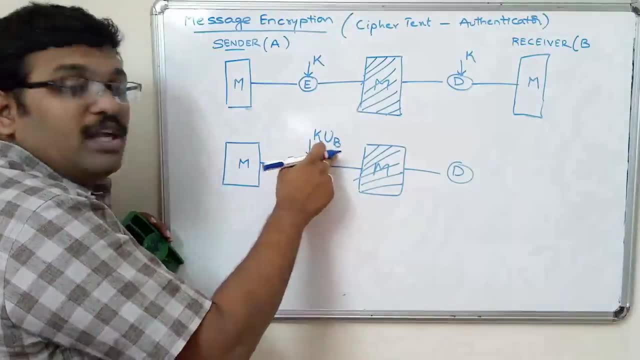 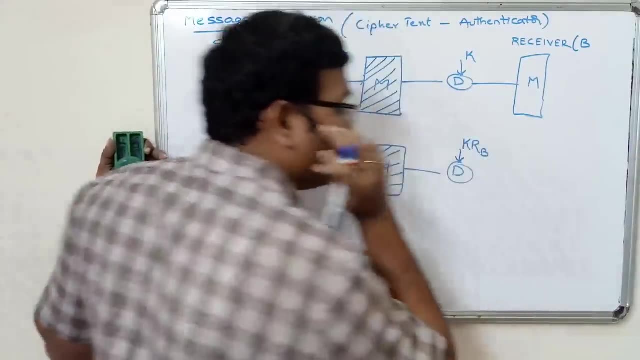 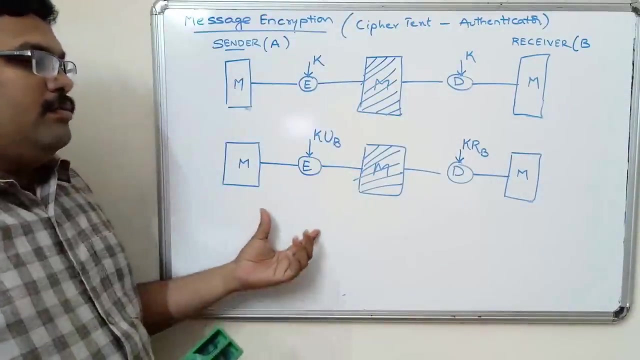 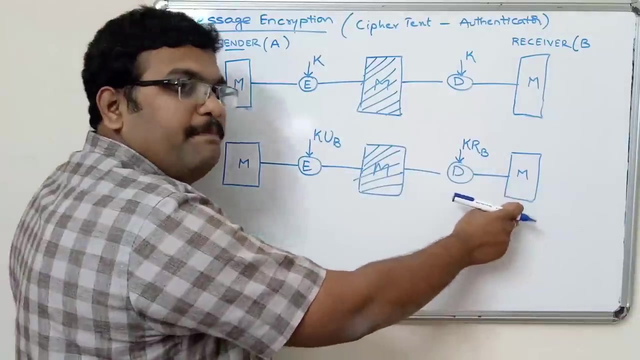 another key of same pair. here we are using the user B public key. so here we have to apply user B private key right, so that we will get the plain text message. so here at the encryption side we are using the public key of user B. that means 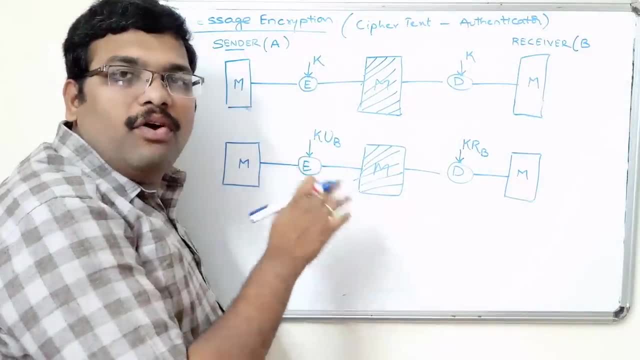 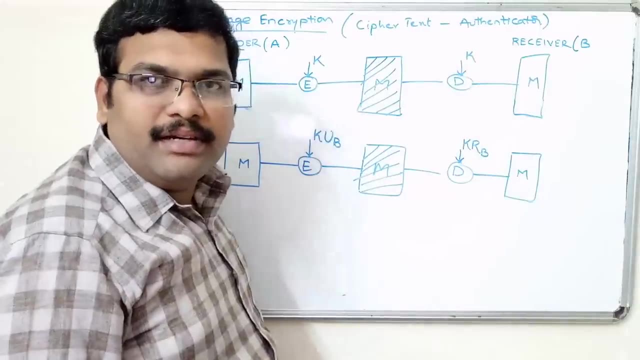 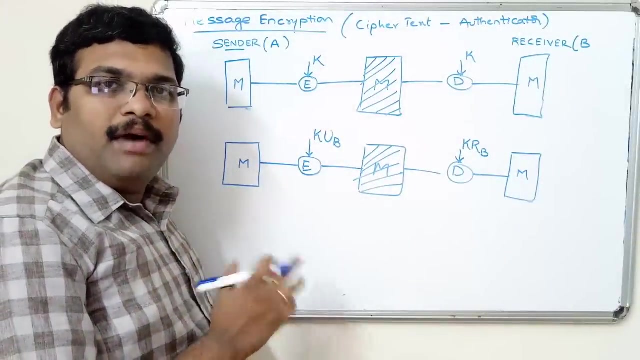 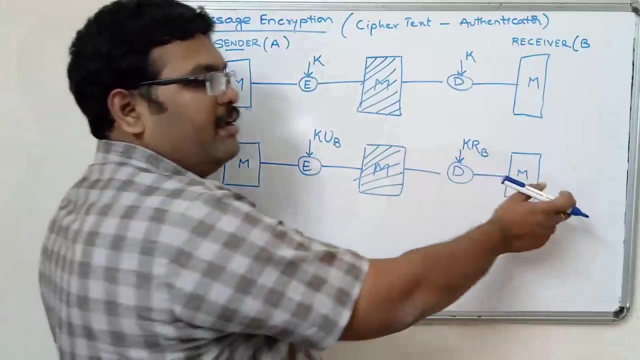 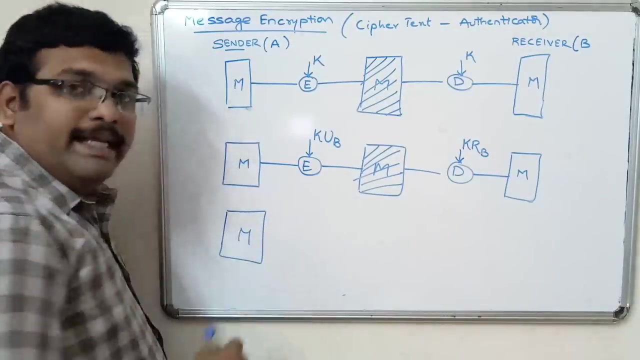 the public key of B is available with all the users in the network, so that any person can encrypt the message and send to the receiver. that means so here the confidentiality is achieved, but authentication is failed. so A is not authenticated by C, now this third one. so in order to avoid this, 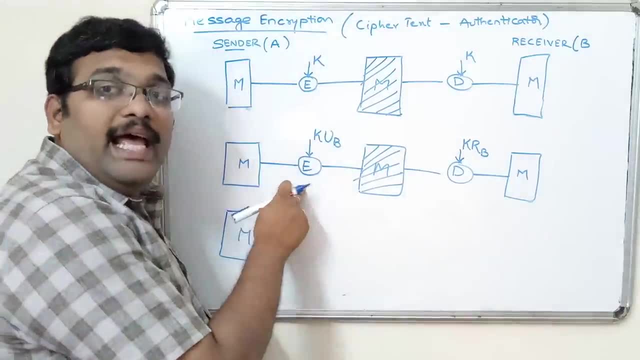 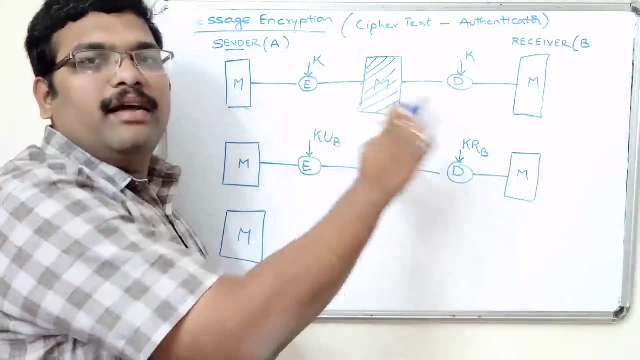 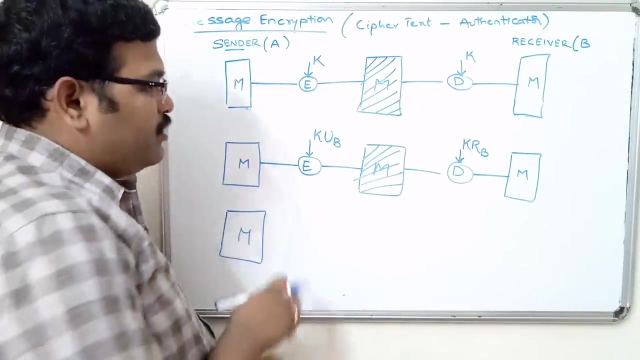 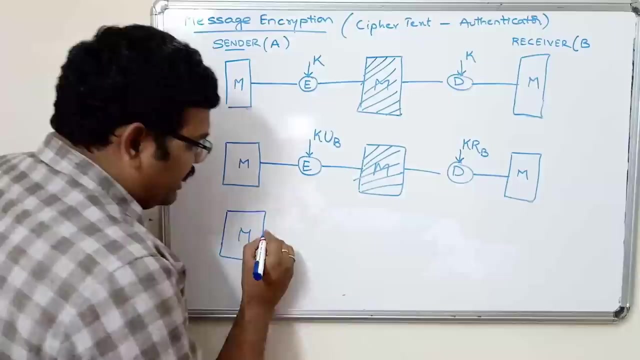 so hope you understood. at the sender side, anyone can send the message. at the receiver side only the B can receive the message, because here we are using the private key of B, which is not A read. so that means authentication fails, only the confidentiality is achieved. so in the third case 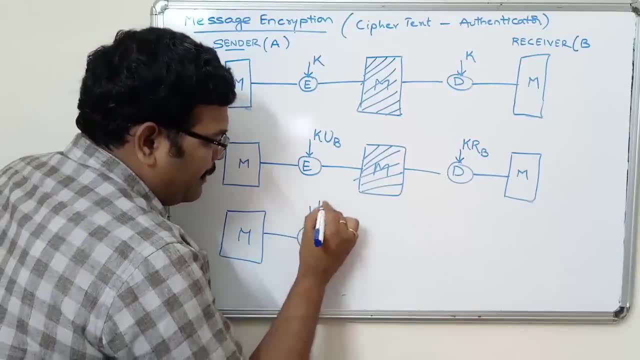 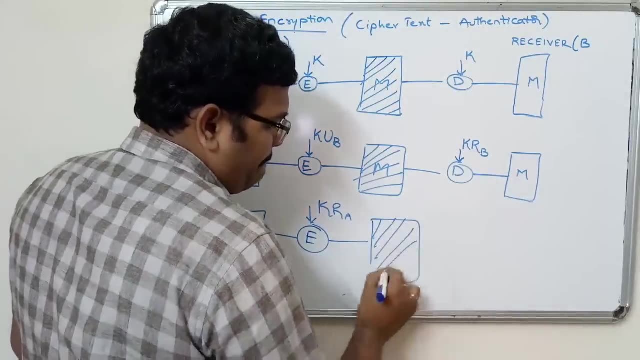 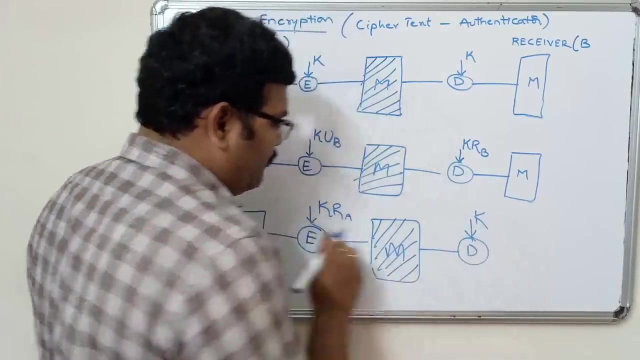 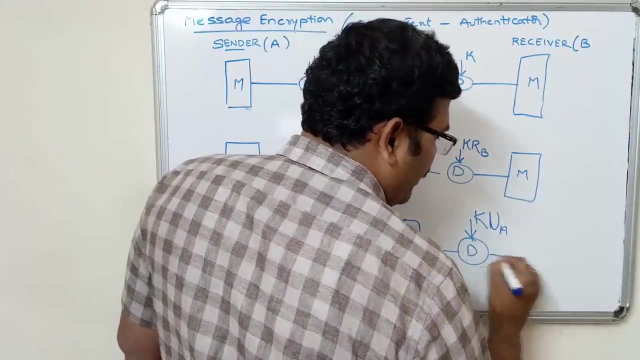 if we apply here the private key of A so that encrypted message will be appeared, and at the decryption side, if we decrypt, so here we are using the private key of user A, here we have to use the public key of user A so that we will get the. 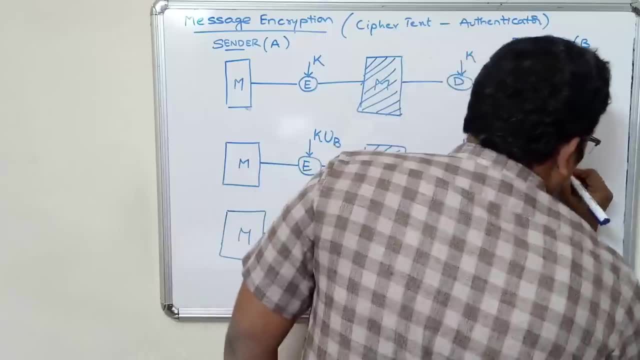 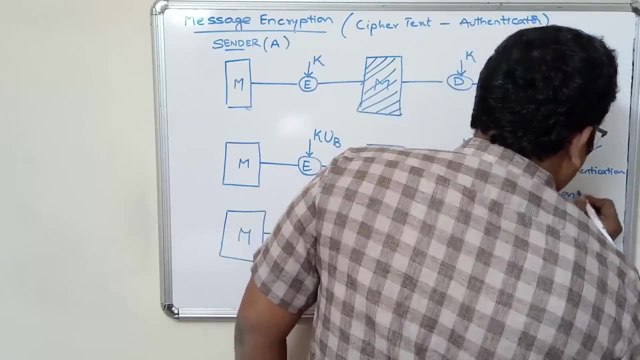 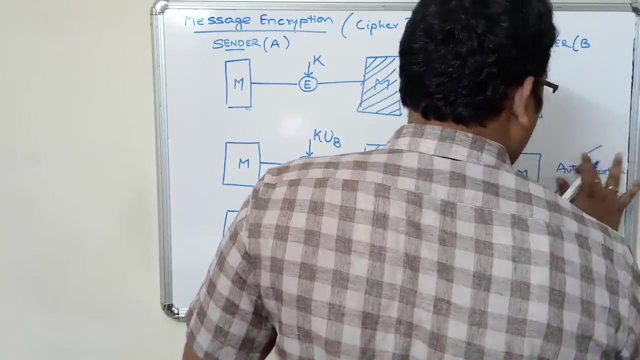 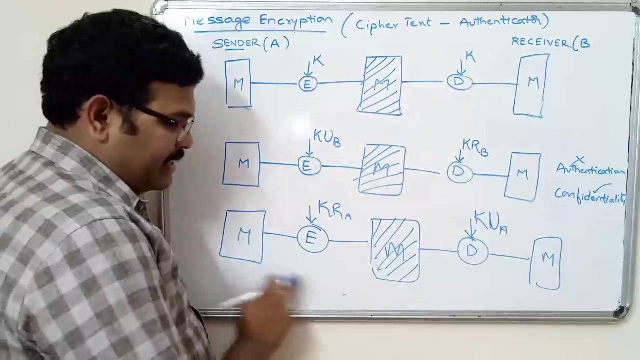 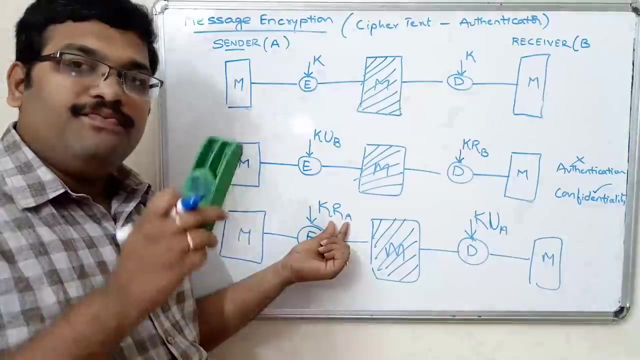 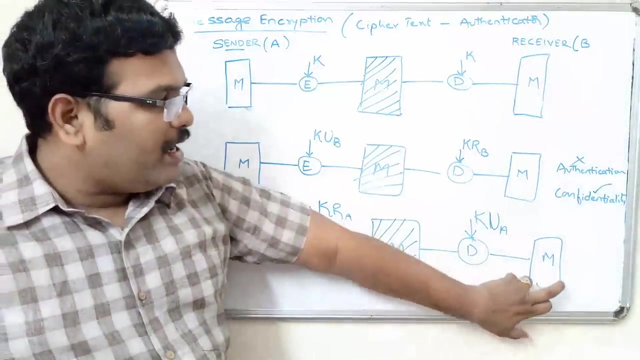 plain text. so in this case, authentication is achieved and, sorry, confidentiality is achieved. authentication is failed in this case- see here at the sender, we are using the private key so that the message will be sent only by the user A. that means user A is authenticated. but at the receiver: 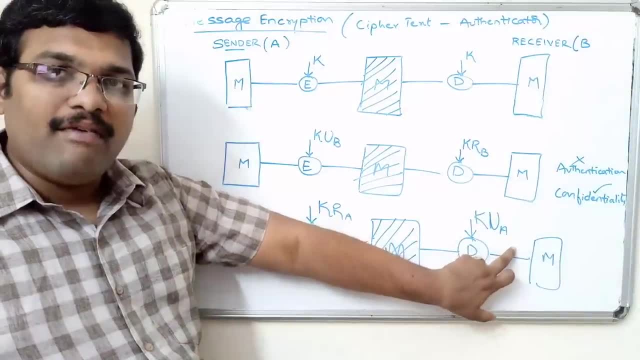 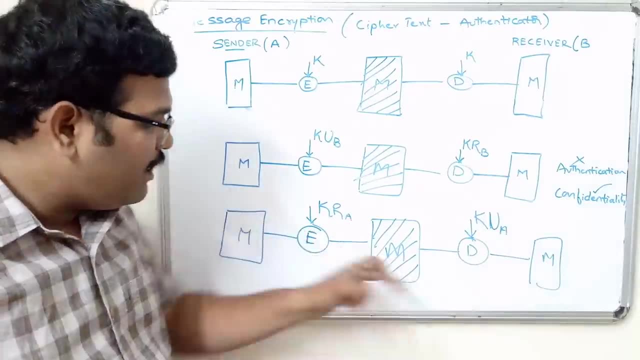 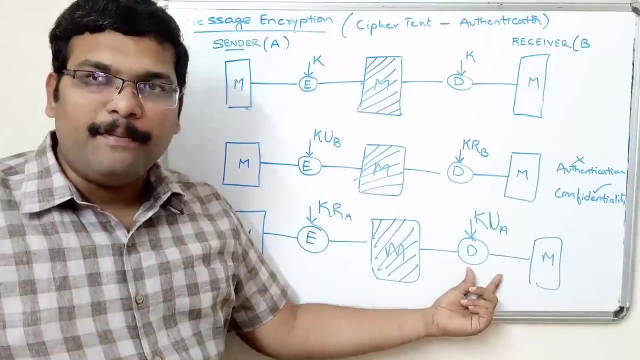 we are using the public key of A, which is available with all the users in the network, so anyone can decrypt the message. so here authentication is achieved, signature is achieved, but confidentiality is failed, because here there is no secrecy, there is no security, because at the receiver side, 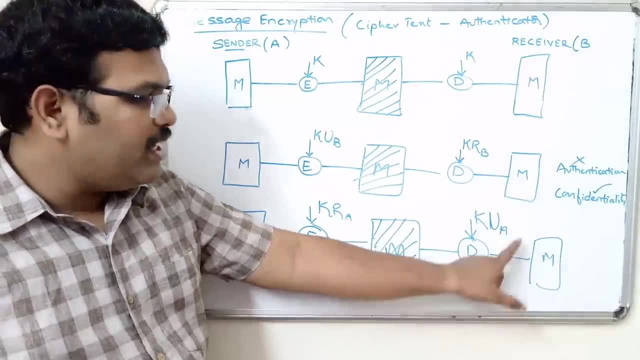 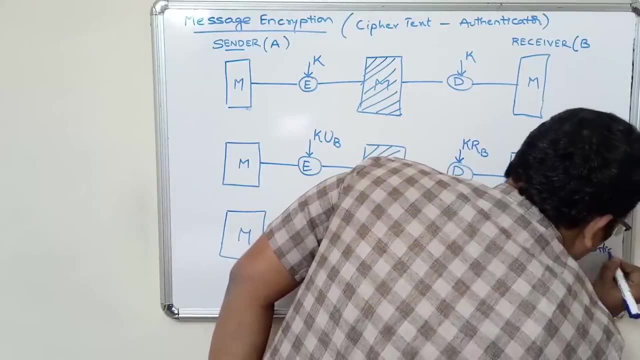 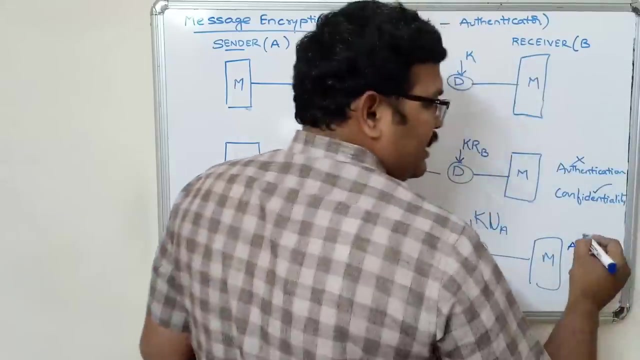 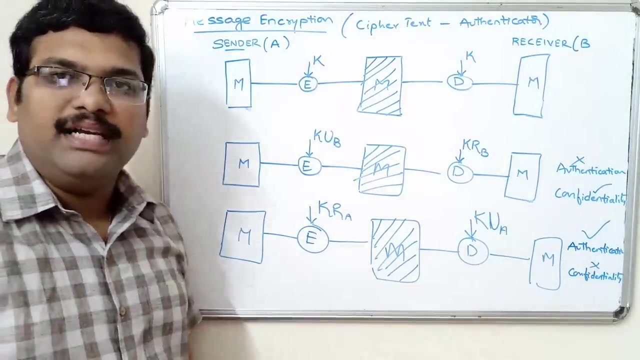 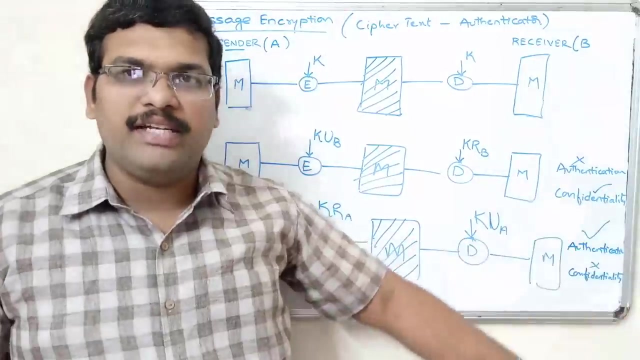 anyone can decrypt this message because here we are using the public key. so in this case- so in this case, authentication is achieved but confidentiality is not achieved- fails the confidentiality. here, authentication fails and confidentiality is achieved. so, in order to get both the authentication and confidentiality in asymmetric 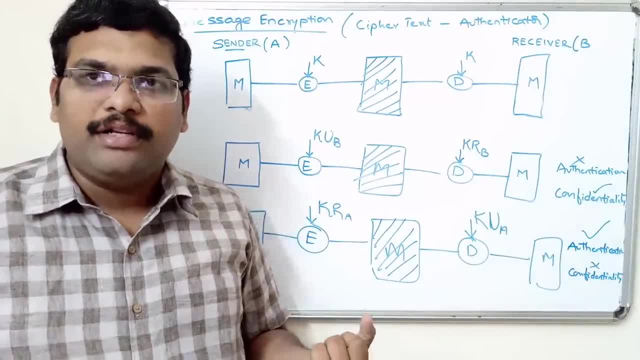 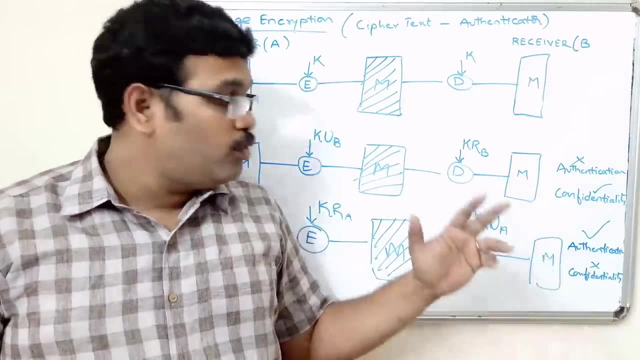 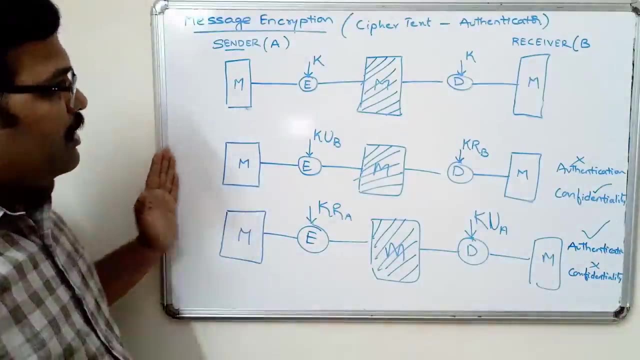 we have to apply the dual encryption. so at the sender side we will use two encryptions and at the receiver side also, we will use two decryptions. so in order to achieve both authentication and confidentiality. so in all these cases, this ciphertext only will act as an authenticator. 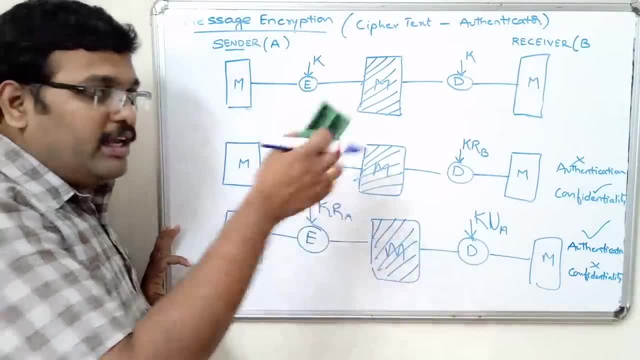 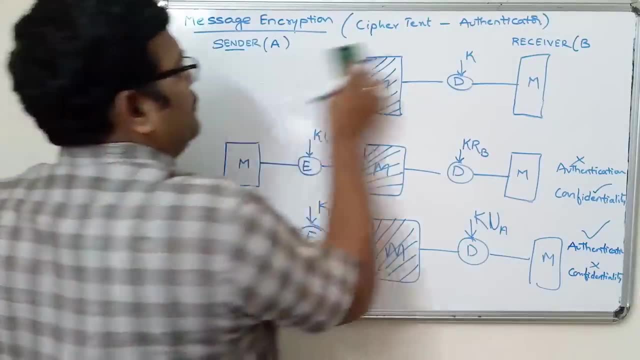 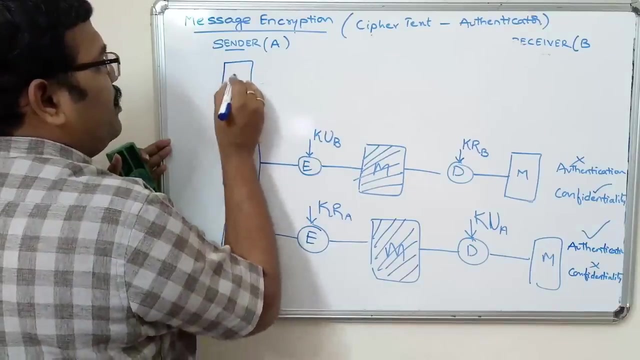 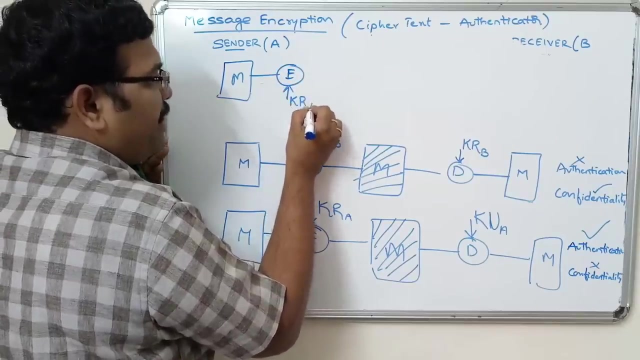 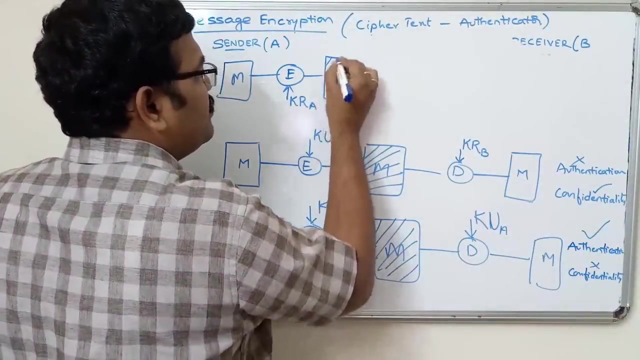 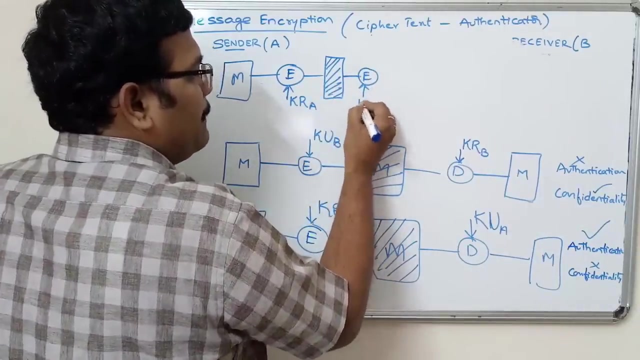 so let us see the third case, which is in which we will achieve both the authentication and confidentiality- see plaintext message- first encrypted with private key of A. we will get the message, which is encrypted using private key, and then again encrypt with with public key of B, so which is available with all the users in the network. 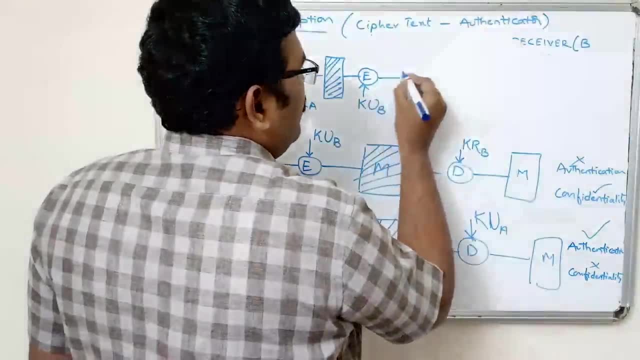 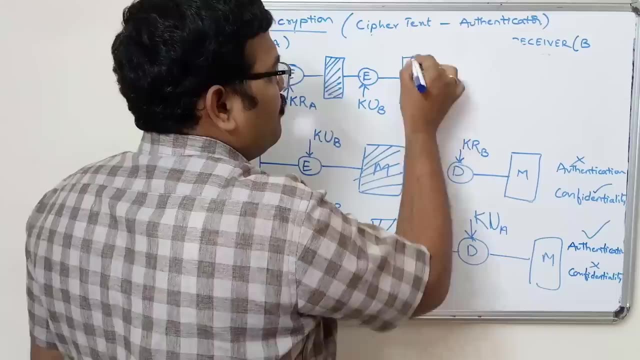 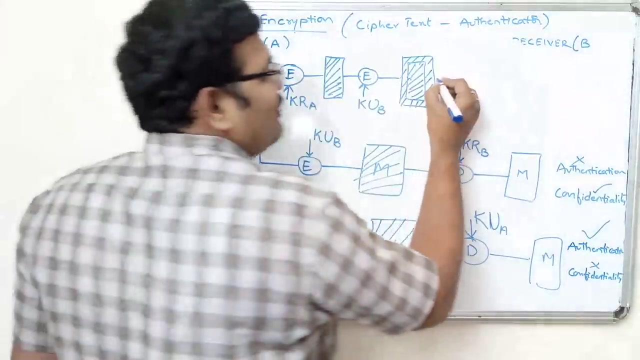 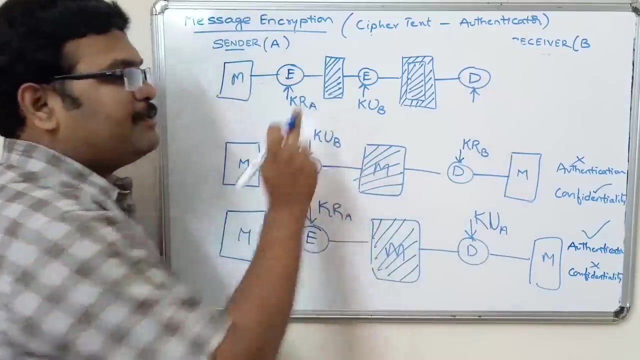 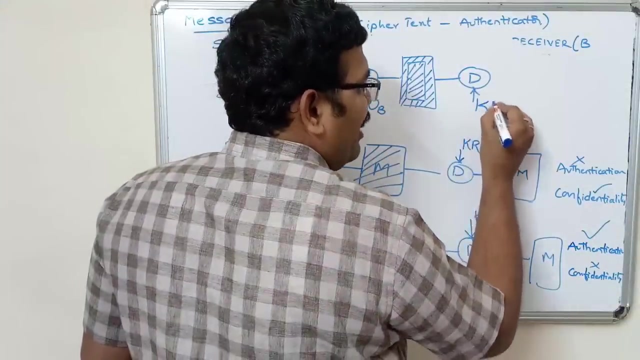 so we can use the public key of receiver and here we will get one more encryption, one more encryption. so in the receiver side, first decrypt. so recent encryption is with KUB. so first we have to decrypt this message with KRB because the recent decryption is KUB. 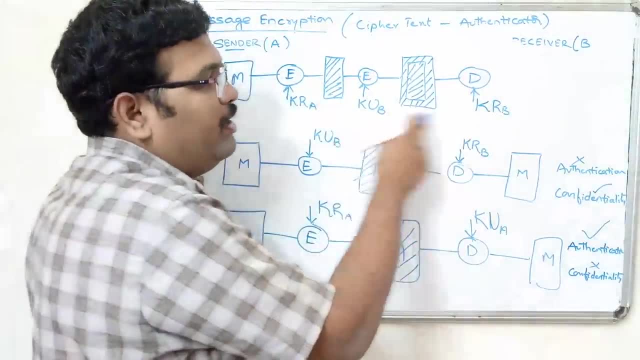 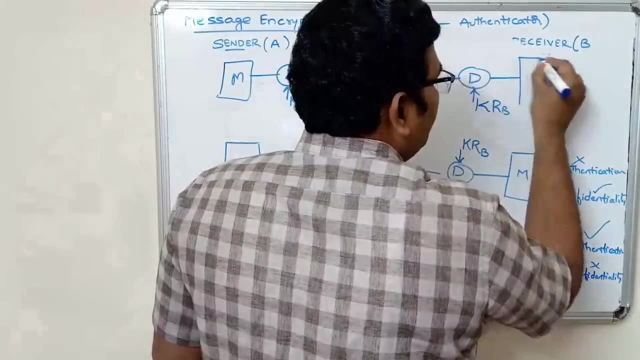 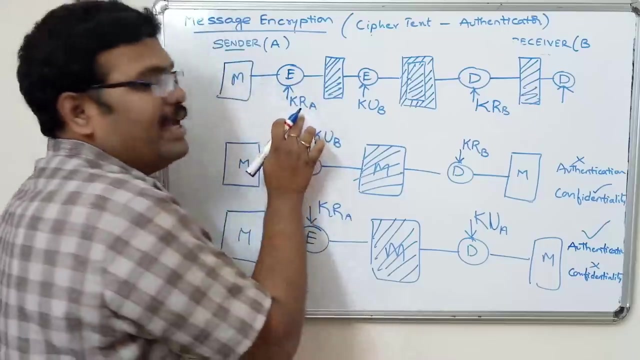 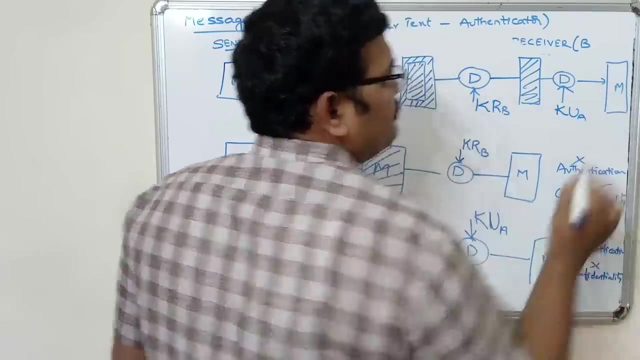 so I mean recent encryption is KUB. here recent decryption must be the first. decryption must be using KRB and after getting the encrypted message again we decrypt using. the second one is KRA. here we have to use KUA so that we will get the plain text message. 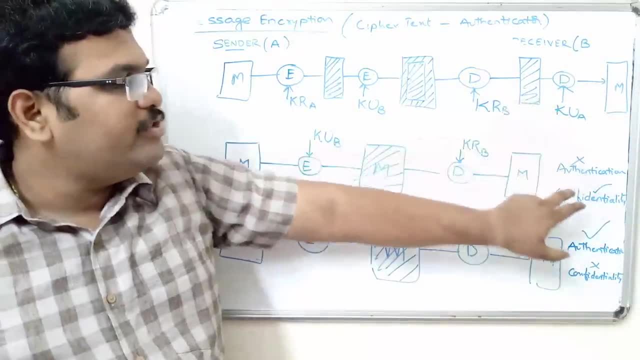 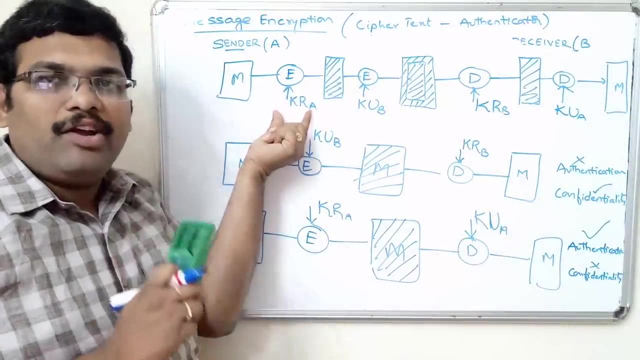 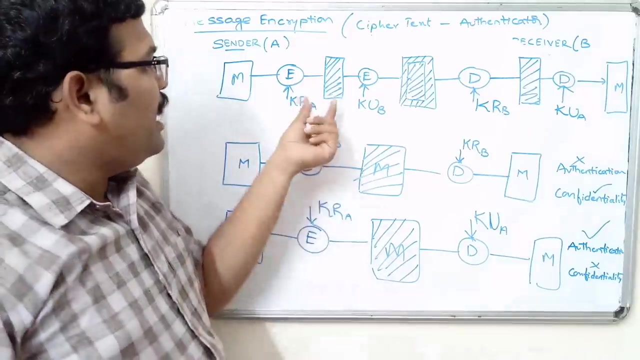 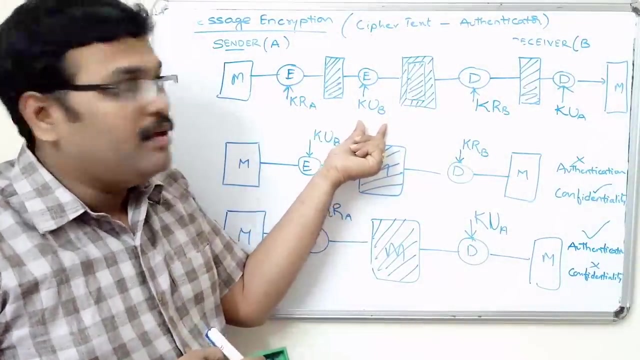 so here, in this case, we can achieve both authentication and confidentiality because at the sender side we are using the private key of sender, which is not shared, so that, compulsory, the sender will send the message. and again we are encrypting the encrypted message using a public key of B, so that at the 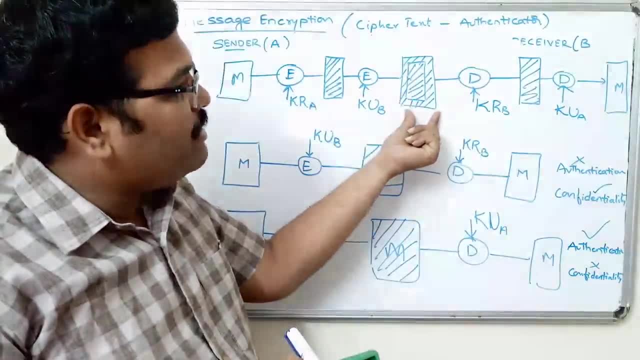 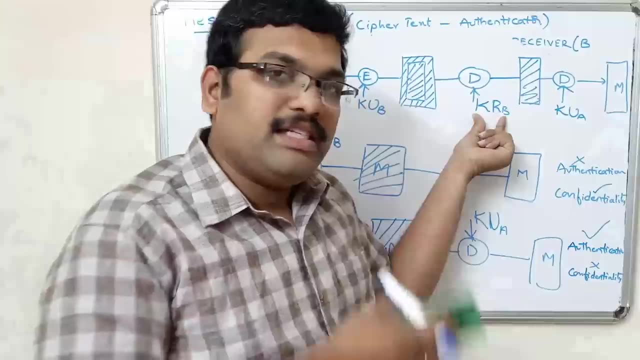 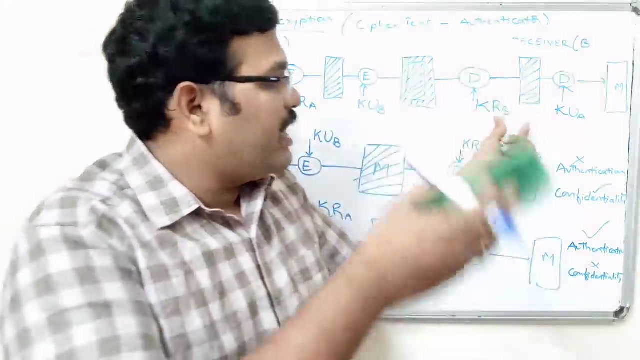 decryption: first we have to decrypt the received message with private key of B. so here also we are decrypting this message with private key which is not shared. only the receiver can receive. I mean, the receiver can decrypt the message in the first level. so after that we can. 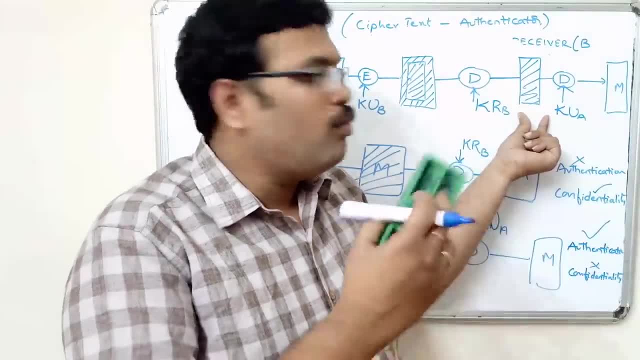 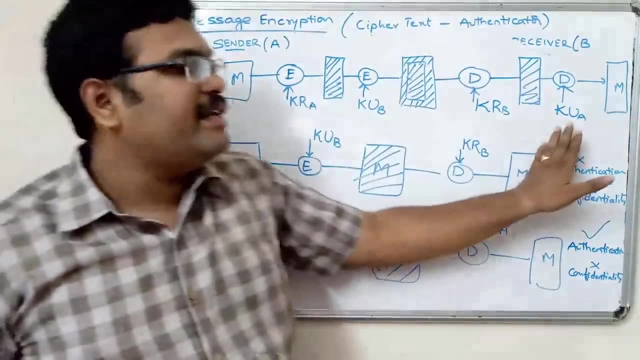 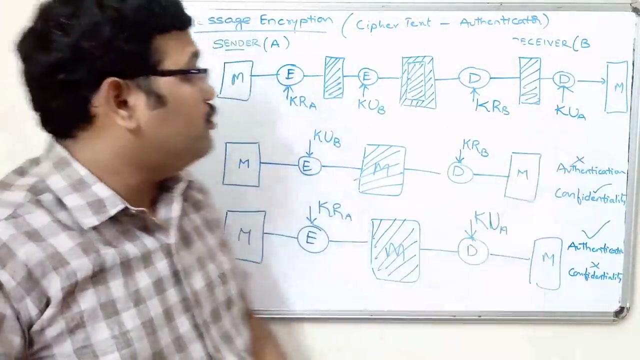 again, we will get the another ciphertext, inner ciphertext, so which can be further decrypted by using public key of A. so sender is authenticated and receiver is also authenticated. so only sender can send the message here, only receiver can receive the message. so this case will achieve all the authentication confidentiality. 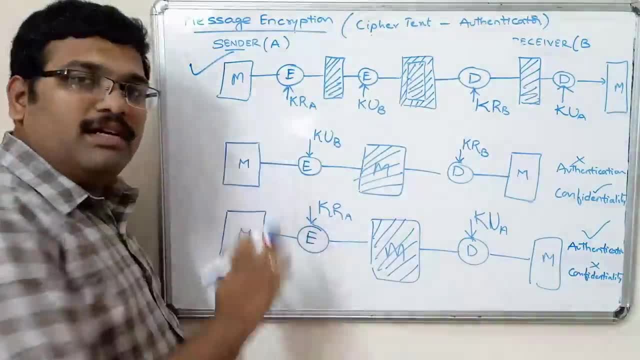 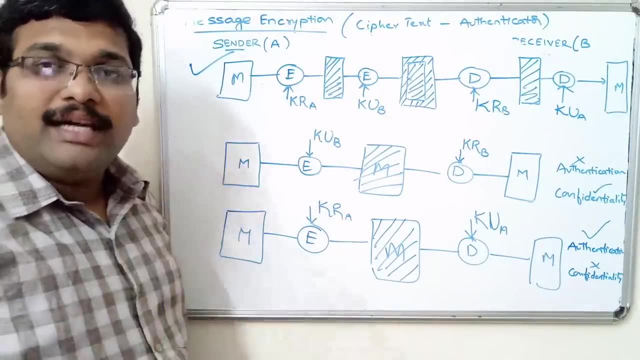 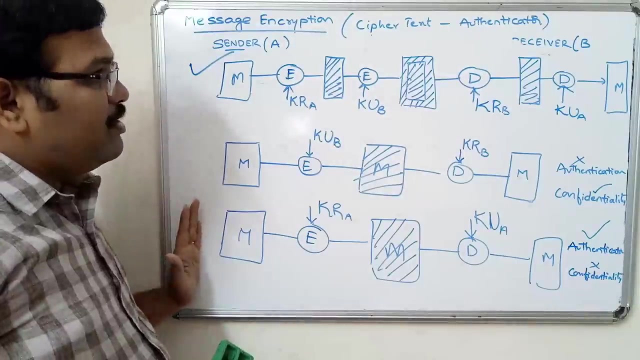 and also signature, because at the receivers- I mean at the sender side- we are encrypting the message using the private key of sender. so that's why we call it as it achieves the signature. so this is the first type of authentication, that is, message encryption. where here we 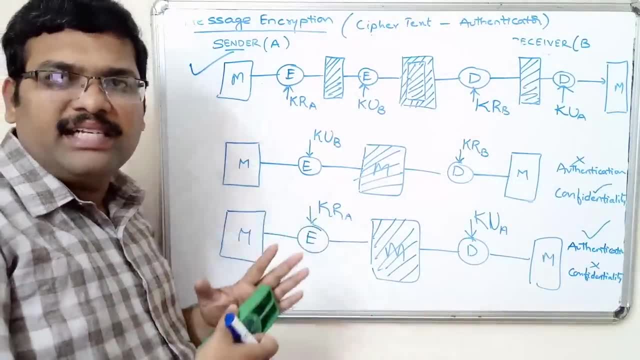 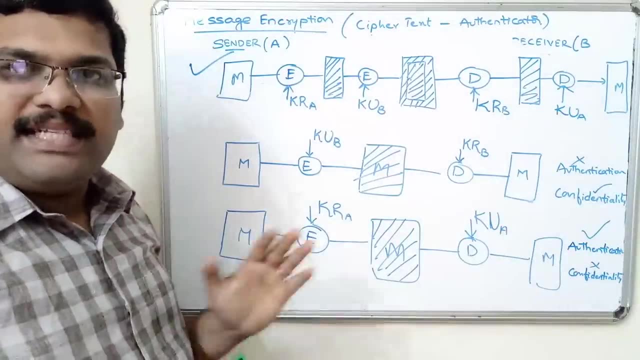 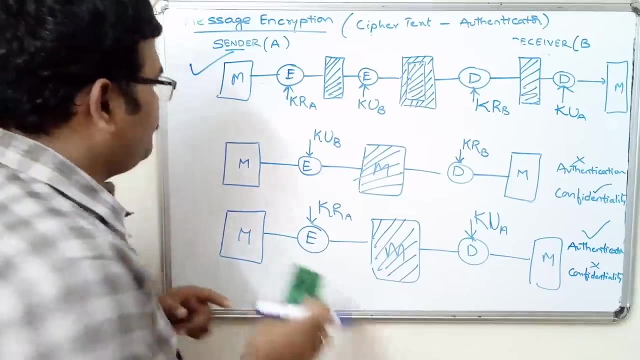 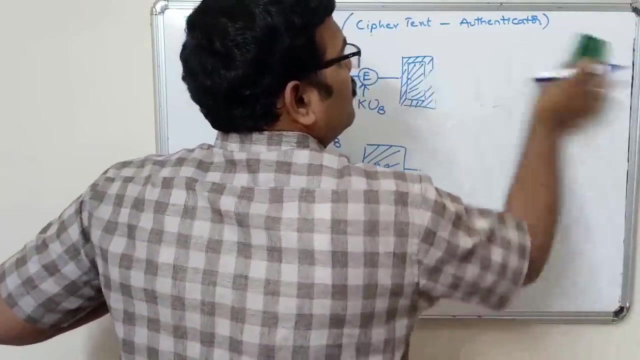 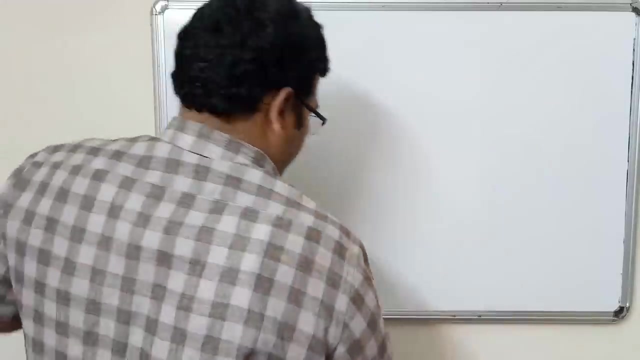 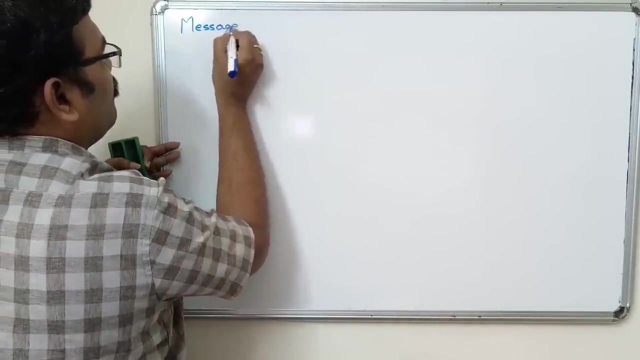 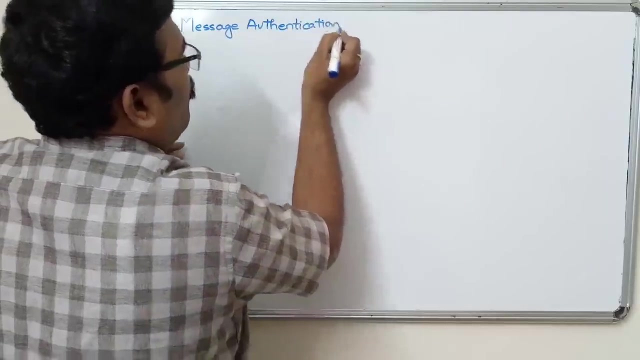 did use any separate functions and any separate keys. just ciphertext only will act as an authenticator, right? so this is the first type of authentication: message encryption. now let us move on to the second one, that is, message authentication code. the second one is message authentication code. message authentication. 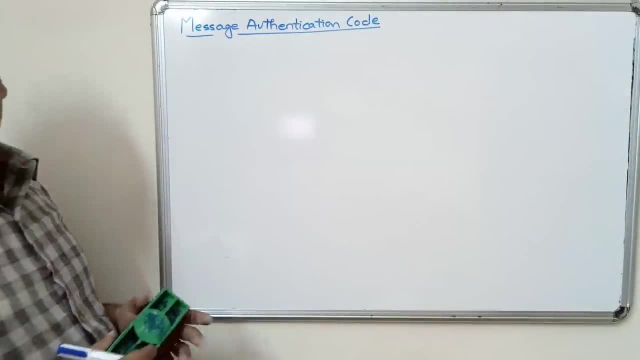 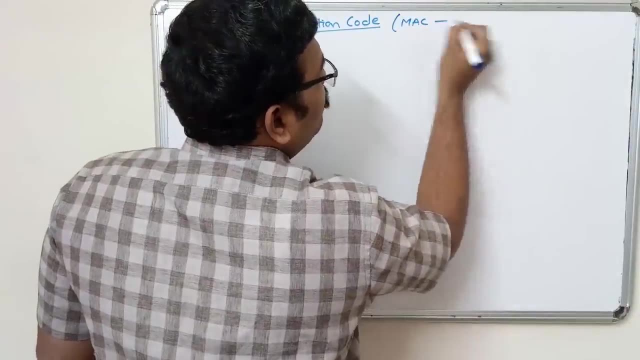 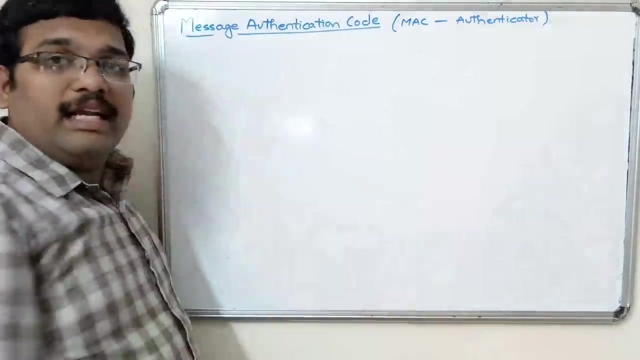 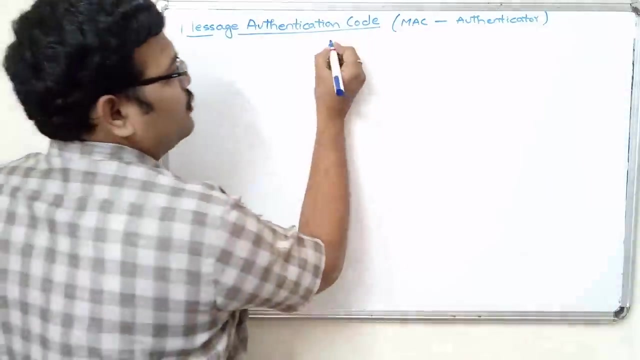 code. so here we have to apply- sorry, here MAC we acts as an authenticator, so we have to generate that MAC. so in order to get that MAC we have to apply the functions of plaintext message along with the key. so C must be applied on message along. 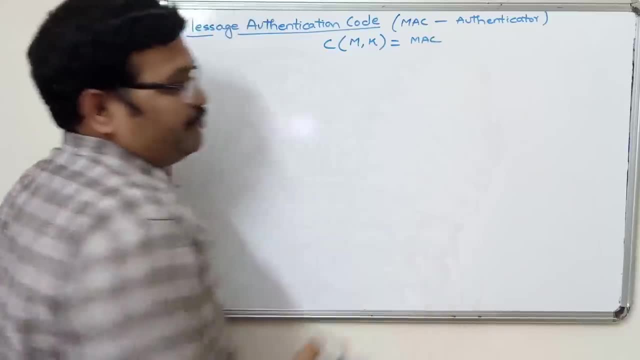 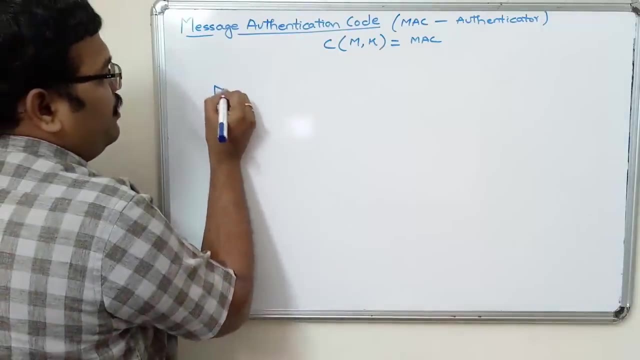 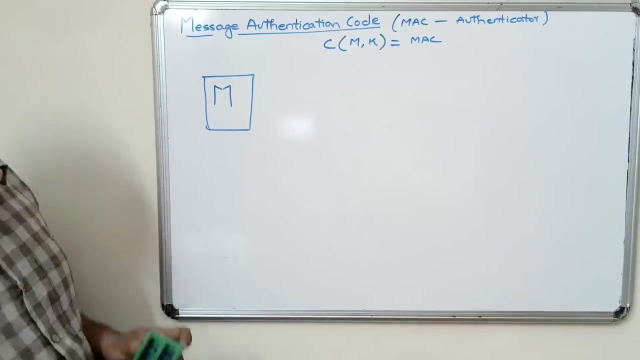 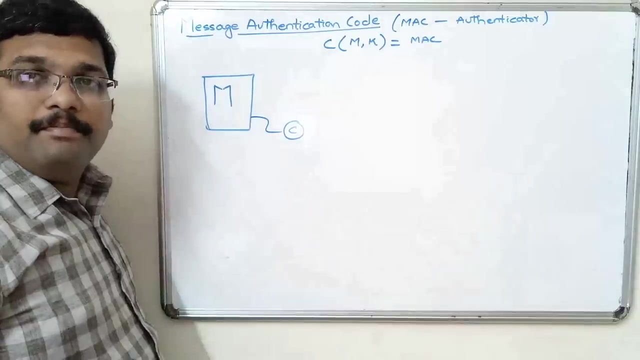 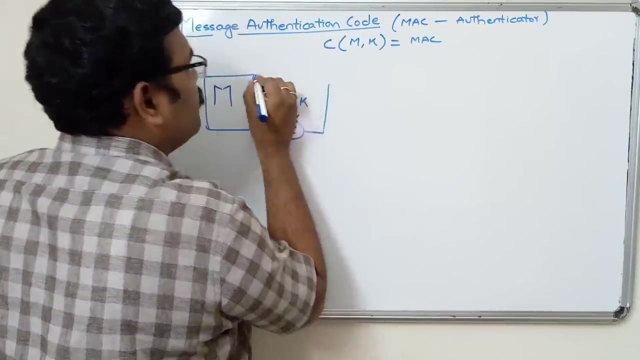 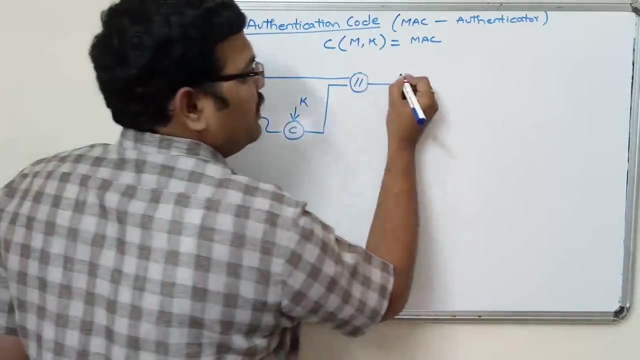 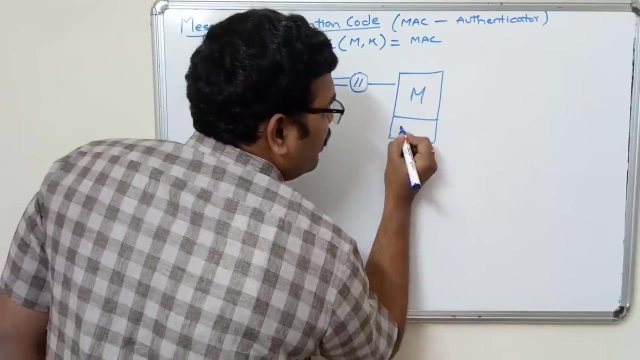 with key which gives MAC and which acts as an authenticator. so here, consider the plaintext message, apply the functions along with key, so that we will get one code which is appended with the plaintext message, so that we will get plaintext message and MAC. so here we will get. 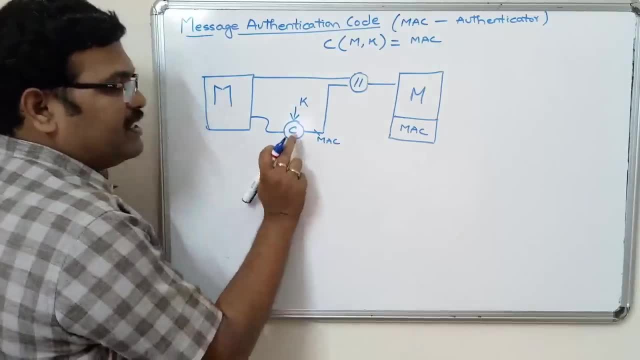 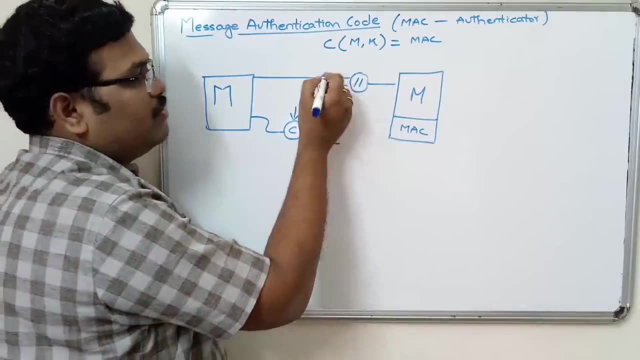 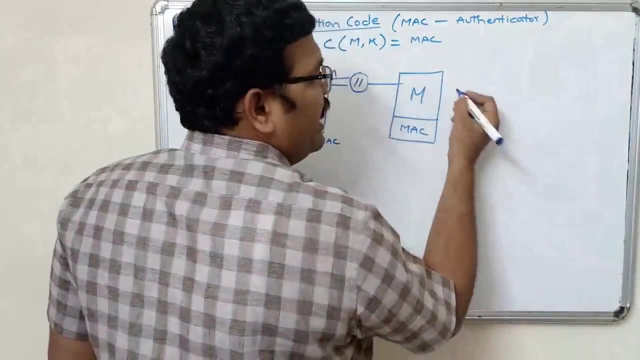 MAC. so we are applying the functions along with the key on plaintext message which gives the MAC which is appended with the plaintext message. so this is plaintext message, right? so this will be sent to the receiver and at the receiver, again, the same functions will be applied on the message. 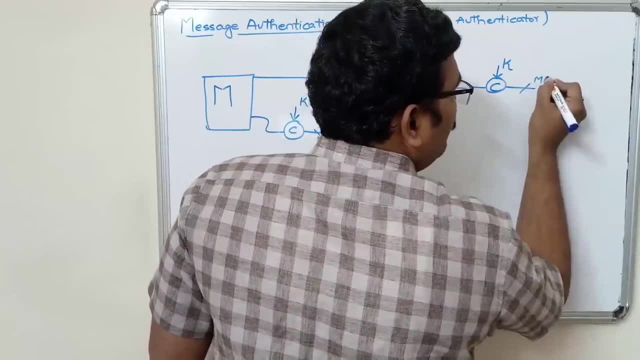 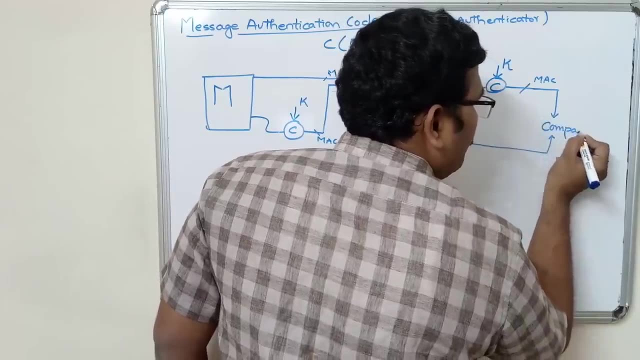 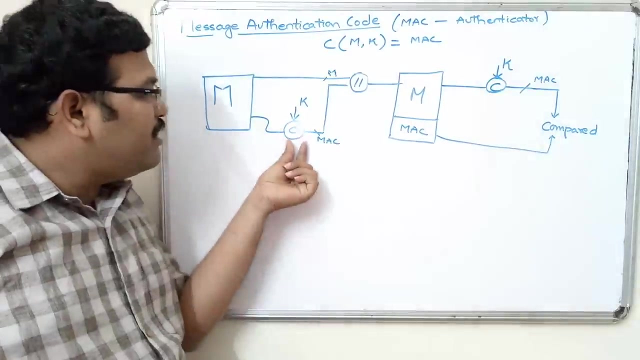 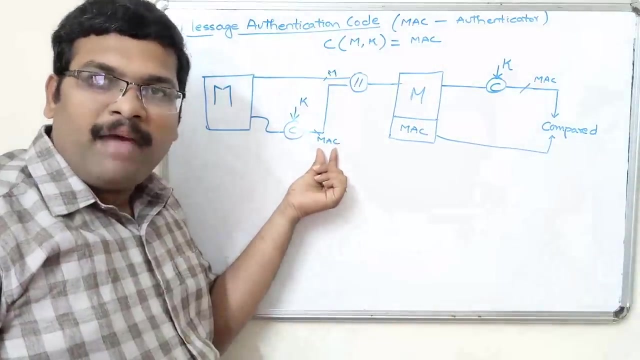 along with the key, so that again MAC will be generated and this appended MAC and generated MAC will be compared. so hope you understood this. consider the plaintext message. apply the authentication functions message- authentication functions- along with the key which generates the MAC- and append this fixed length code. 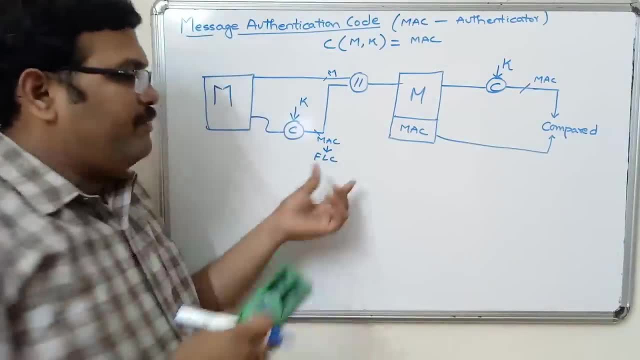 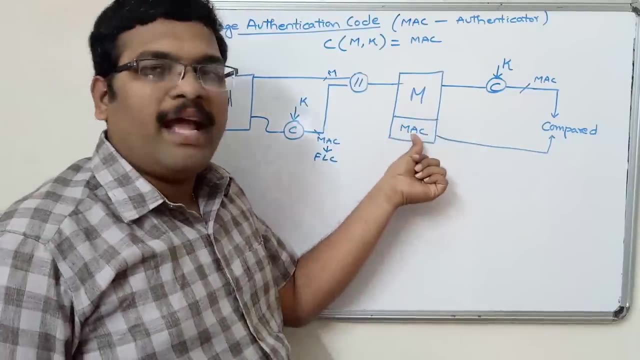 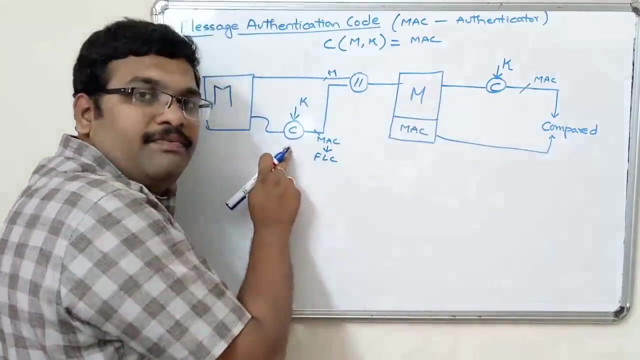 here. this MAC is a fixed length code, fixed length code. so append this fixed length code with the plaintext message so that plaintext message and MAC and send to the receiver at the receiver side again apply the same authentication functions with the same key, so that again we will get the MAC and 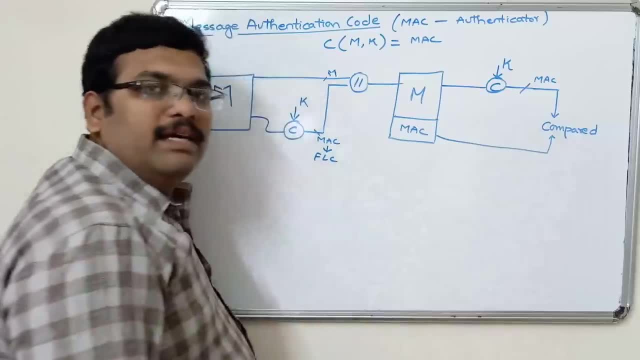 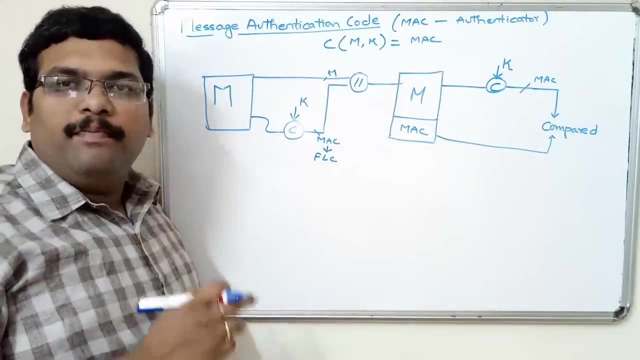 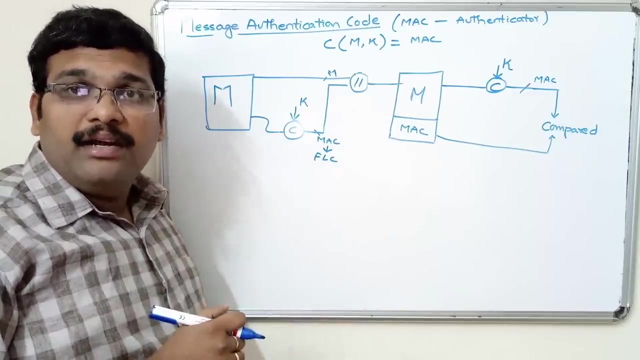 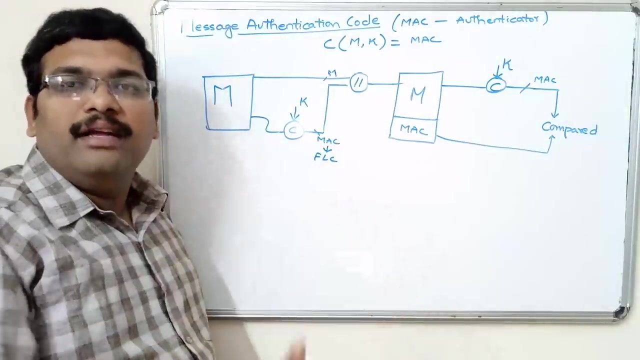 the appended MAC and calculated MAC will be compared. so if both are equal, that implies the sender- the message has been received successfully from the perfect sender- and also integrity. integrity means in between the transmission the data is not modified. so this implies the data is not modified in between the transmission. 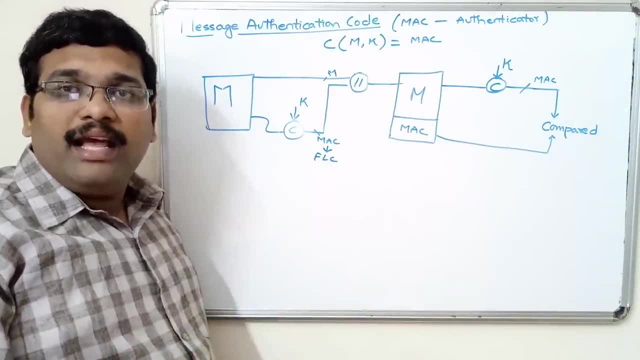 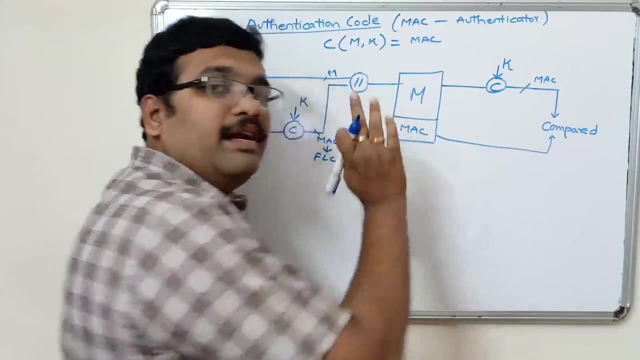 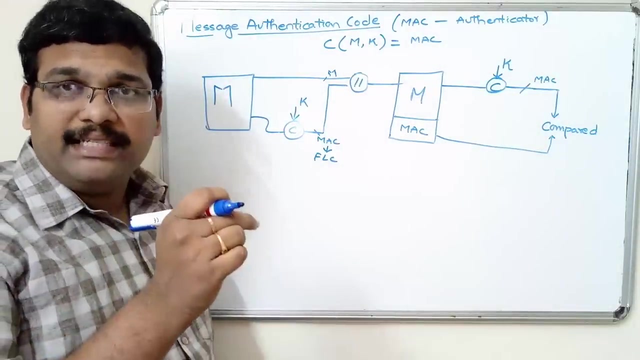 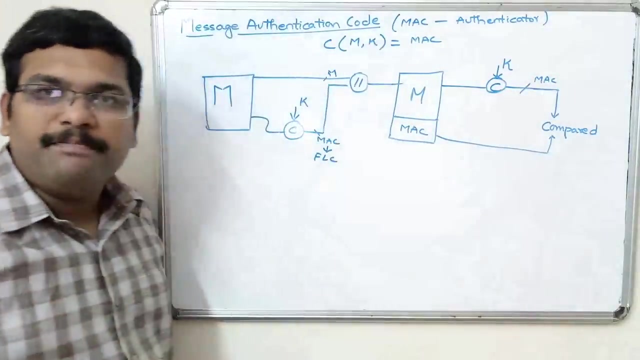 so if the data is modified during the transmission, even change in a single bit will get the difference of this calculated MAC and generated MAC. so this two will not be equal. so if any one bit change in the plaintext message will gives the result of this MAC mismatch. so 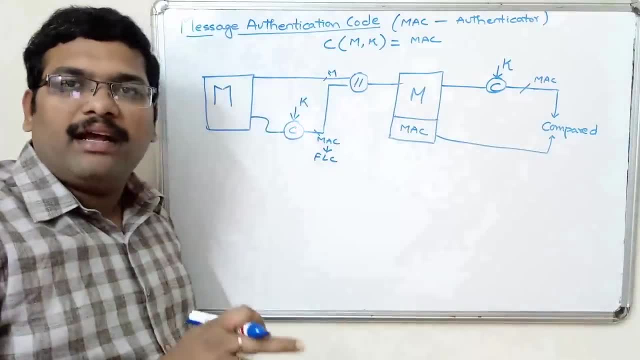 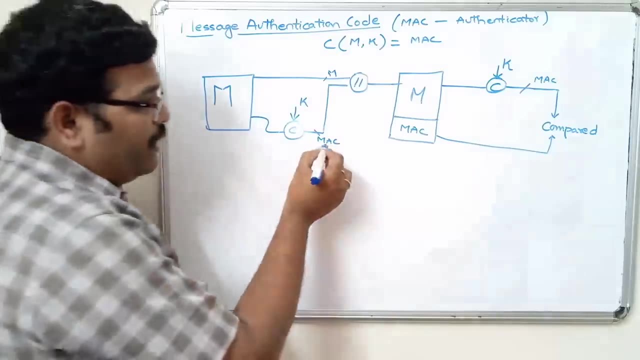 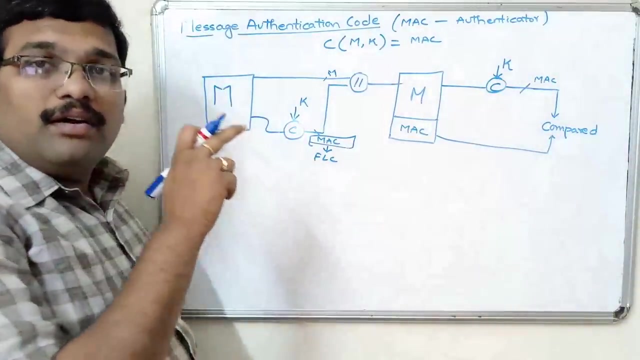 if we get this MAC mismatch, that implies the data is modified or the data is not coming from the perfect sender. so here we are using this MAC, which is called authenticator. so here this MAC is used to authenticate the sender by the receiver, and also vice versa. 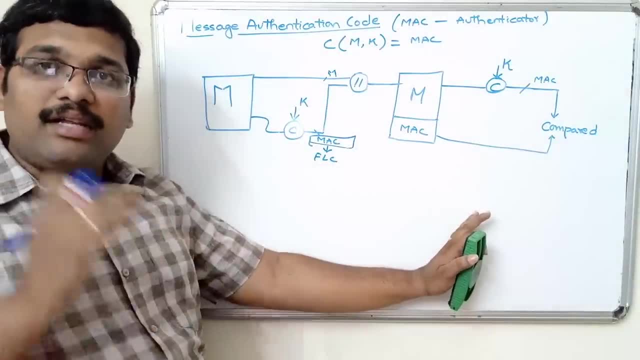 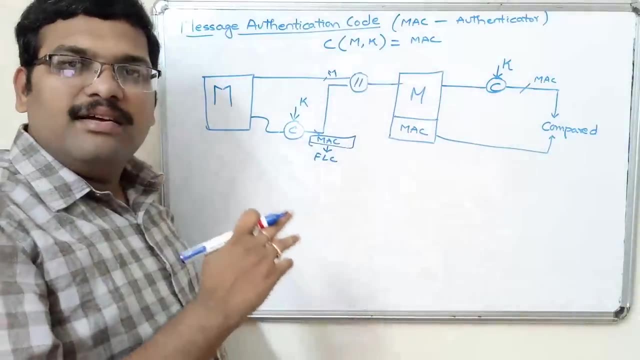 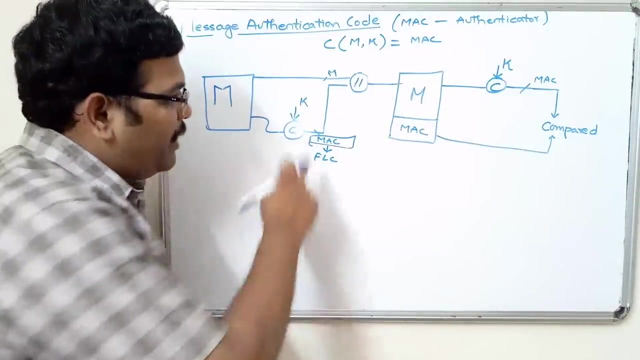 so in this case we have achieved the authentication, but there is no confidentiality, because here the plaintext message is transmitted only in the form of plaintext message. here no encryption has been done. so we are applying the key with the MAC functions, message authentication functions right, so here we are not. 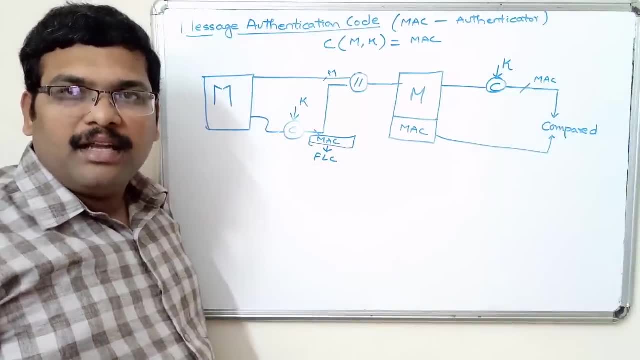 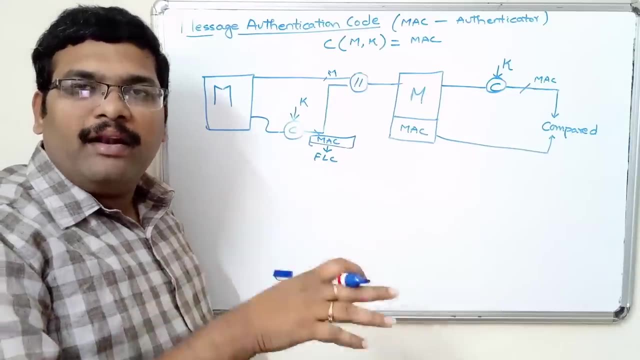 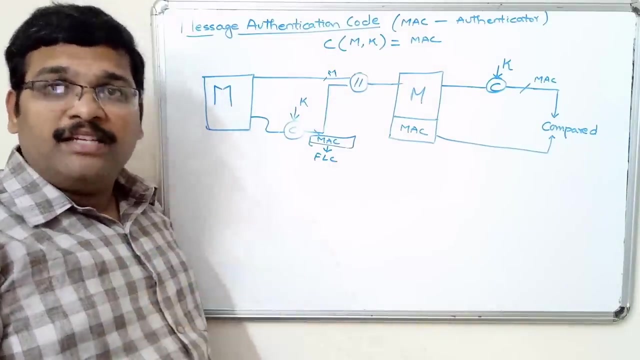 performing any encryption process. so that means the transmission. the bits will be in the plaintext format, so there might be a chance that any one can modify the message during the transmission. so there is no security for the data, so there might be a chance to change the MAC also. 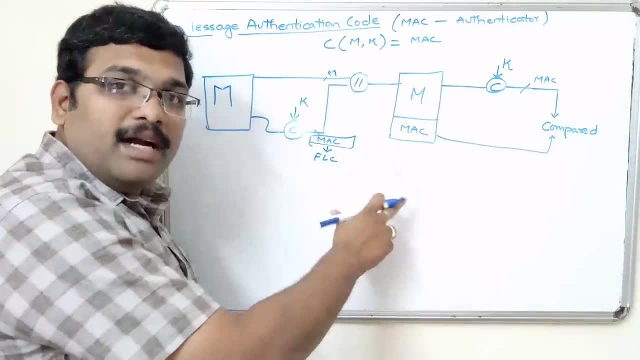 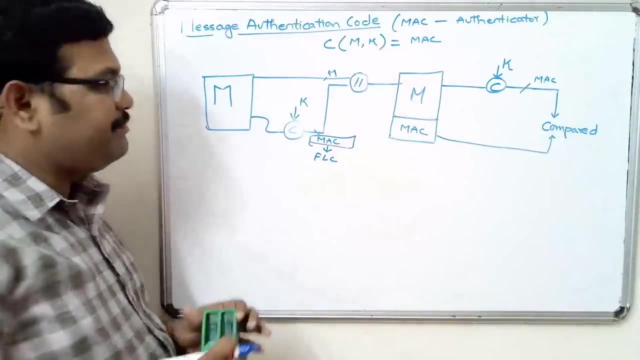 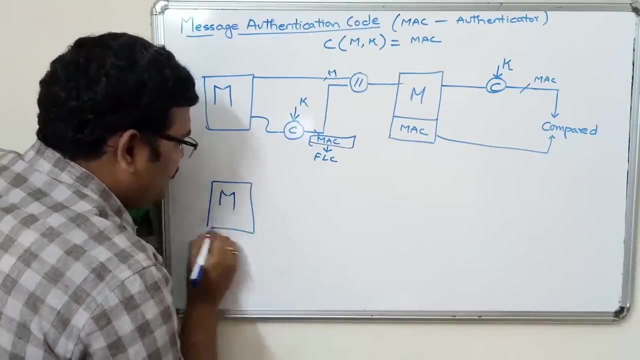 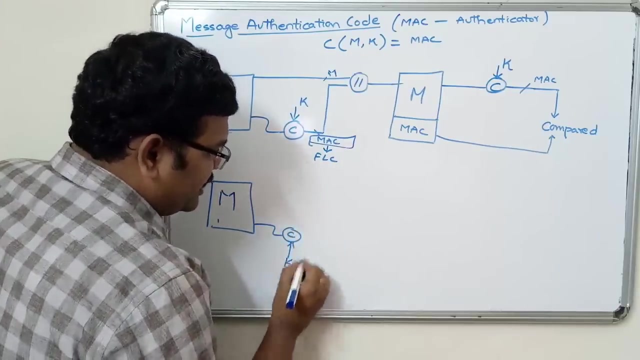 so that means authentication is achieved but there is no confidentiality. so for that we will just add the confidentiality to the MAC, so that we will just add the confidentiality to the MAC and apply the same functions. K is applied so that we will get the MAC and append this MAC. 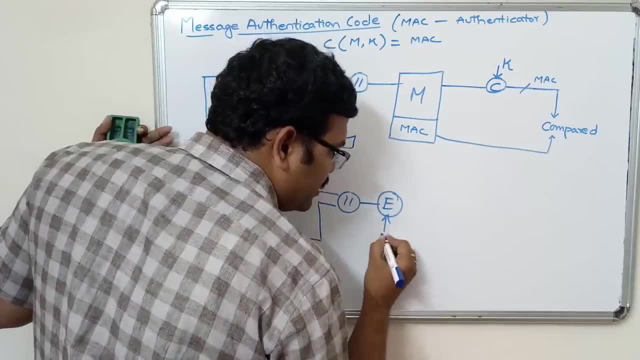 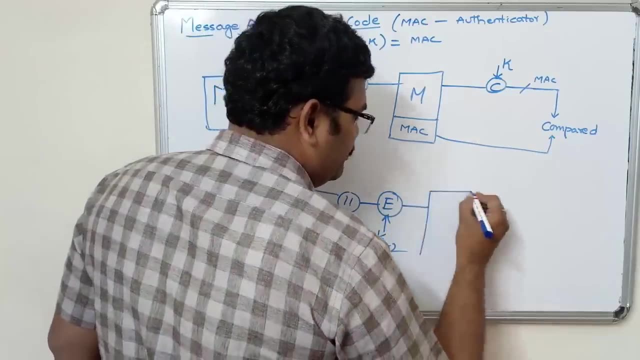 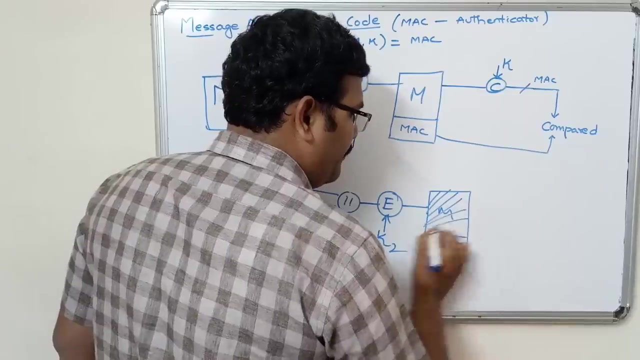 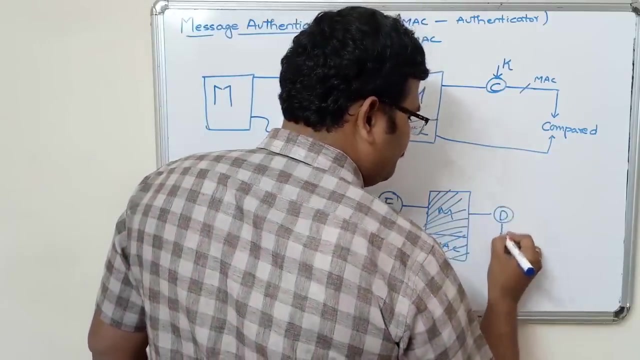 and apply the encryption process, use the symmetric key, so here the K1 and K2, and send to the so see. so this is the MAC and this is the plaintext which is encrypted using the K2, so that first the decryption process will be done by using the. 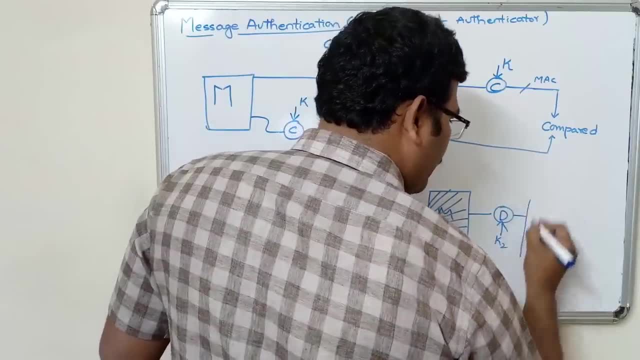 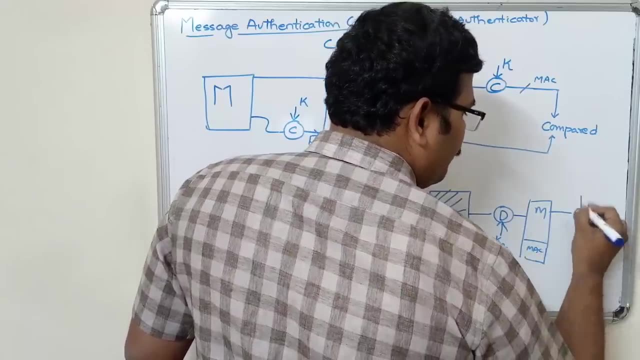 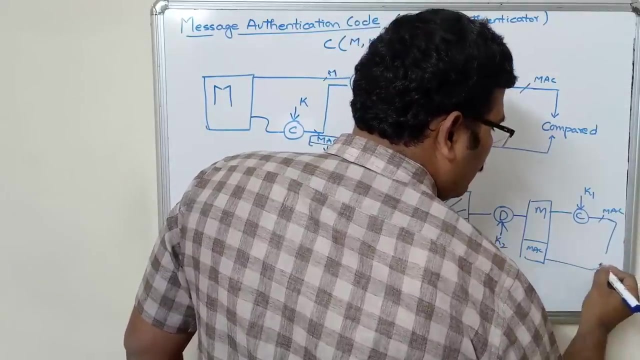 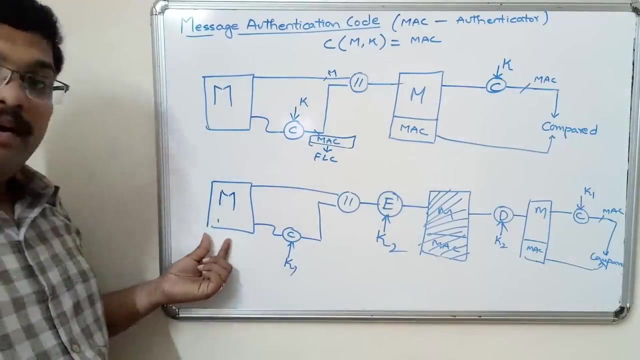 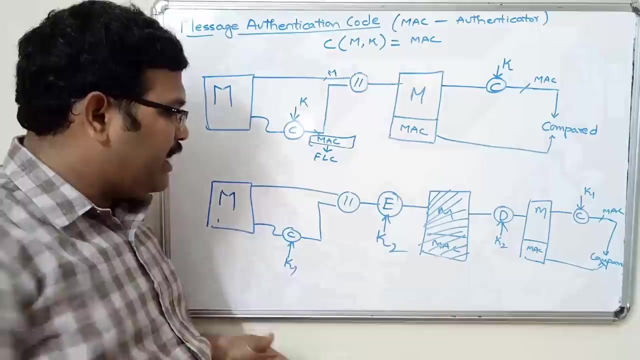 same K2, and then we will get the plaintext message and MAC. now apply the same functions- K1, so that MAC will be generated, and compare this appended MAC. hope you understood. first, control the plaintext message. apply the MAC functions with the along with the K1, so that we will get 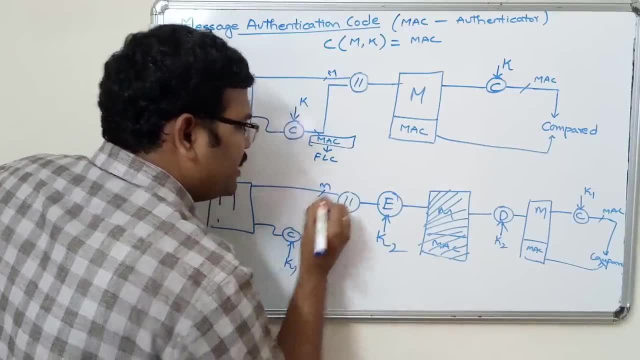 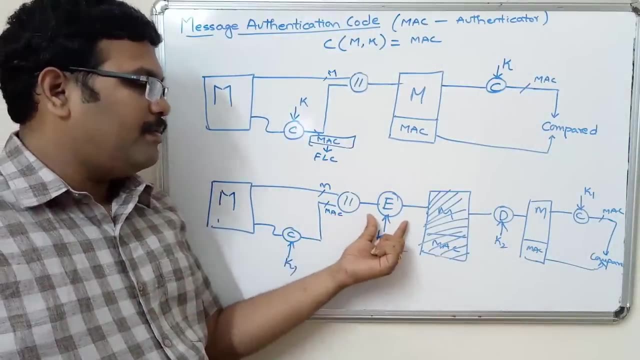 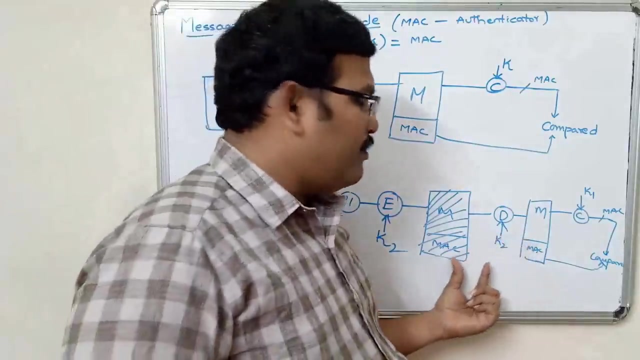 MAC. so this is the MAC and this is the plaintext. so append the message with the plain MAC and encrypt the message with K2 so that we will get the encrypted format and send to the receiver. at the receiver side, first, decrypt this encrypted message using K2 so that we will get 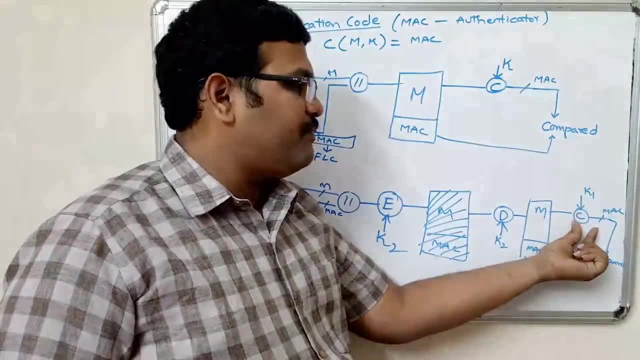 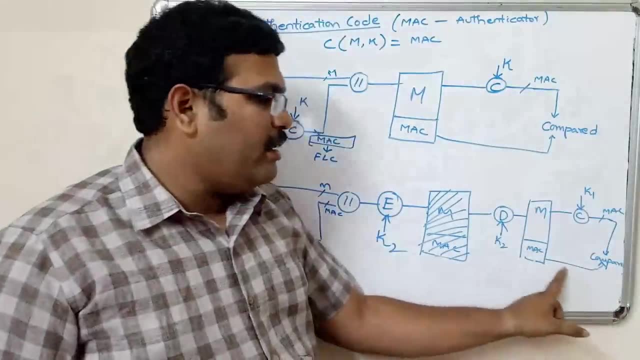 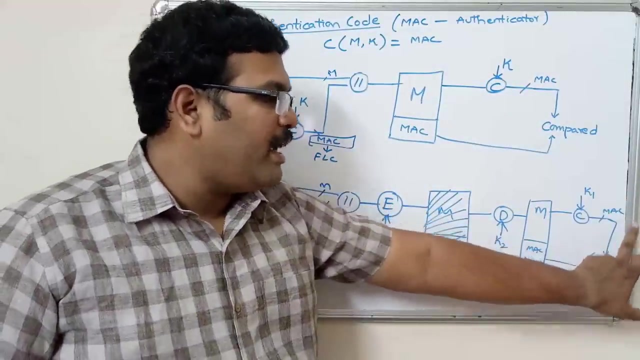 the message and MAC and now apply the message authentication functions along with the key on plaintext message, so that MAC will be generated. now this MAC and the generated MAC will be get compared. so here also same process. so two MACs, that means generated MAC and calculated MAC. I mean calculated. 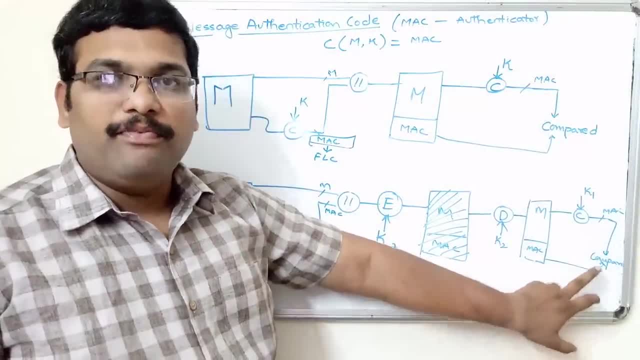 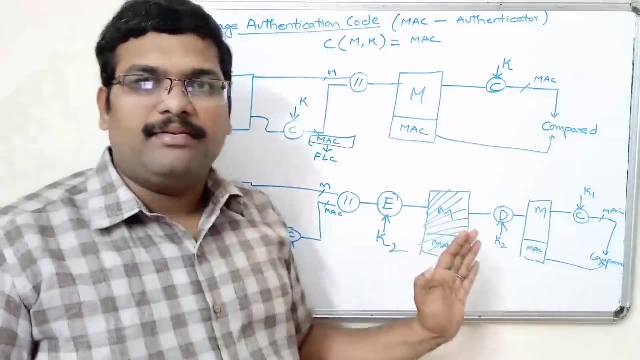 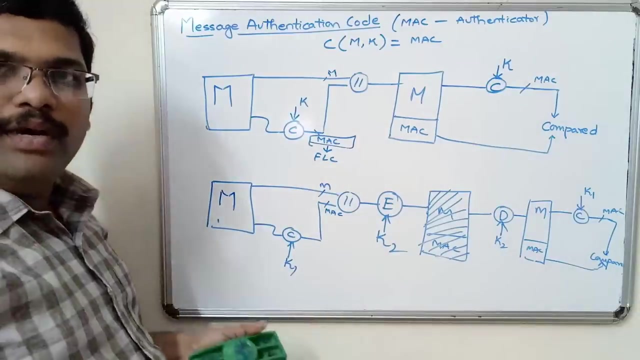 MAC and appended MAC should be equal. so if both are equal, that implies the data is transmitted or sent from the perfect sender. so that means sender is authenticated by the receiver. so there is another form to achieve this authentication. so this is right. so let us see another. 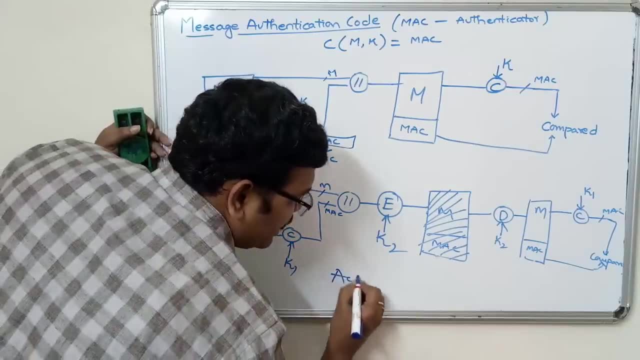 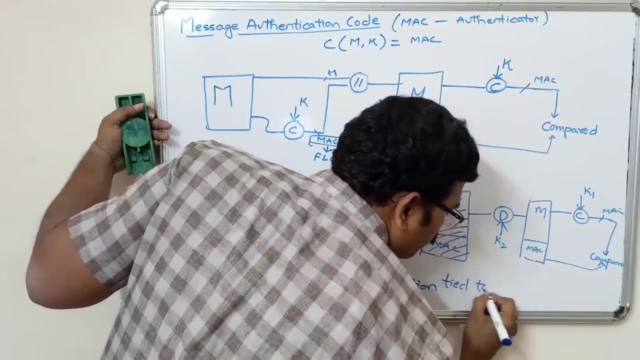 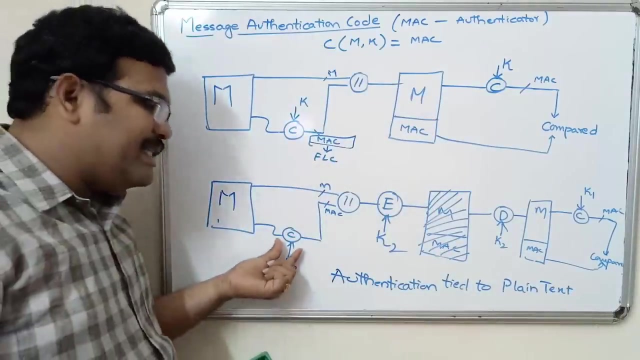 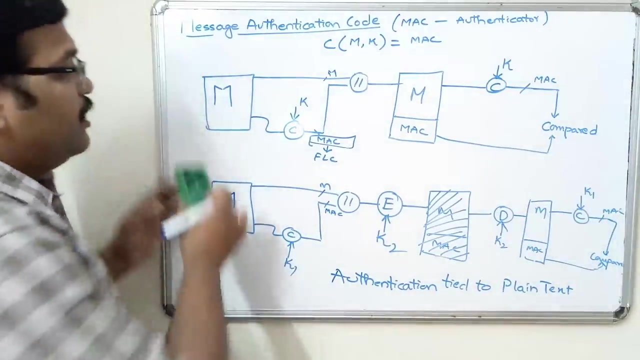 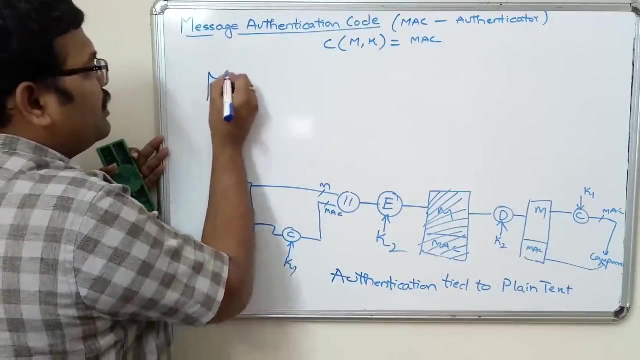 format. so this is authentication tied to plaintext. so authentication tied to plaintext, that means we are applying this. I mean authentication functions on the plaintext, so authentication is tied to plaintext. so if we change this, there is one more format. so first consider the plaintext message. now immediately apply the. 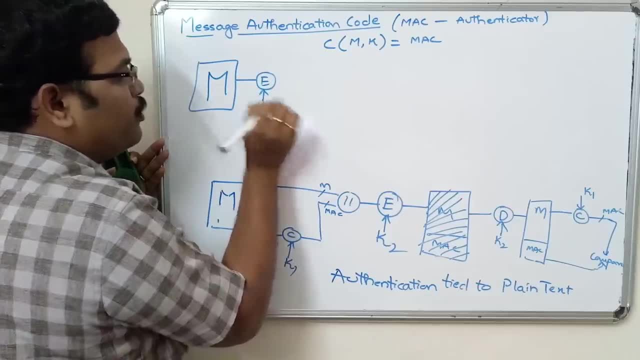 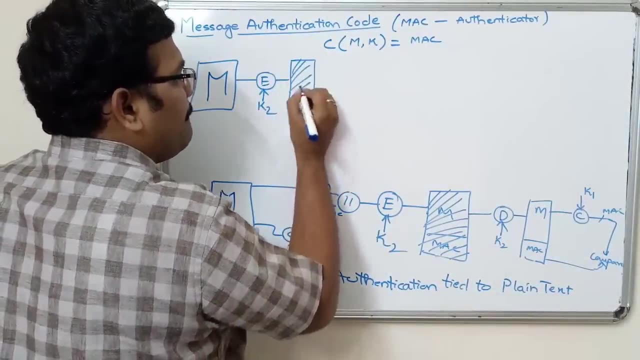 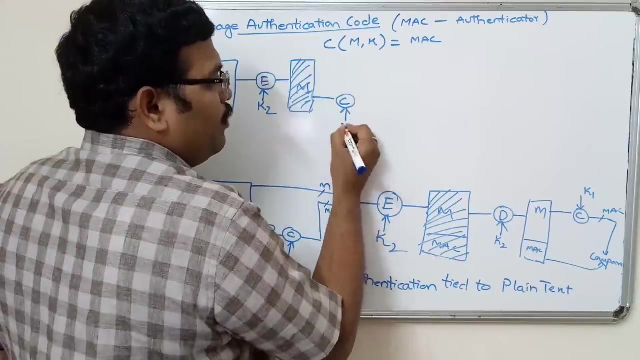 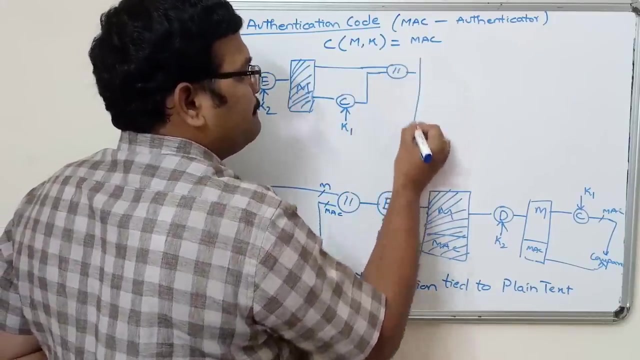 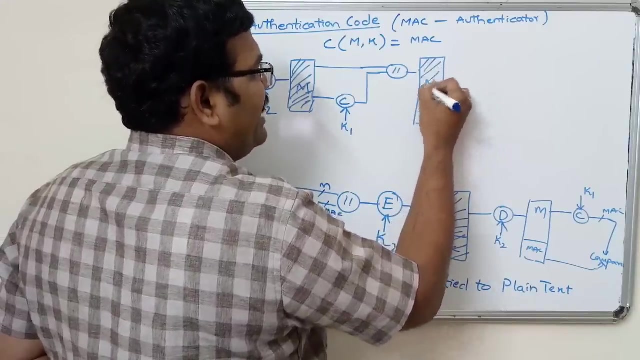 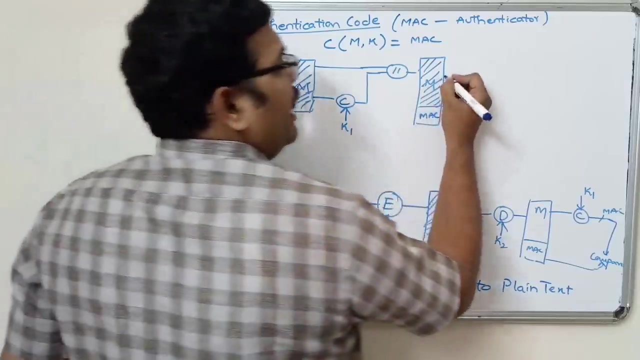 encryption with K2 so that we will get the encrypted message. now apply the functions with K1 and append both. see. so this is the plaintext message which is in an encrypted format and this is the MAC. and at the decryption. so send this to the receiver. so at 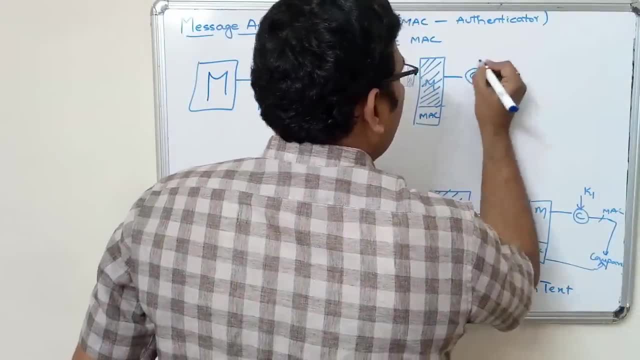 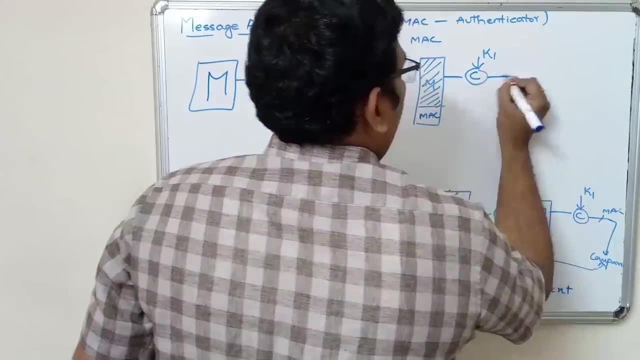 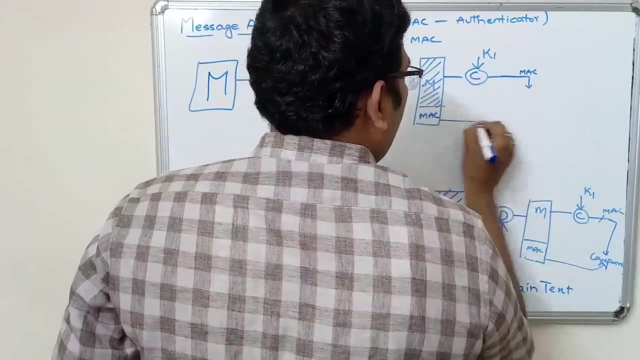 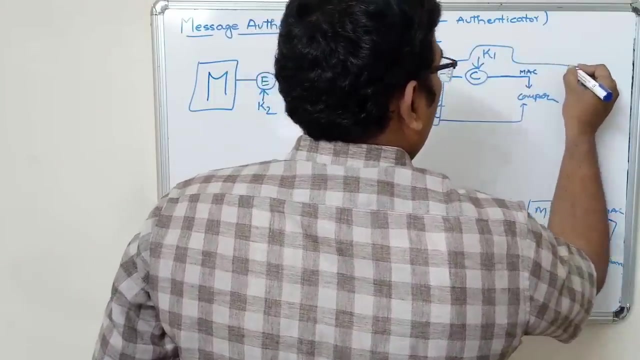 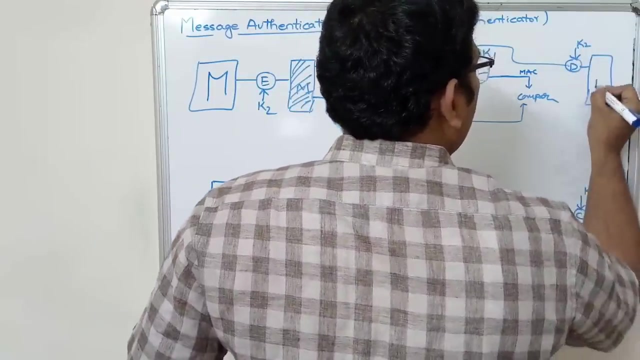 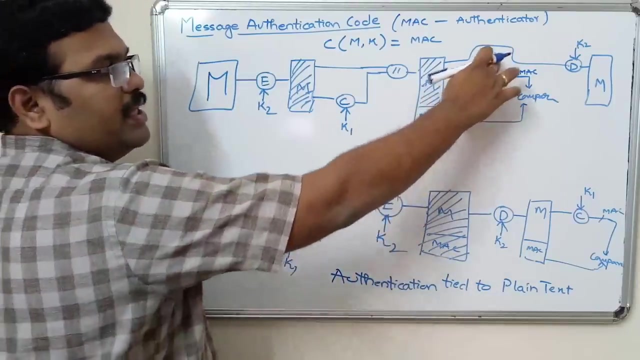 the decryption. first apply the functions using K1, so that we will get the MAC. we will get the MAC and compare, compare. apply the decryption process using K2, so that we will get the plaintext message right. so here, first we have to apply the encryption with K1, so that 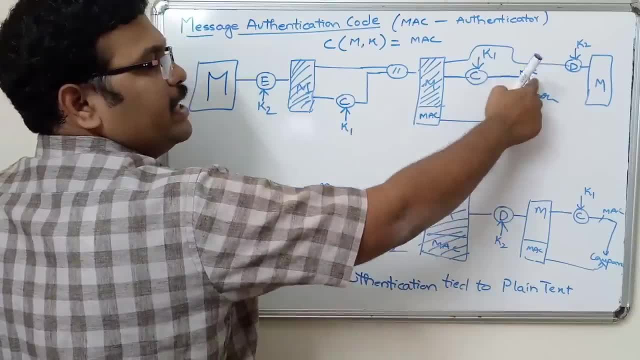 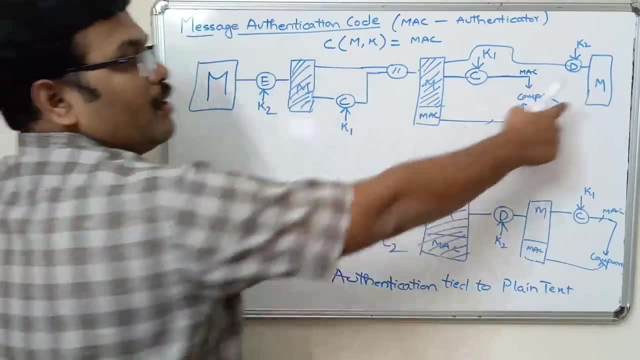 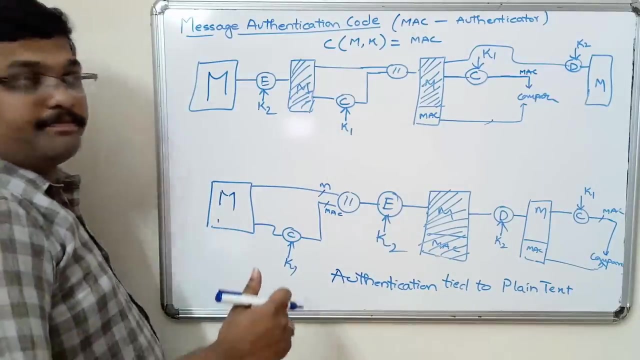 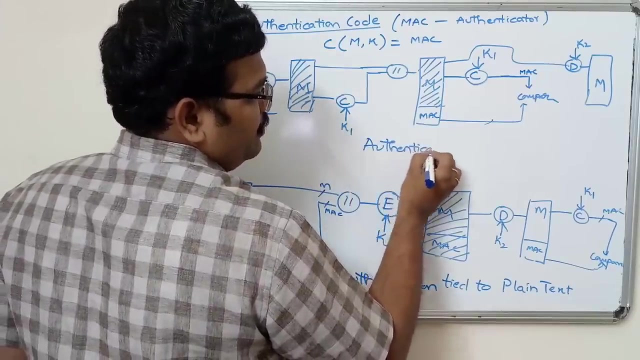 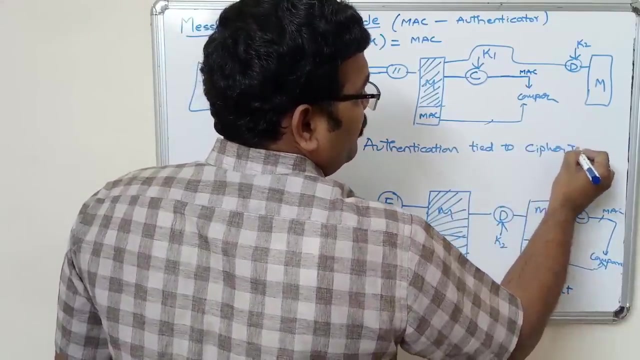 we will get the MAC and appended MAC and this generated MAC will be compared and similarly, the encrypted message will be decrypted by using the K2 so that we will get the plaintext. so this is called authentication tied to ciphertext. so because first we are generating the ciphertext and then applying 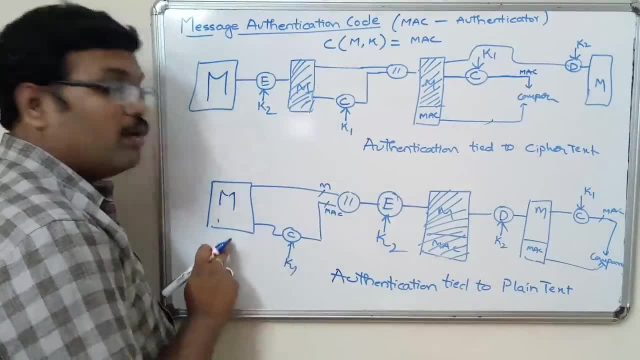 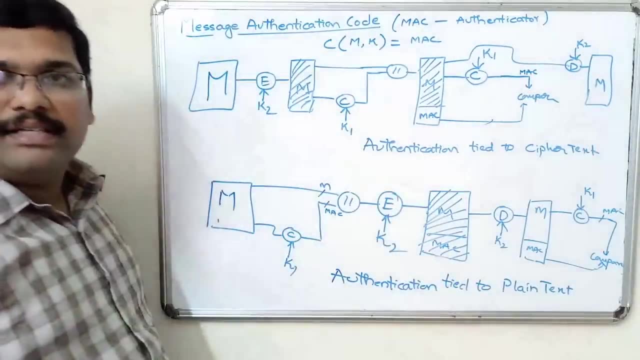 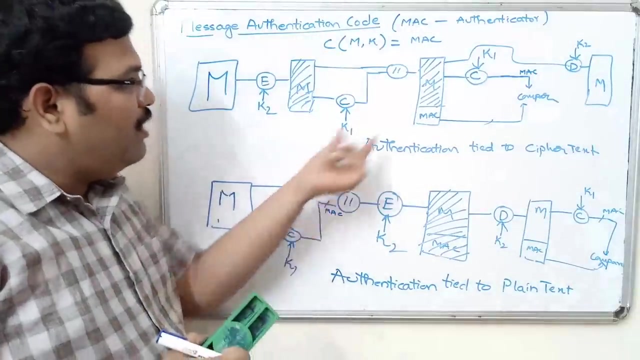 the functions on the ciphertext. here we are applying the functions on the plaintext message. so that's why we call it as authentication tied to plaintext and authentication tied to ciphertext. so this is the second process. so here, first we have to generate the fixed length code by applying 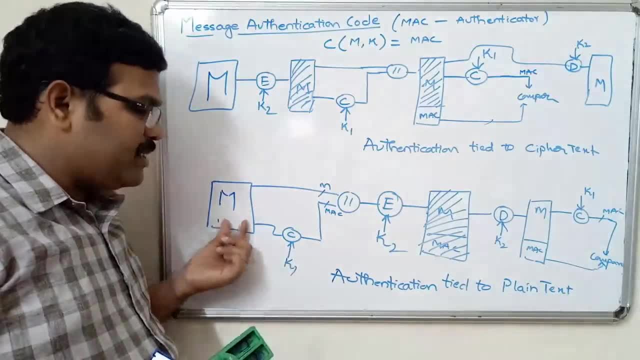 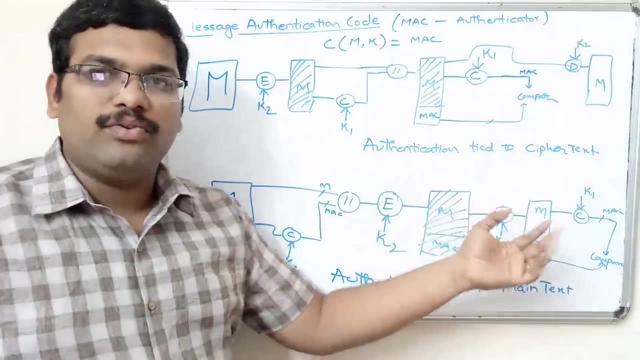 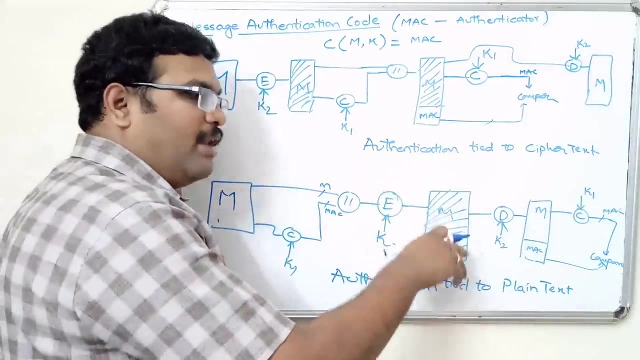 the message functions on the plaintext message along with the key and we have to append that fixed length code with the plaintext message and we have to send that to the receiver at the receiver side again if they will calculate. so at the receiver side the receiver will calculate. or generate the MAC by applying the same functions and the same key on the plaintext message, and the generated MAC and the appended MAC will be get compared. so if both the MACs are equal, that implies the data is sent by the perfect sender. that means sender is authenticated. 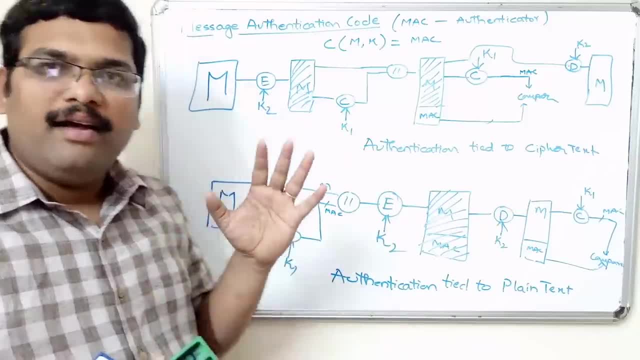 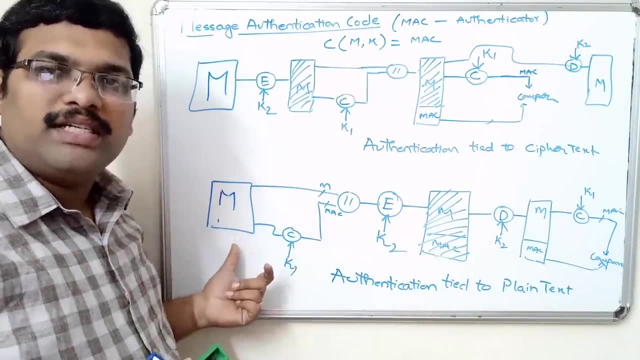 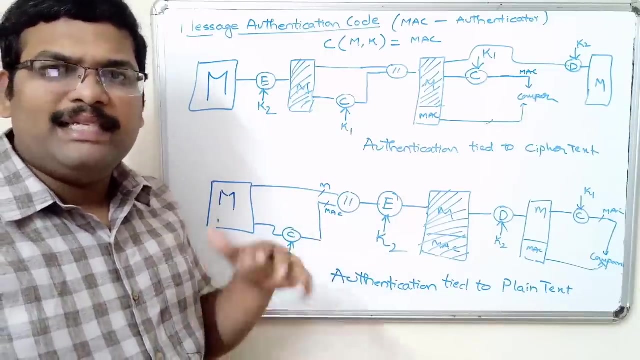 if the message- i mean both the MACs- are unequal or not equal, that implies the data is modified or the data is not sent by the authorizer. sender: authenticated sender. so hope you understood the second one and similarly the third one, that is, hash functions. let's move on to the hash functions. 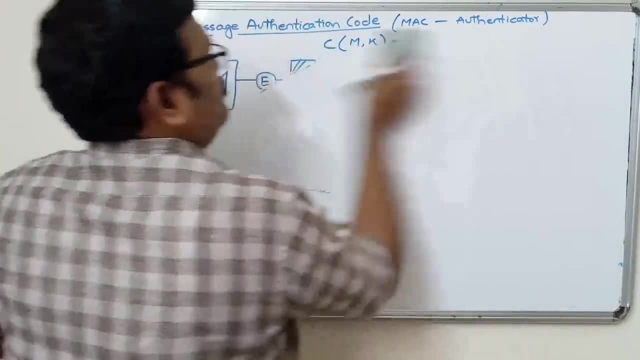 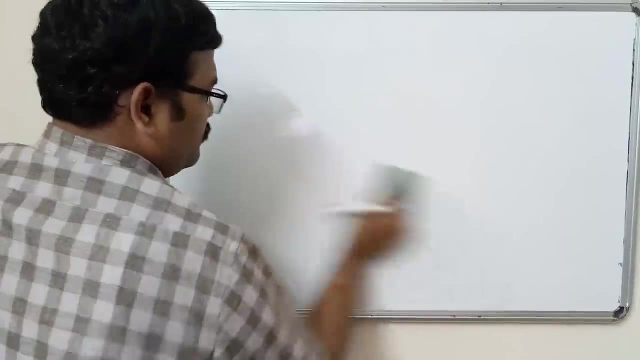 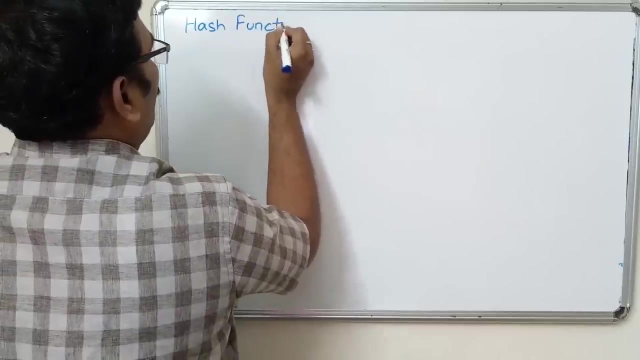 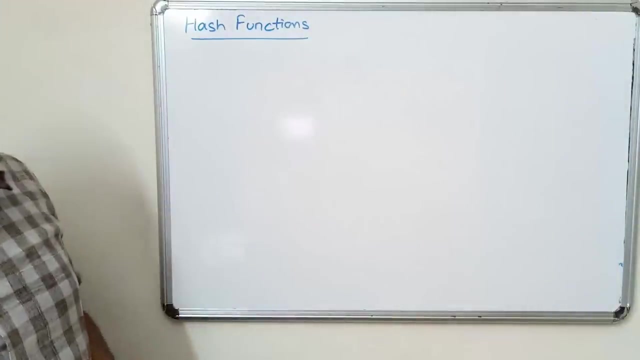 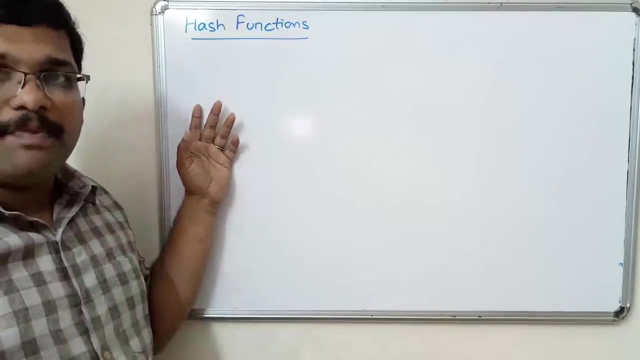 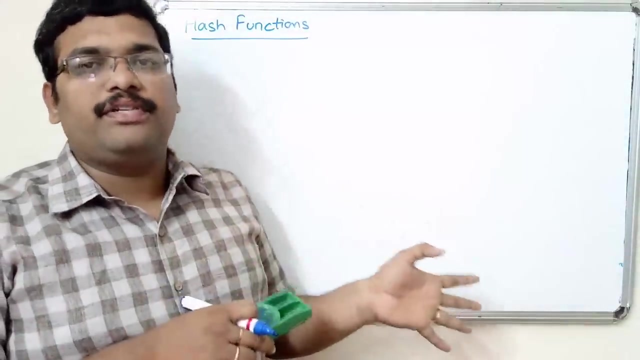 the third process, hash functions. so in this hash function, in this hash function, here also there is a separate authenticator. that is, first we have to generate the fixed length code and then we have to use those fixed length code for this authentication process. so that fixed length code, we call it as hash code. 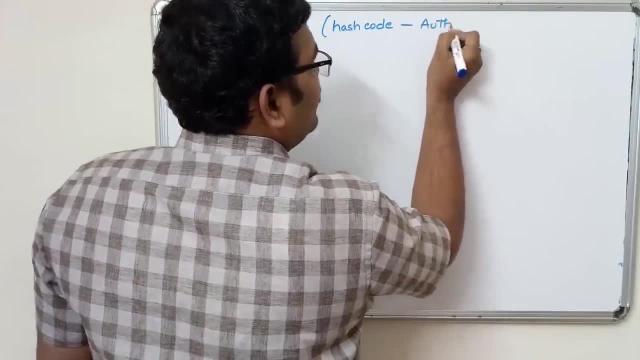 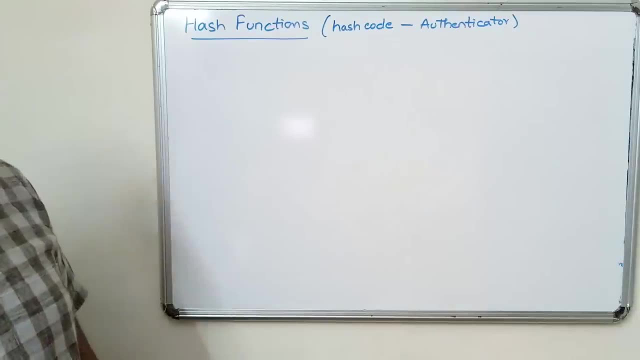 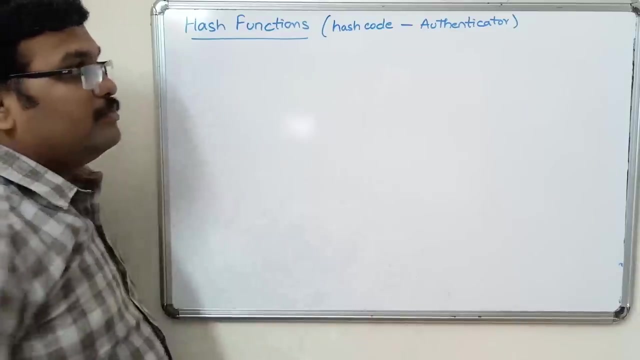 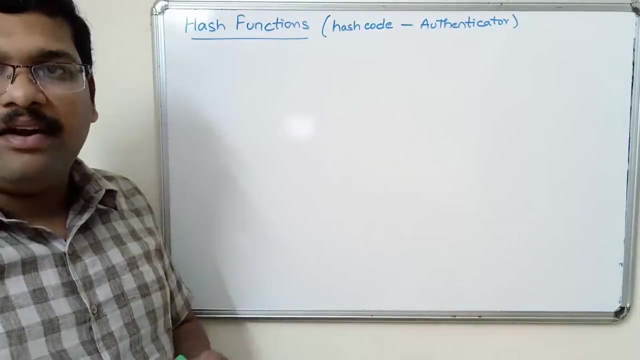 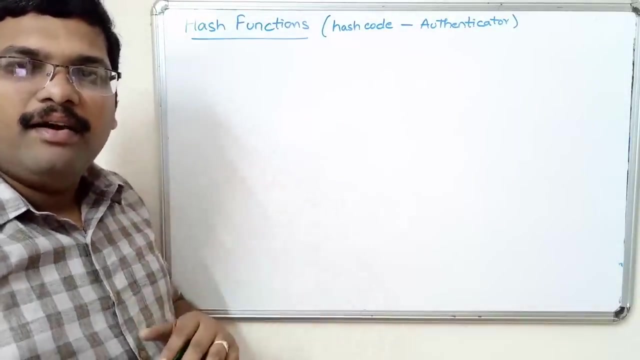 hash code which acts as an authenticator. hash code which acts as an authenticator. so here, let us see here the difference between this. hash functions and message authentication code is independent of key. so in the MAC we are using the message authentication functions along with the key, and here we will. 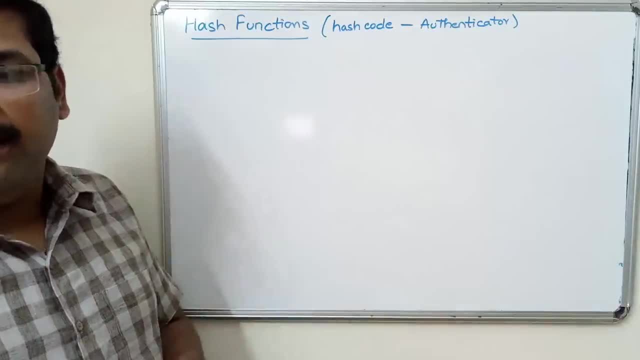 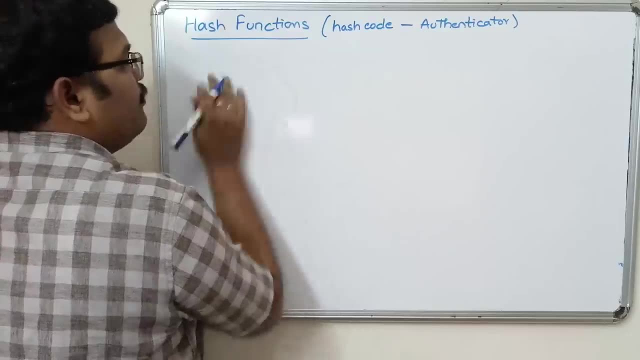 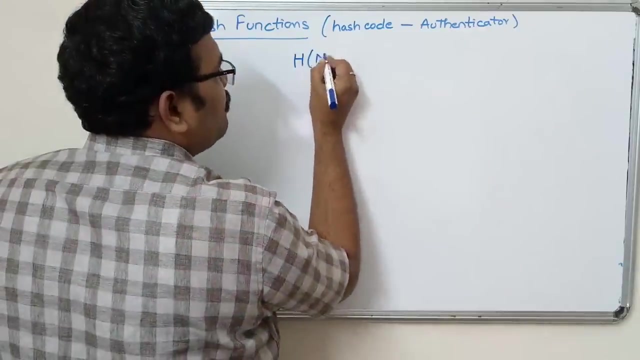 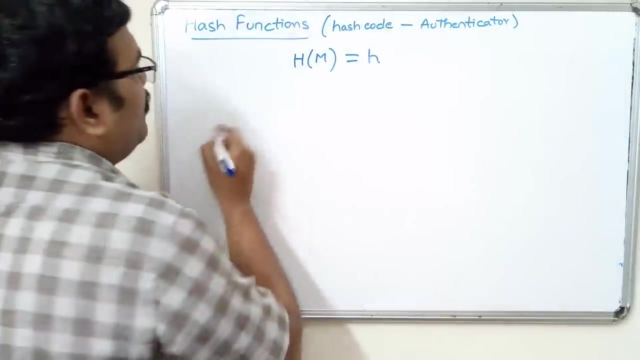 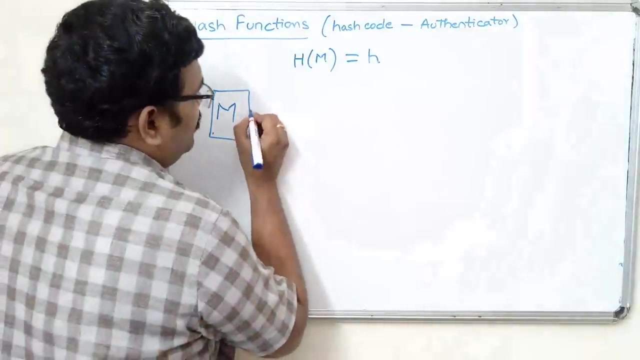 use only the hash functions without any key. so let us apply so before that. so let us see capital. H means hash functions. applied on plain text message will produce fixed length code which is called H is a hash code. now consider this plain text message. similarly, apply the. 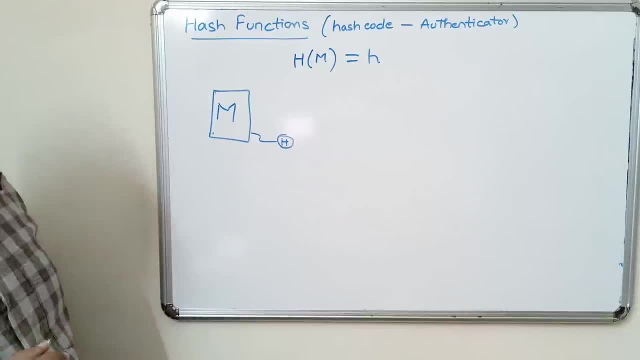 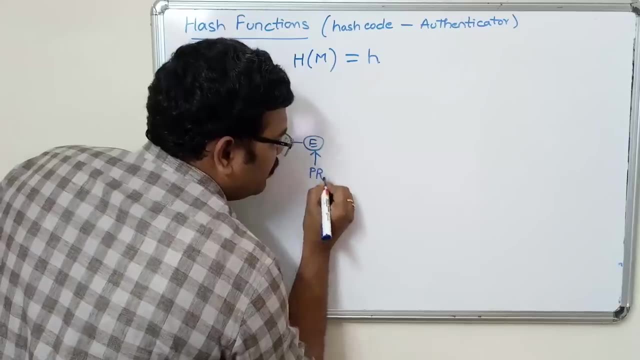 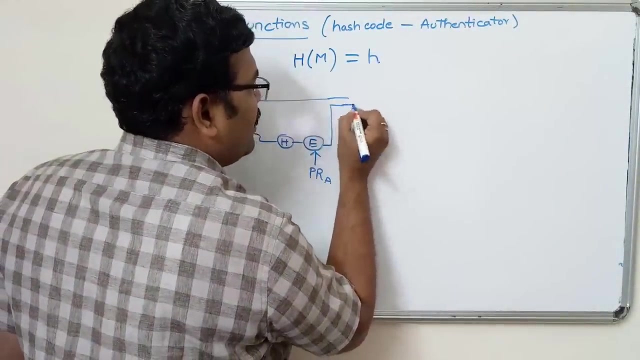 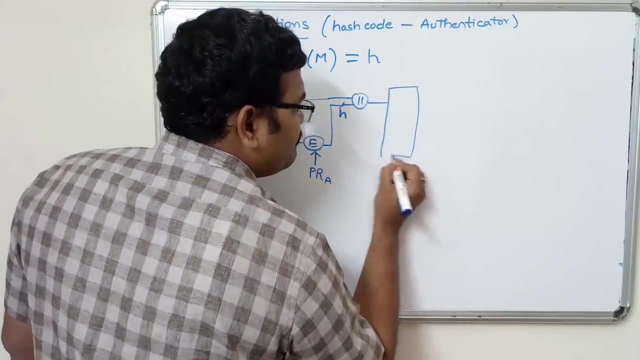 hash functions. apply the hash functions. similarly, apply the hash functions. next, encrypt this hash function by using PNA. by using PNA, so encrypted MAC, I mean hash code. encrypted hash code will be appended to the plain text message. appended to the plain text message, so H. so here H is a hash code. 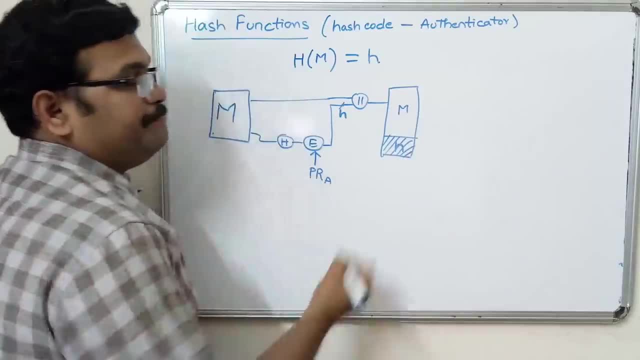 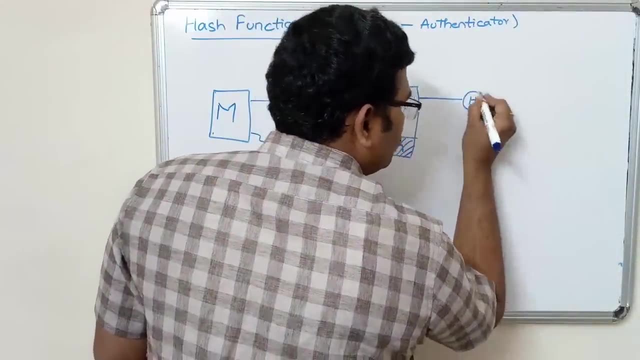 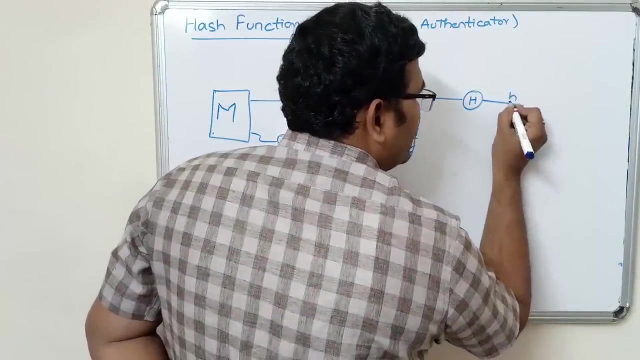 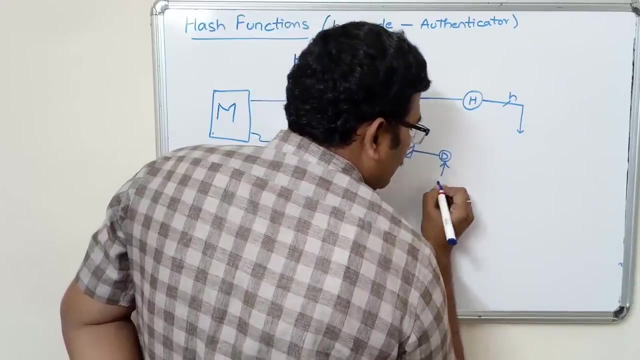 this is a plain text message. this will be sent to the receiver. so at the receiver side again, apply the hash functions. so here we are not using any key. apply the hash function so that again we will get hash code. so decrypt this one by using public key. 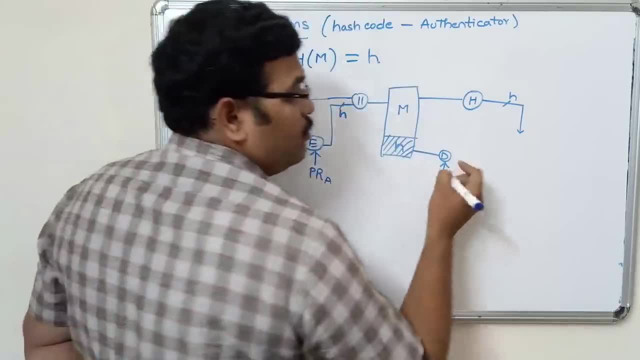 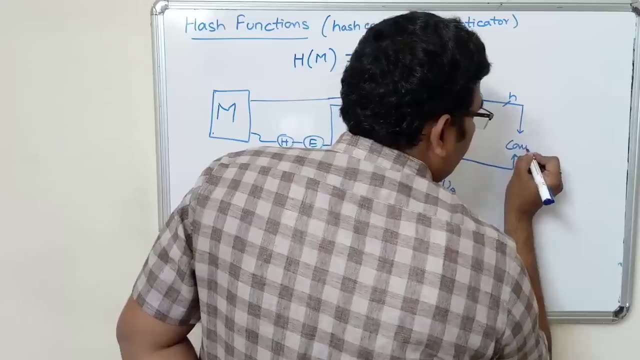 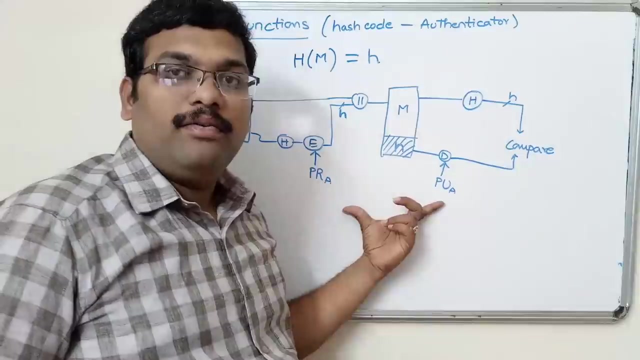 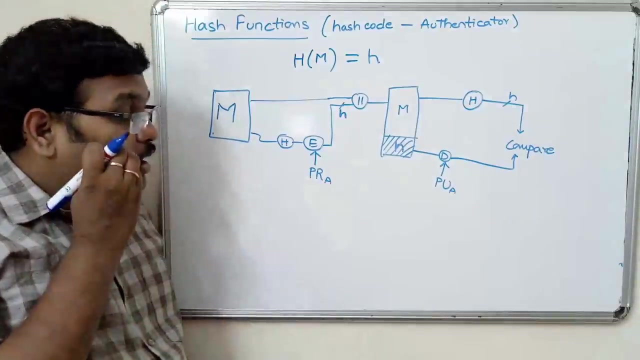 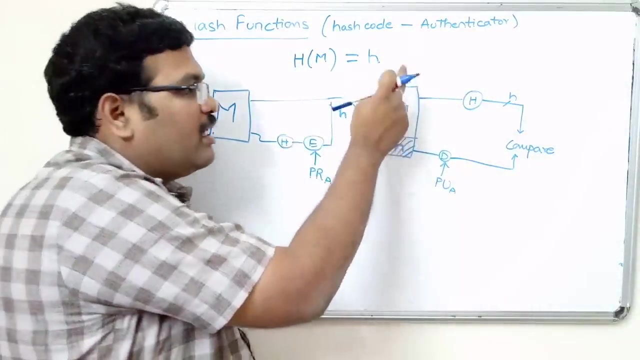 of A, which is available with all the users, and then compare with the generated hash code. so this is the one way we use this hash function. so there is a drawback of in this case, because here we are applying encryption to the hash code but not to the plain text message. here 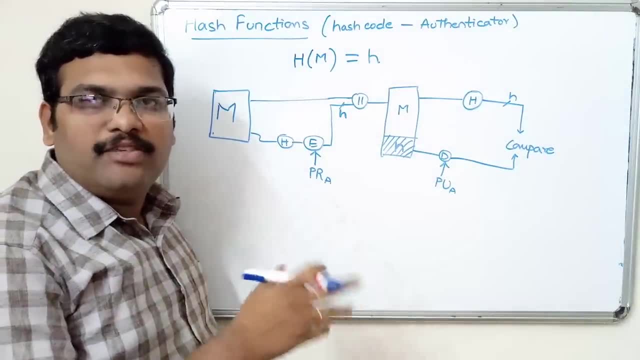 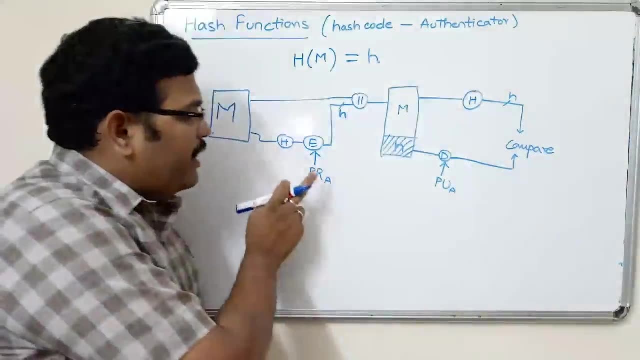 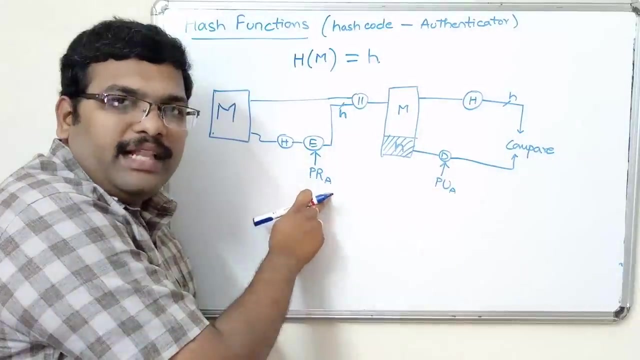 the bits will be transmitted only in the form of plain text, so there is a chance to modify to the plain text. and the second one is here. we are applying encryption. we are performing the encryption on the hash code using the private key of A. that means sender is perfect and 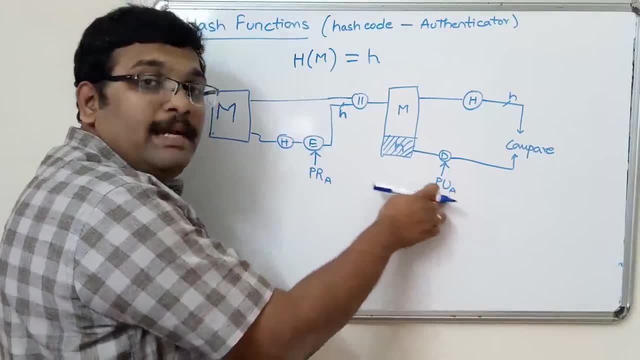 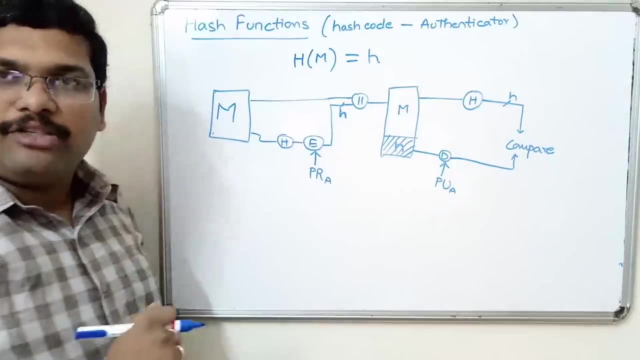 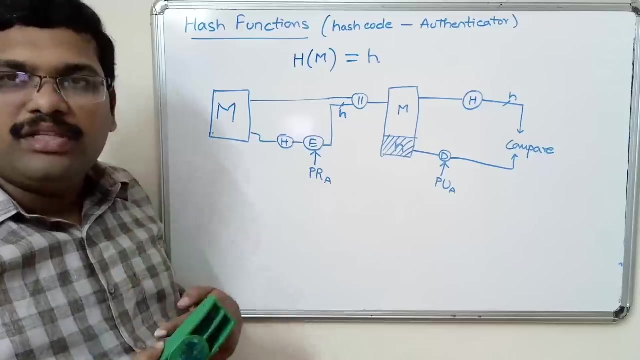 at the receiver side. we have to decrypt the same by using public key of A, which is available with all the users in the network, so anyone can decrypt this hash code. so that is the drawback in this case. so in order to avoid this again, we have to use the. 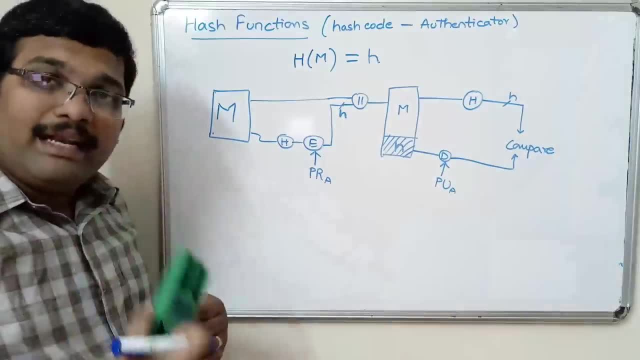 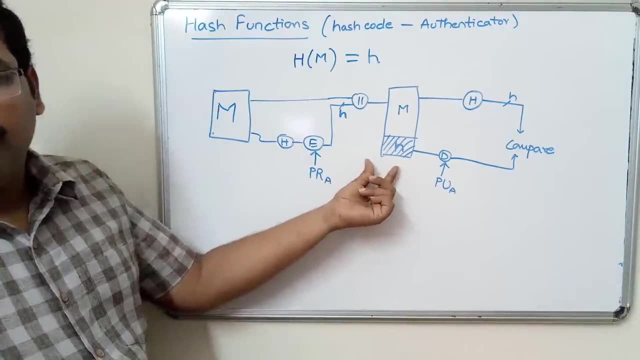 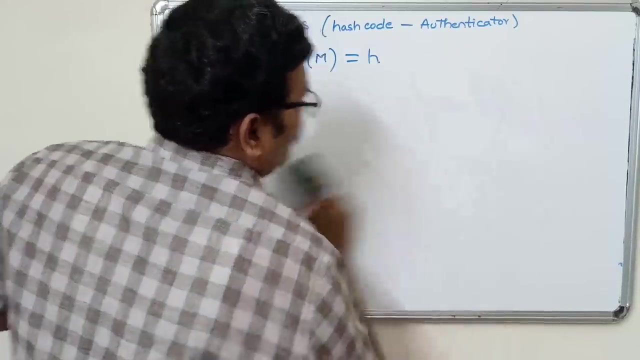 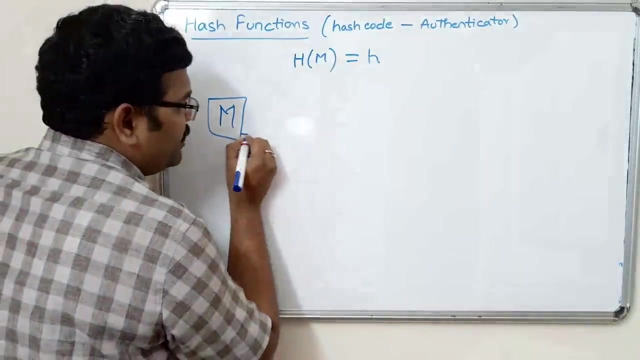 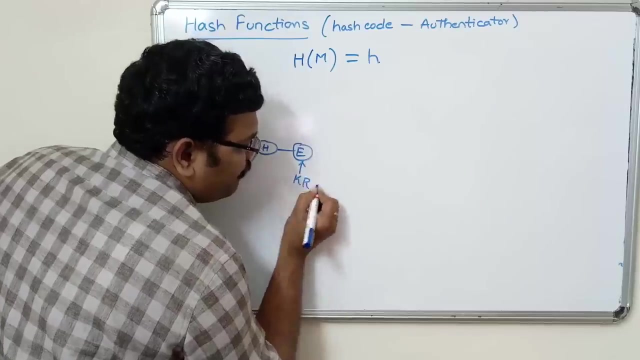 encryption. I mean we have to perform the encryption algorithm on this plain text message and the encrypted hash code. so let us see that. so first, apply the plain text message, consider the plain text message, apply the hash code and apply the encryption process by using private key, so that 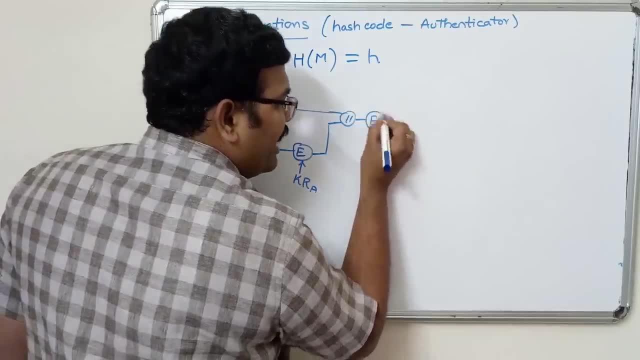 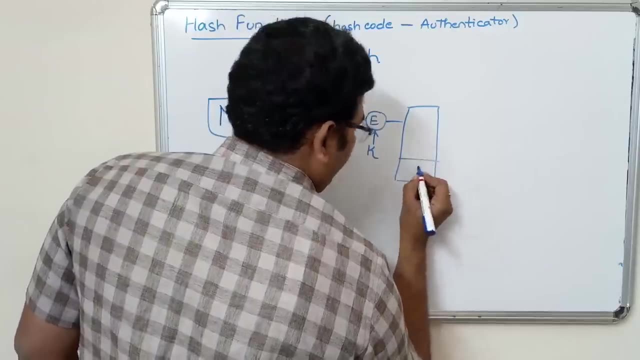 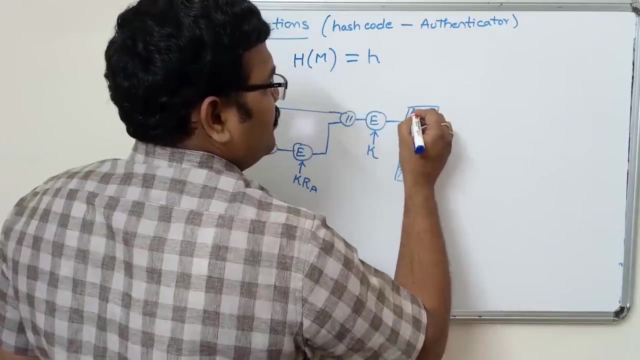 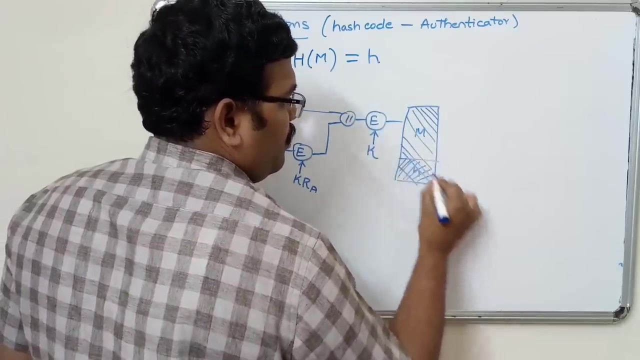 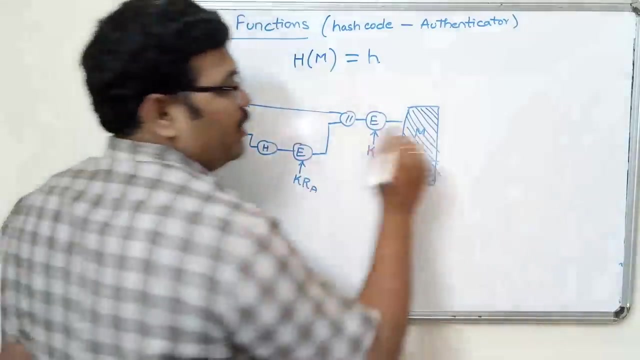 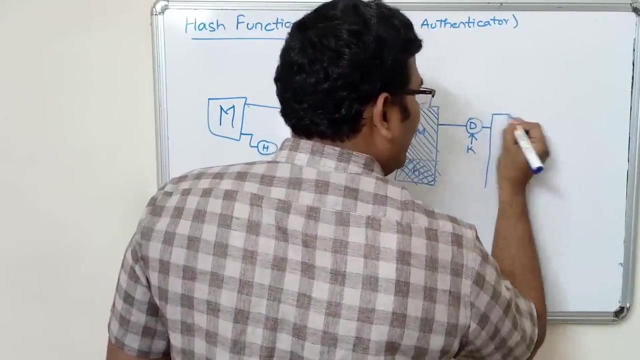 appended and again encrypt this using the secret key. now the message will be hash code, plain text message. so this is the encrypted format now. first we have to perform the decryption by using the secret key so that we will get the plain text message and encrypted hash code. 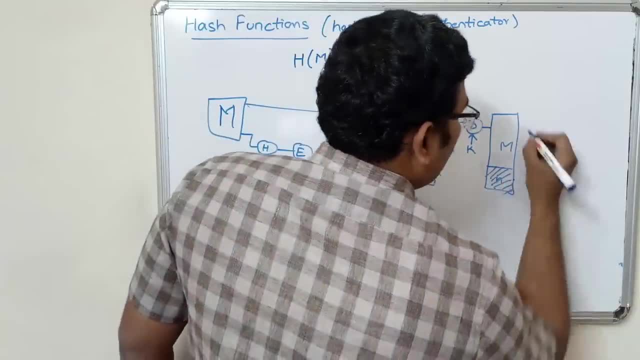 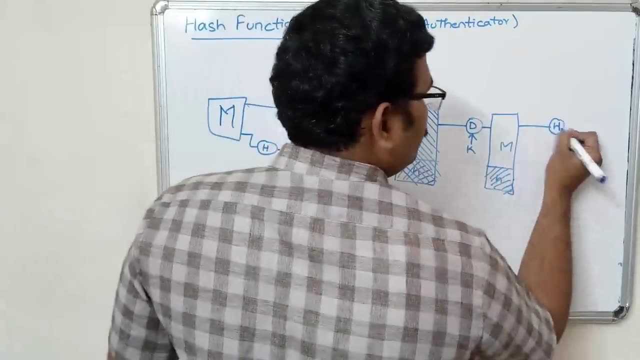 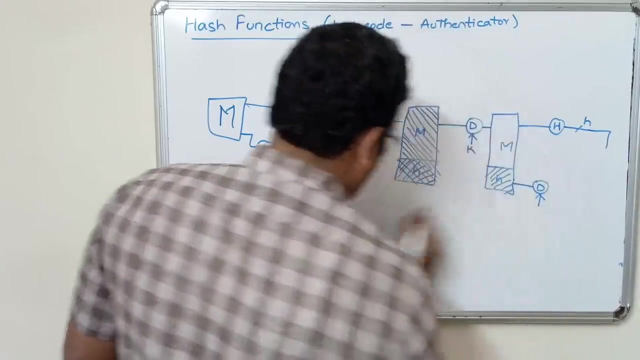 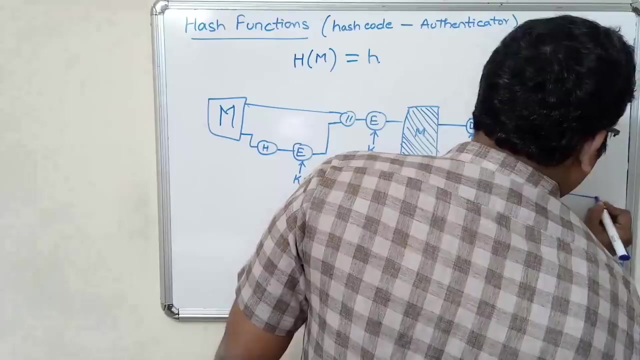 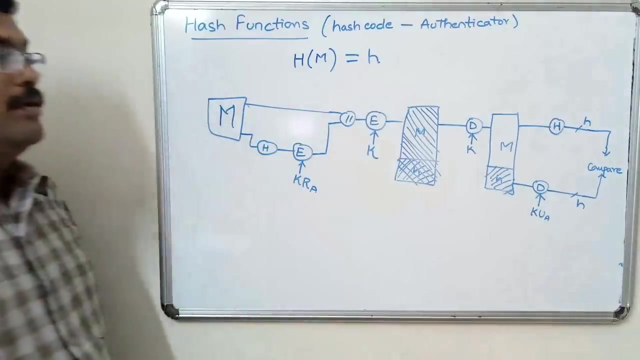 where again we have to apply the hash function. sorry, apply the hash code so that we will get hash code and decrypt this using public key of A, so that we will again get the hash code which is to be compared with the calculated hash code. so this is the process. 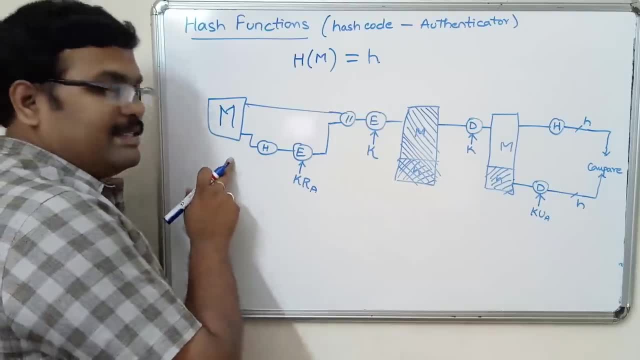 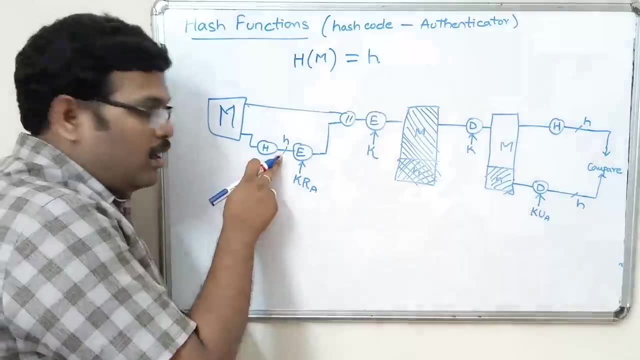 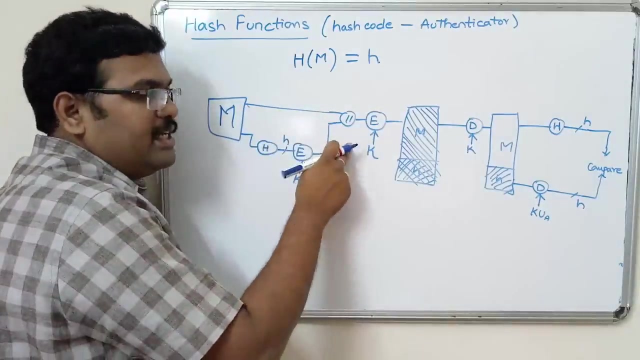 right. so in the sender side, first we are applying the hash function and here we will getting the hash code. we are getting the hash code and encrypting: encrypt the hash code by using the private key of A and then appended with the plain text message and the complete message. 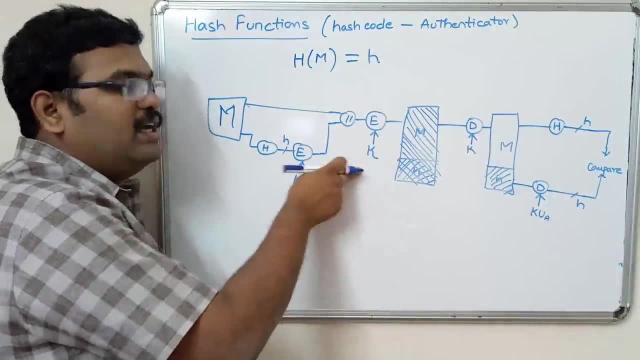 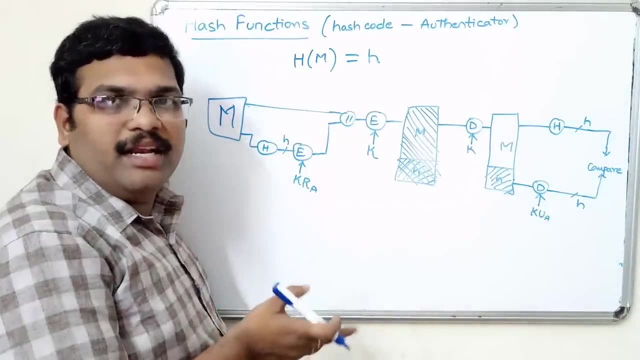 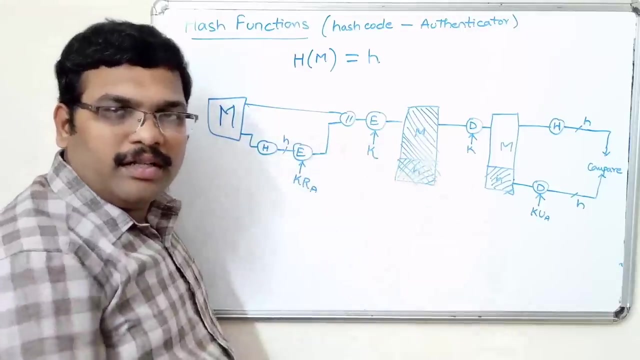 with the encrypted hash code will be encrypted by using the secret key. so again, here we are using the symmetrical encryption. so this is the combination of both the symmetric and asymmetric encryption. so by combining these, both symmetric and asymmetric encryption, we will achieve the authentication. so here we are using. 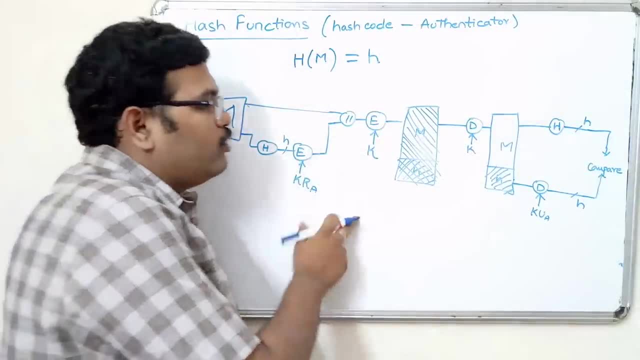 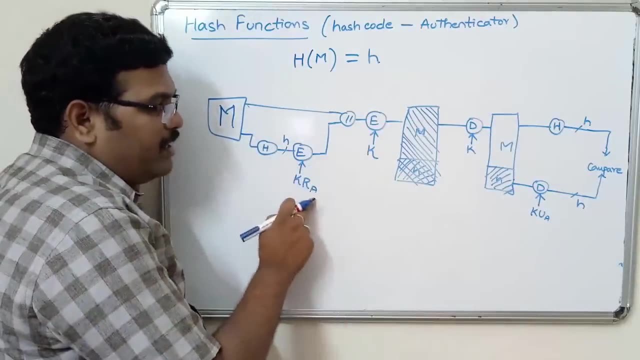 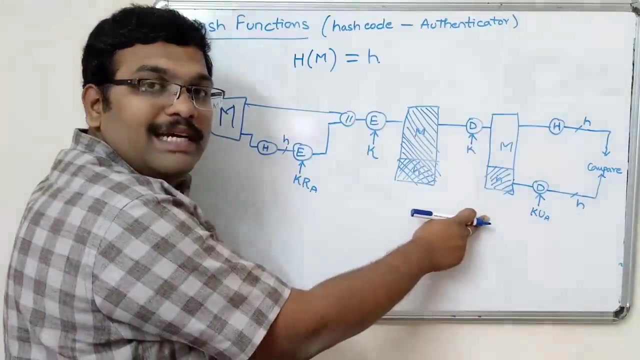 the public key encryption only on the hash code and we are using the symmetrical encryption on the plain text message. so, after applying the private key on the hash code appended with the plain text message and encrypt that with the secret key so that it will be sent to the receiver and at the receiver, 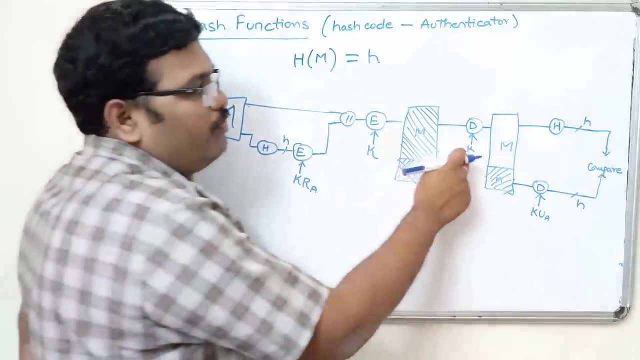 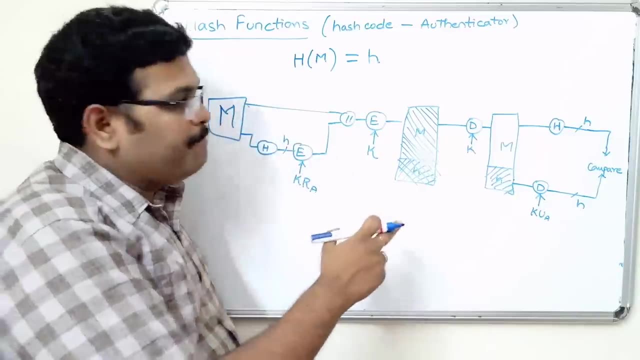 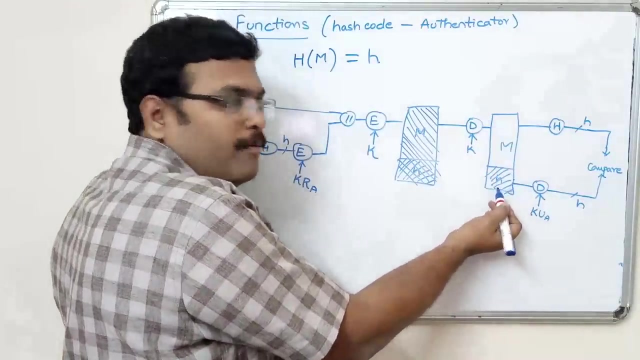 first decrypt this complete encrypted message with the secret key, so which is shared between only sender and receiver, so that only the receiver can decrypt the message. so after this description, decryption, we will get the plain text message along with the encrypted hash code, and this hash code is encrypted by using the private key of user here, so it 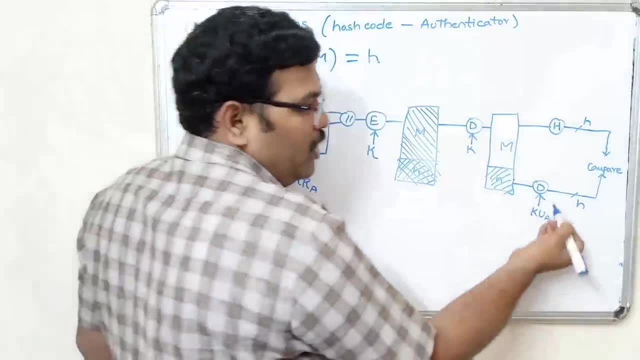 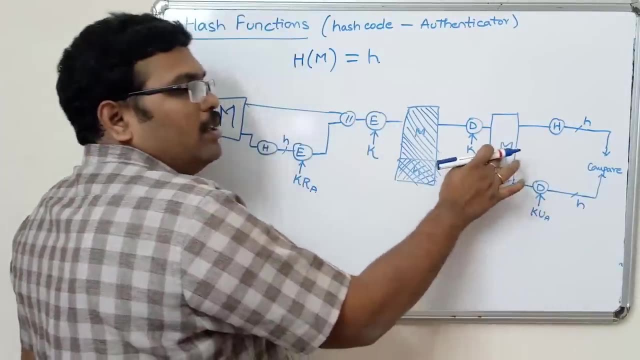 must be decrypted by using public key of user year. so we can decrypt this message by using public key of user here so that we will get the hash code. now on on the plain text message: apply the same hash functions. apply the same hash function so that we will again get the 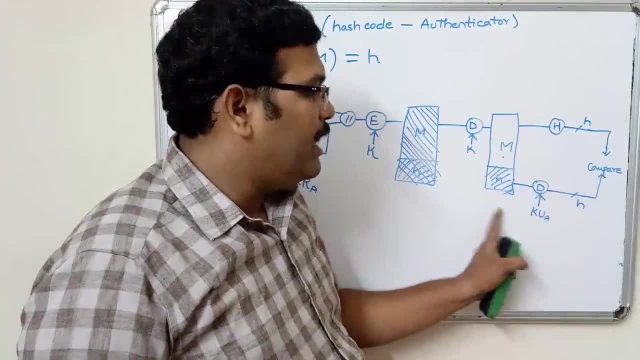 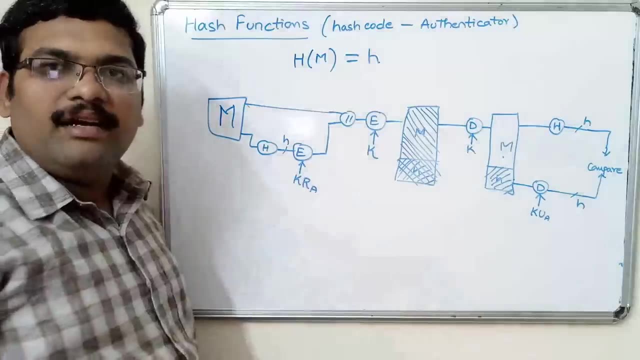 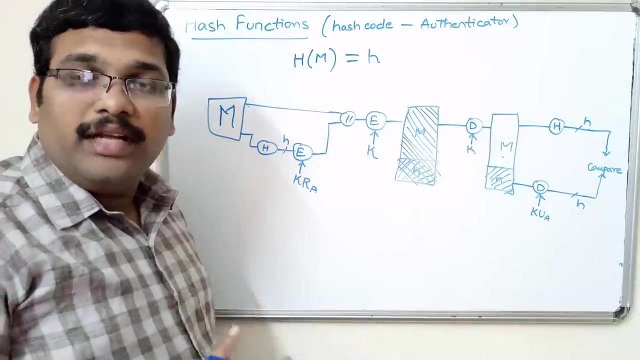 hash code which is to be compared with the appended hash code. if both the hash codes are equal, that implies the sender is other dedicated by the receiver. so that means the data is coming from the perfect sender, a valid sender, and also the data is not modified during. 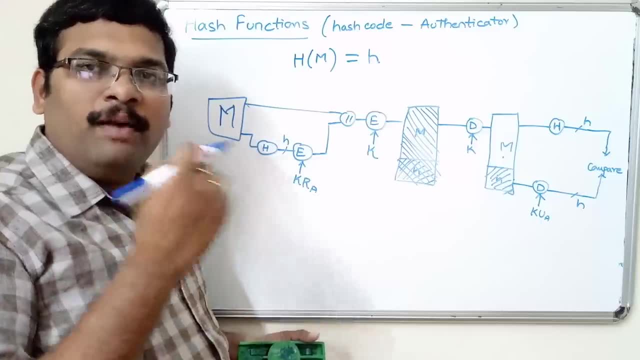 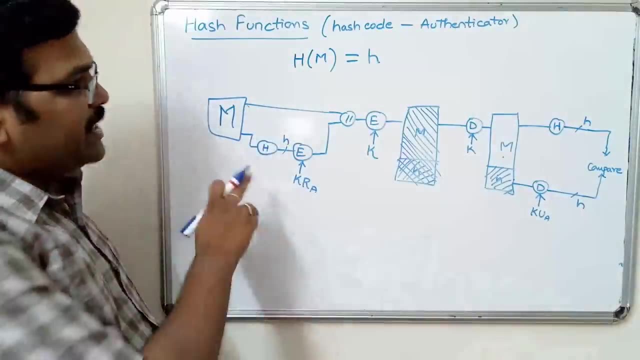 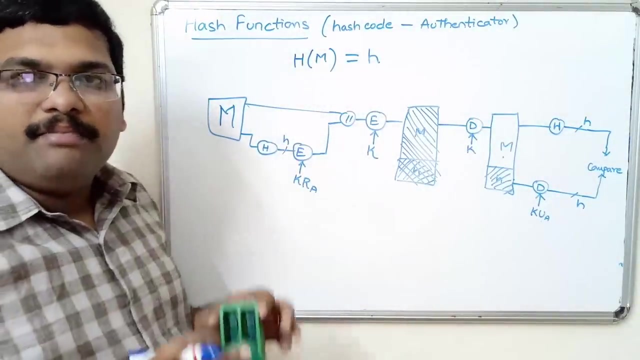 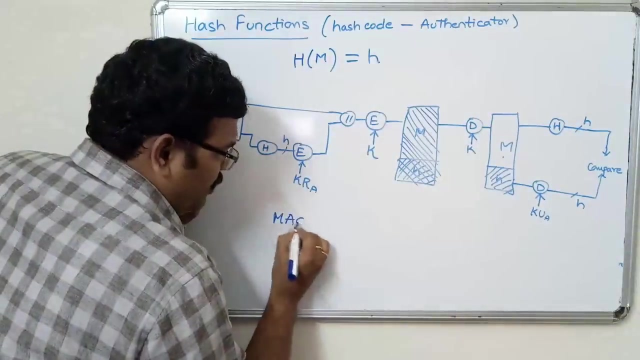 the transmission. so during the transmission if any one bit is changed automatically this hash code will be mismatched. so that's why we call it as authenticator. so here the hash code is an authenticator. in the Mac message authentication code is an authenticator. so both the Mac and hash code, Mac or 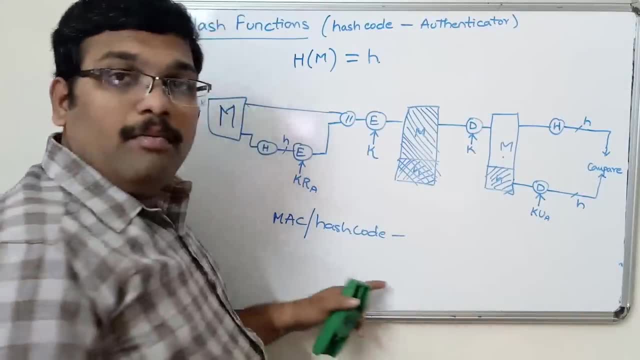 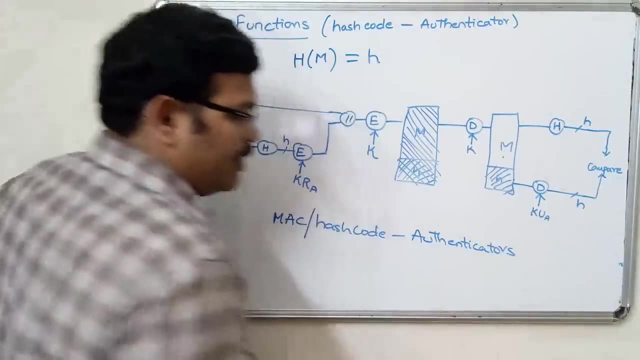 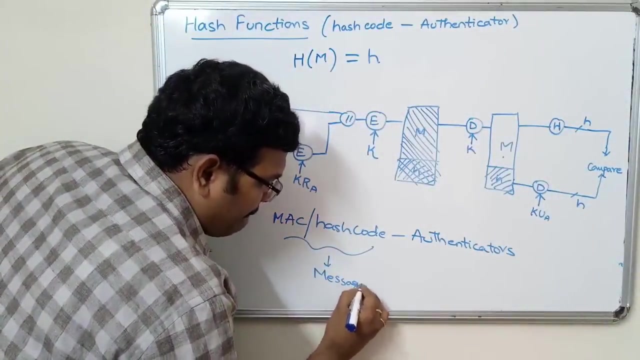 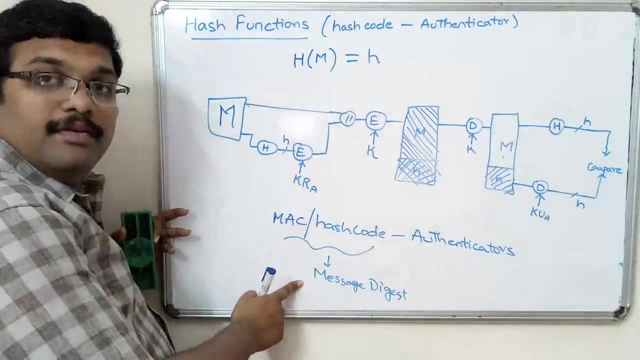 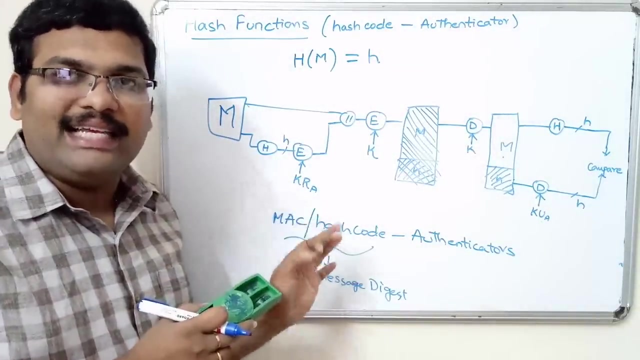 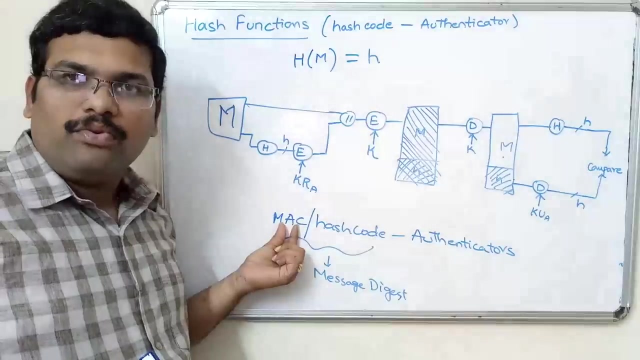 hash code, both are the authenticators, and this Mac and hash code, both are also called as message digester, message digester, right. so once again I'm repeating: these are not the encryption algorithm, this is the authentication, and there are different algorithms to generate this hash code and to generate this message authentication code. so 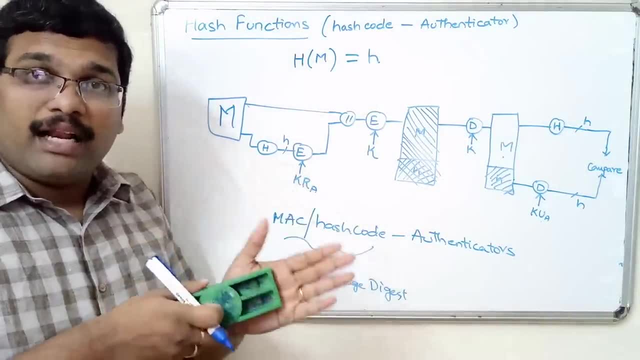 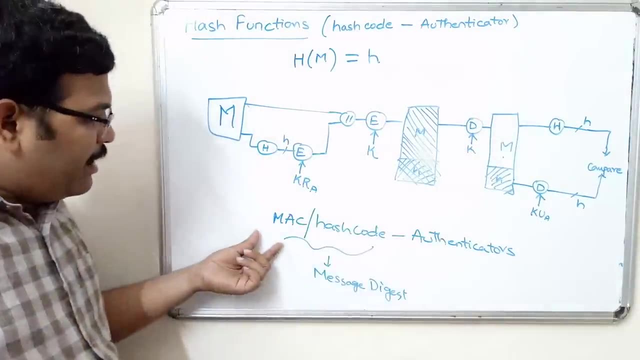 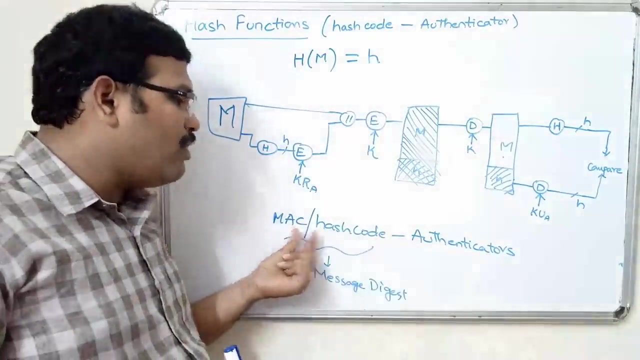 similar to the encryption algorithms. so encryption algorithm don't get confused. encryption algorithms means conversion of plain text message to ciphertext and and this authentication algorithms are to generate this authenticator. that means either Mac or hash code. so in order to append with the plain text message and 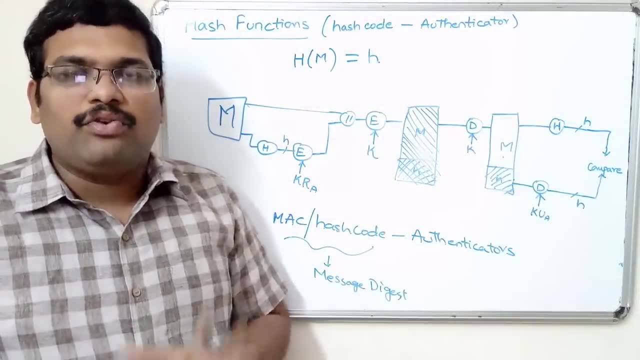 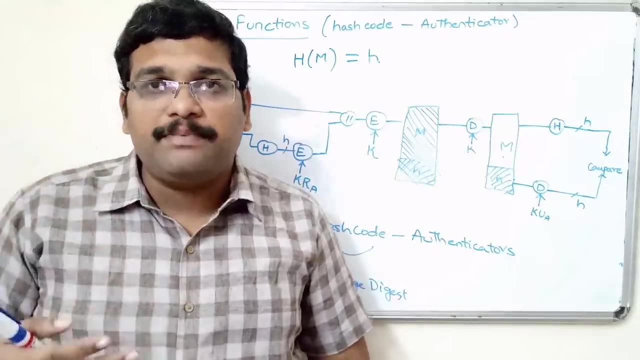 send to the receiver. so hope you understood. so there are once again. I'm repeating: there are three types of authentications. so one is message encryption, where the ciphertext will access an authenticator, and the second one is message authentication code, where a fixed length code is used to send an. 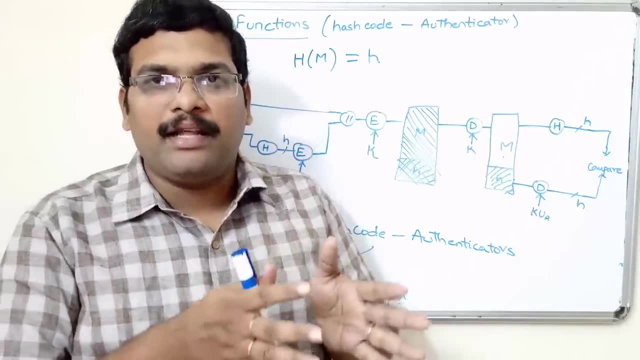 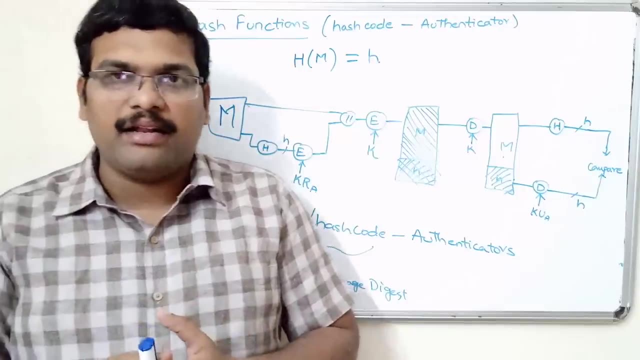 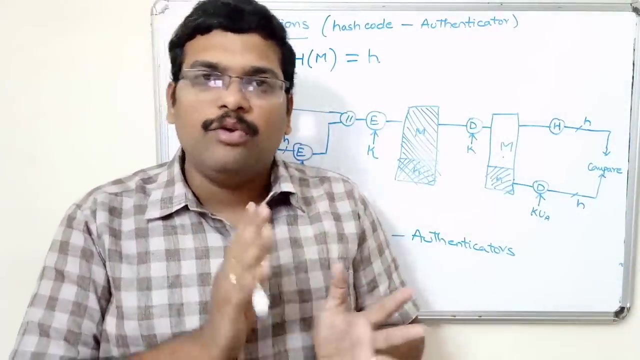 length code should be produced by applying the message authentication functions, along with the key, on the plain text message, and that message authentication code will act as an authenticator. and coming to the third one, hash functions, here we have to apply the hash functions on the plain text message, which again produces the fixed length code, which is called as hash code. here 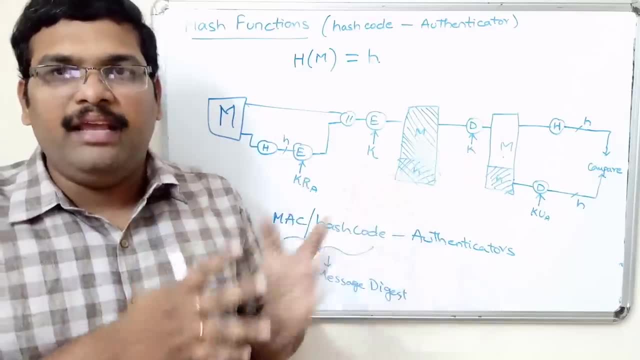 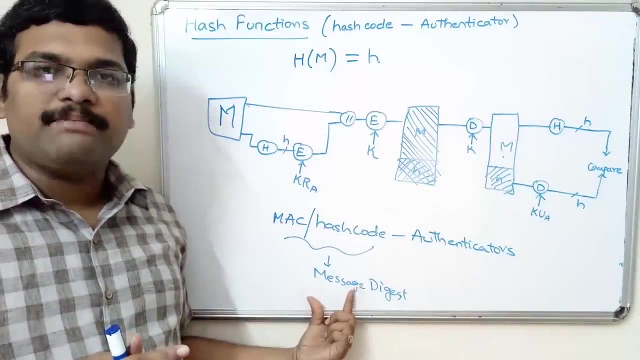 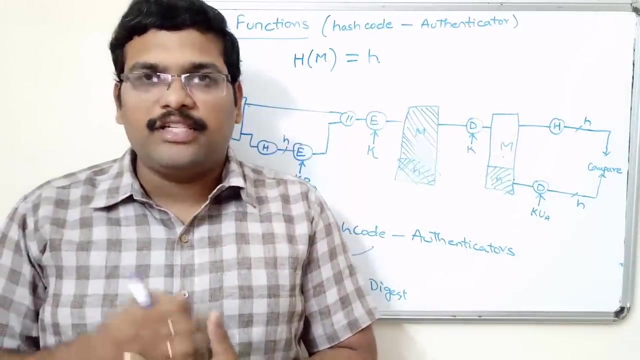 independent of key. we will not use any key on the plain text message. so this hash code or mac, both are called as message digest, so this will act as an authenticator. so let us stop here. in the next session let us have a look on these authentication algorithms. 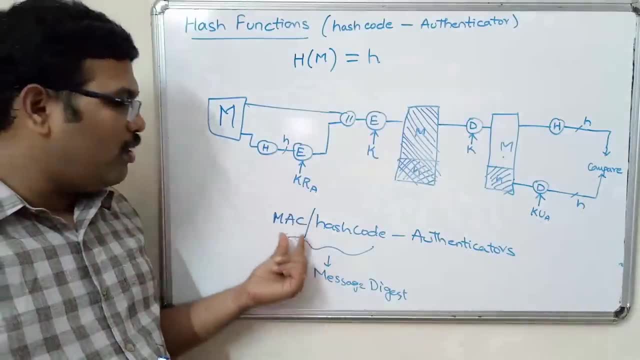 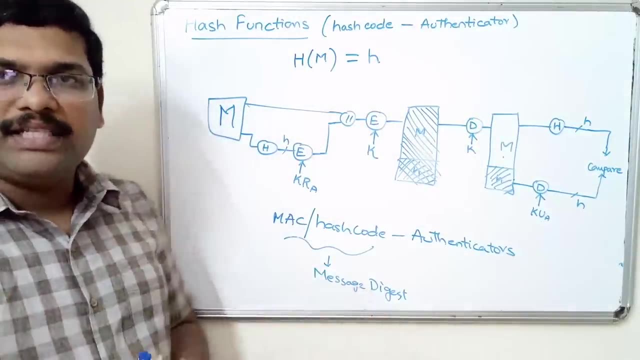 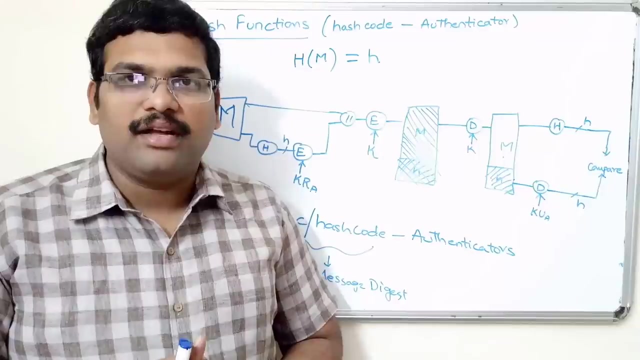 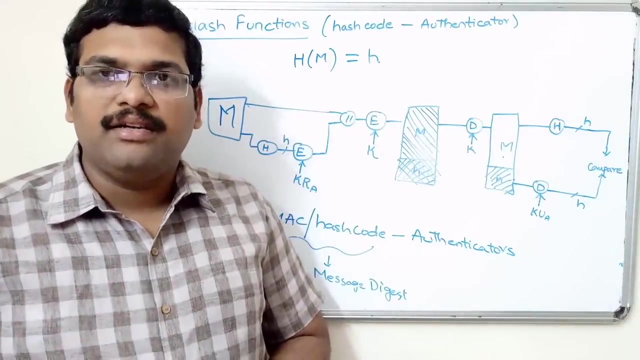 so algorithm which will produce this hash code or message authentication code. so simply we can say it as message digest. so in the next session we will discuss about this authentication algorithms. hope you understood. so if you are having any doubts regarding this message authentication, feel free to post your doubts in the comment section.